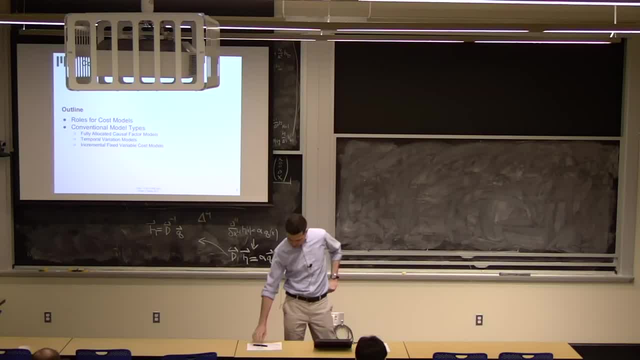 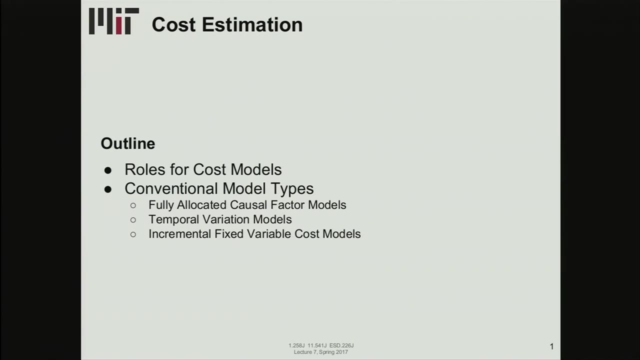 So today we'll talk about cost estimation. It's the first of the modeling lectures. We'll talk very briefly about the role that the different roles that cost models have in transit agencies And then we'll discuss three types of, three categories of cost models. All right, 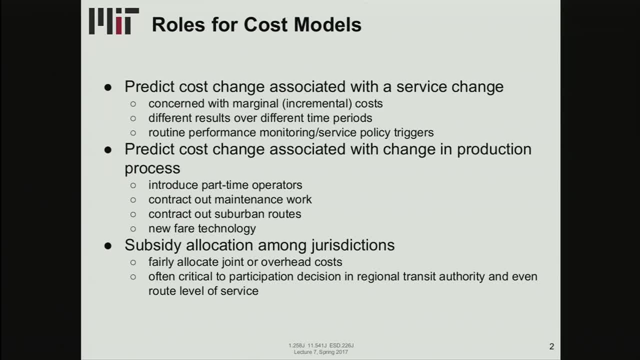 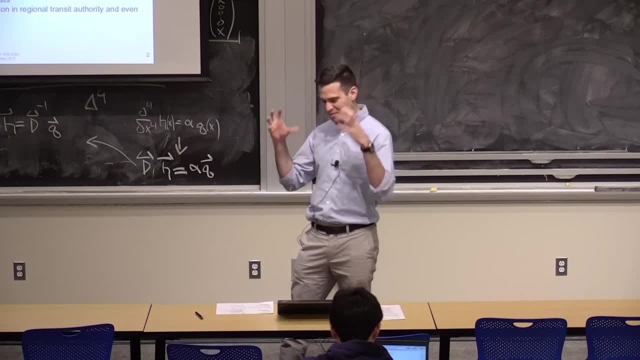 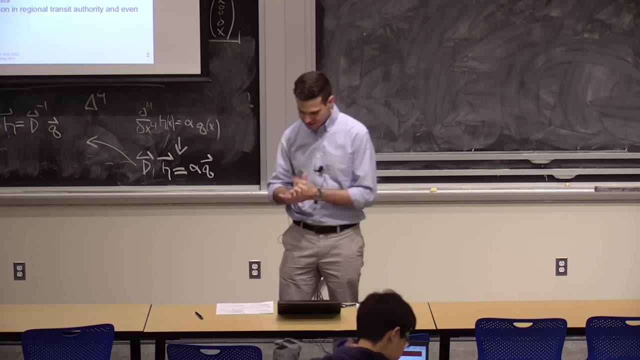 let's get right into it. So what are the roles? Why do we? how could cost models be used? And to start a cost model, right is a model, a mathematical model that takes some variables and predicts some cost for the agency. It could be operational cost, it could be fixed cost. 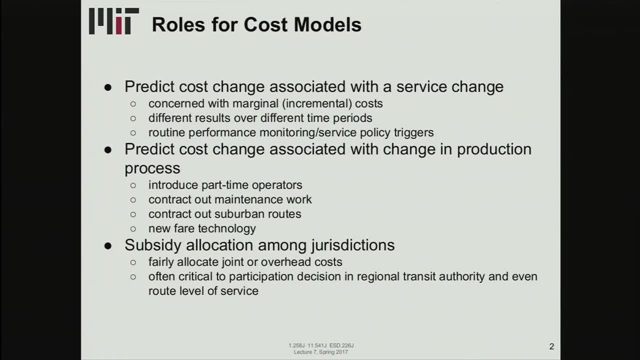 So how could these be used? The first role is predicting the cost change associated with the service change, right? So this is a very traditional, a typical example. So you might extend the route as we are thinking about in this assignment, route 70 and 70A extending it. 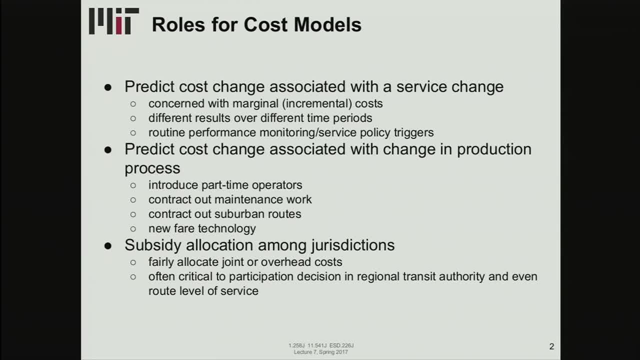 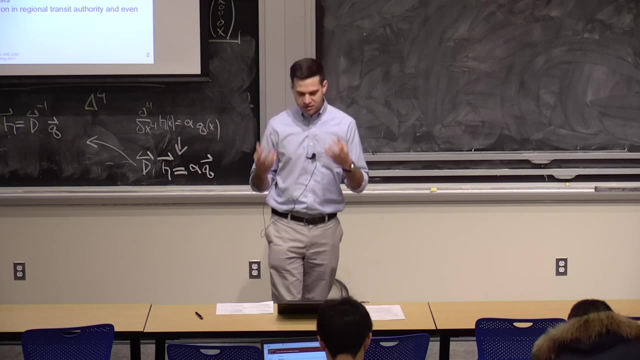 And you might wonder how much will that cost to operate right, So you could use a cost model in that situation. Or maybe there's a wider increase in service, maybe service is being expanded from ending at 2am to running 24 hours. How much would that cost? So these are the kinds of questions 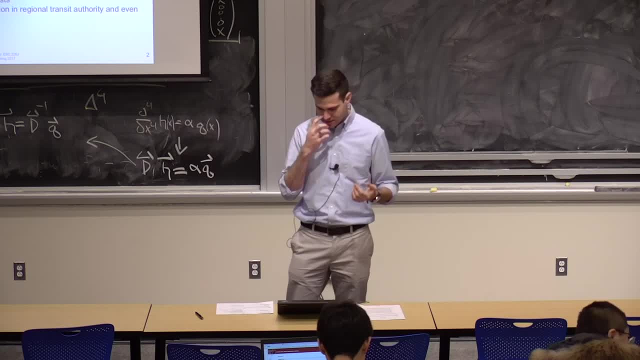 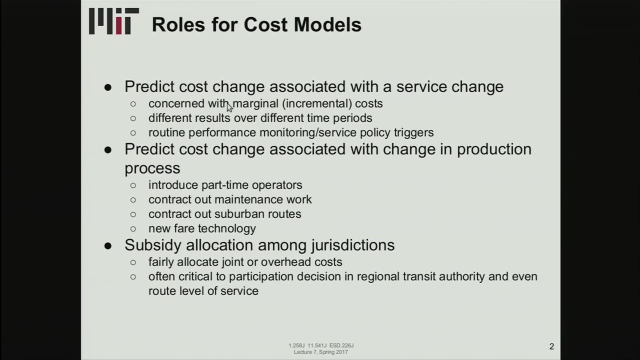 service changes that you might want to have an idea. how much will it cost mean? So they are often concerned with marginal or incremental costs. So we can talk about the responses here. incremental costs, especially in this application. So if you expand service to cover all night, for example, 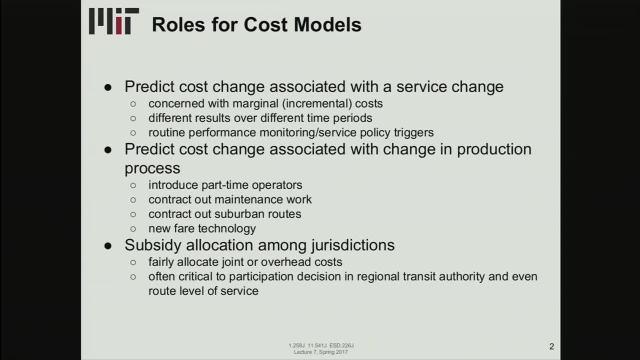 you may not need that. That change may not trigger the need for a new bus maintenance facility or some large capital expenditure. So we're talking here about incremental cost. As I add buses or as I add bus hours or as I add driver hours, how much extra do I pay? 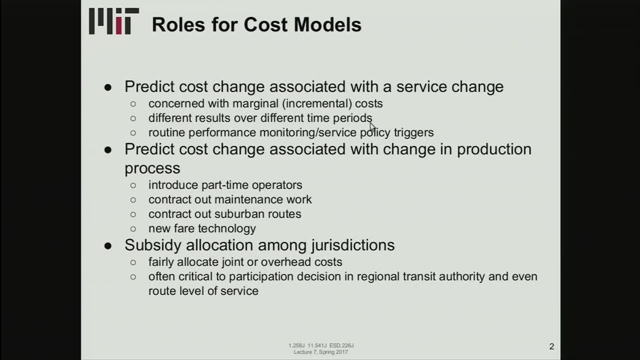 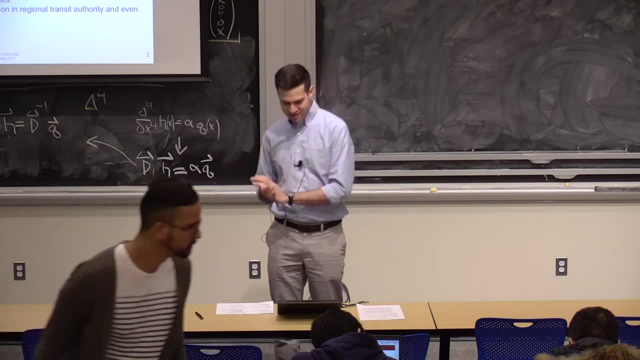 You have different results over different time periods. This is important. It doesn't cost the same to run service off-peak or at night as it does on the peak. I'll talk more about that later in this lecture. But having that in mind and having a cost model that 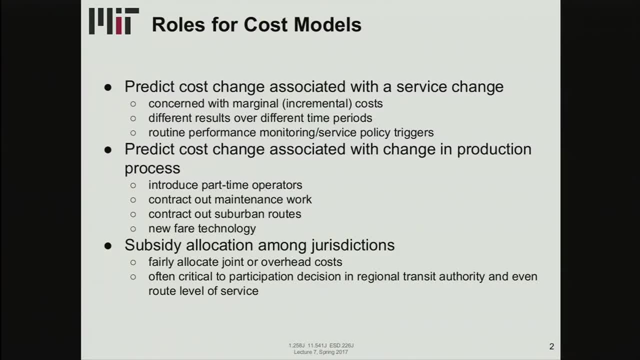 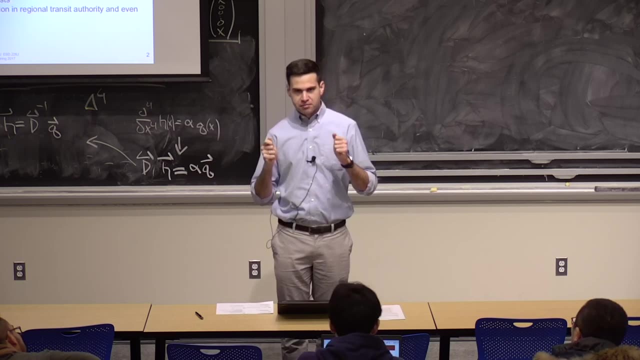 is sensitive to time periods, might be very important to get accurate estimates. OK, so these models can also be used for routine performance monitoring and service policy triggers. You might remember from the short-term planning lectures that there are some processes where every bus route might be reviewed. 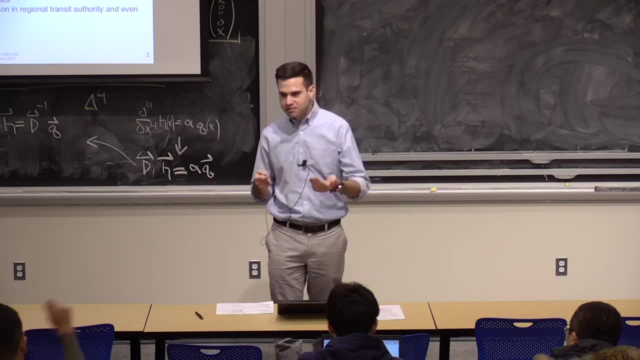 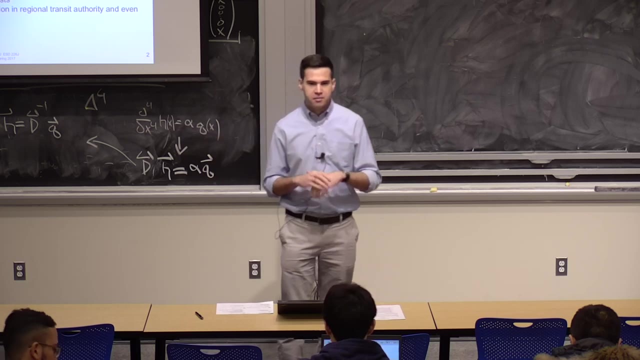 And you might decide that you need to add service based on its performance. Or you might decide that a bus route isn't meeting the requirements to be financially sustainable, So you are considering removing dropping service on that bus route. How much will you save by doing that? 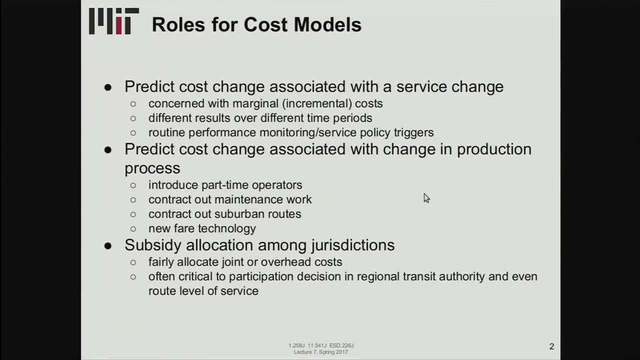 All of those are applications of custom models. OK, The second point here is That you can predict the cost change associated with the change in a production process. Now we're not talking so much about service, But we're thinking of what happens. 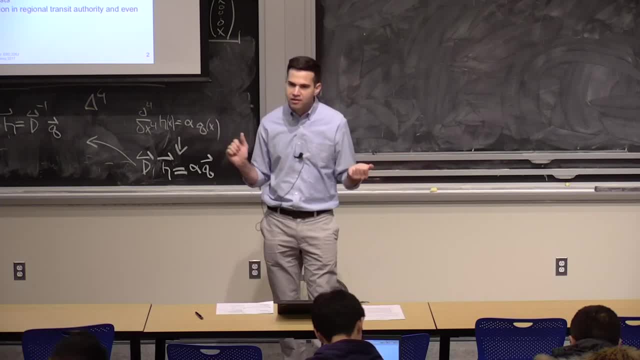 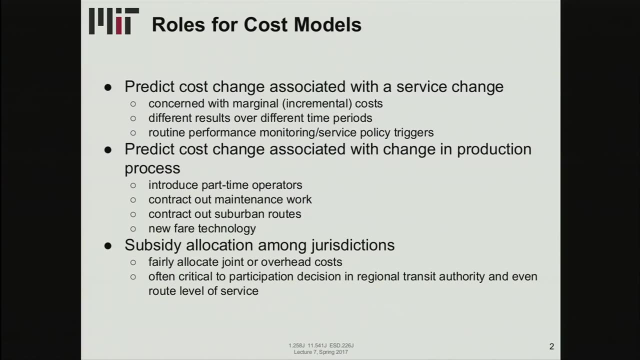 if I'm in a labor agreement that does not allow part-timers and now I've negotiated the ability to hire part-timers, What will that do to cost to the cost structure? What about if I want to contract out maintenance work? I'm doing that right now in-house and now maybe for a portion. or for all of it. We are looking at public-private partnerships to contract out maintenance work Or contracting out suburban bus routes, Routes that have low ridership and they're kind of on the outskirts. You don't want to drop service, but maybe you. 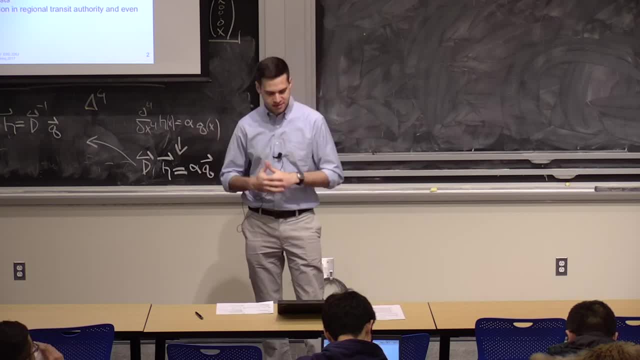 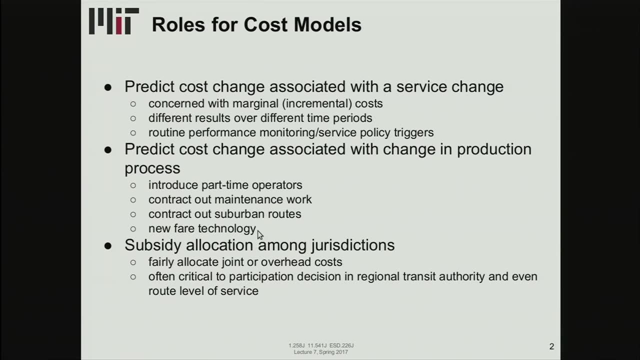 don't need big 40-foot buses And you can run them with smaller buses. Could you contract those out? What will that do to cost? New fare technology, The BTA? I don't know who was here a long time ago. 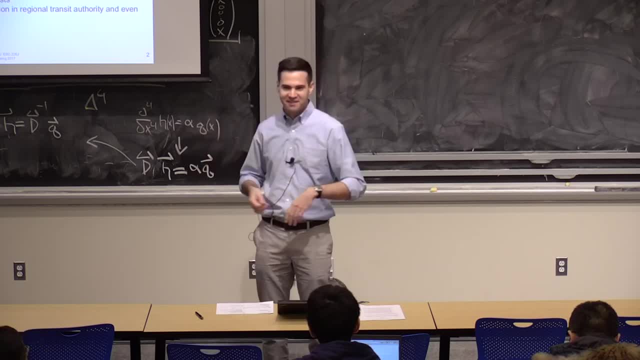 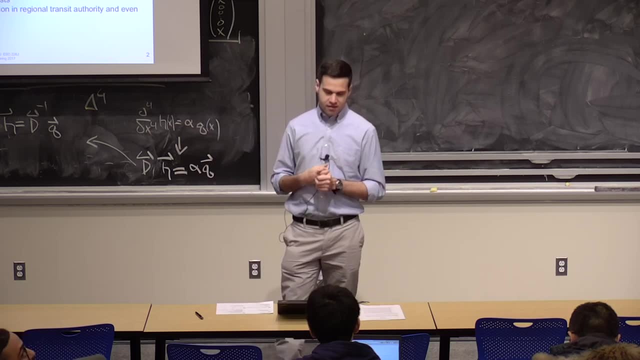 but we had tokens here And we moved to the Charlie card, And now the MBT is thinking about the next generation of fare collection for Boston. So when was the Charlie card introduced? I don't remember the year, but it was the mid-2000s. Because I remember in 2004, there being tokens still, I think the last station was token government center in 2006.. So any time something like this happens, there is a change in costs And administration costs And the recovery, the fare recovery ratio, might change. 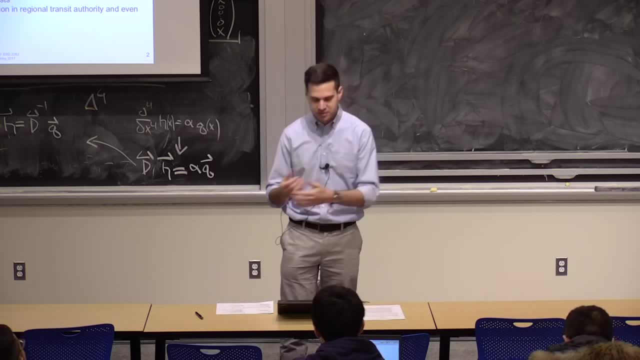 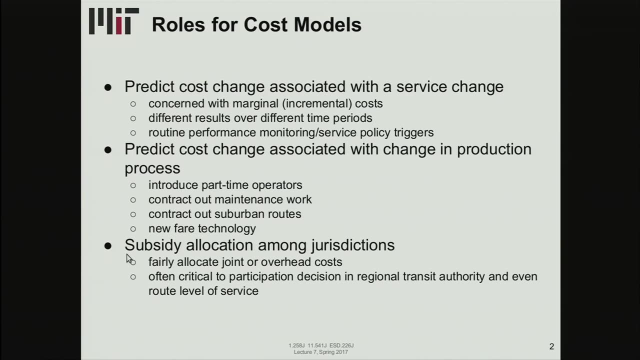 So can we model that And can we use cost models to predict those changes in cost or in revenue? Then another third and very important allocation, not so much in Boston right now but certainly in other jurisdictions, is the allocation of subsidy required by jurisdiction. So if you look at, for example, the one in WMATA in Washington DC, there are different districts And they all have to pay for service. So there are many examples of this over the state and also internationally, where different jurisdictions are. 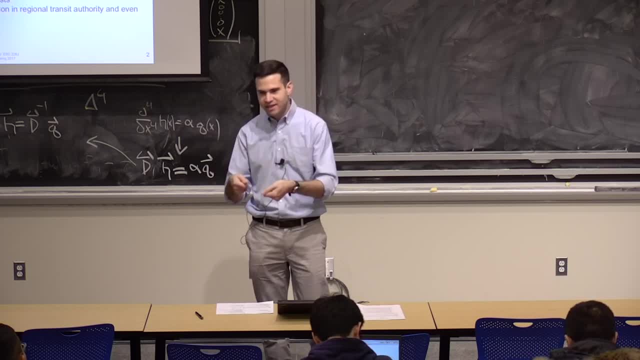 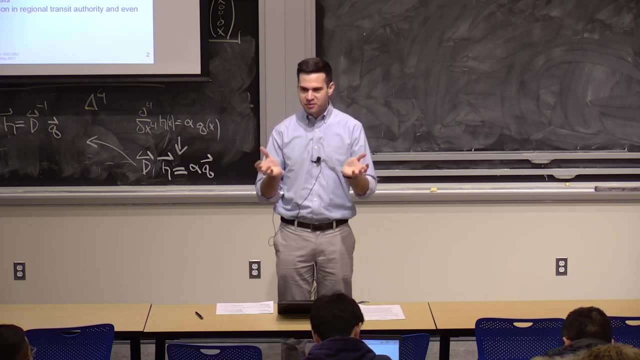 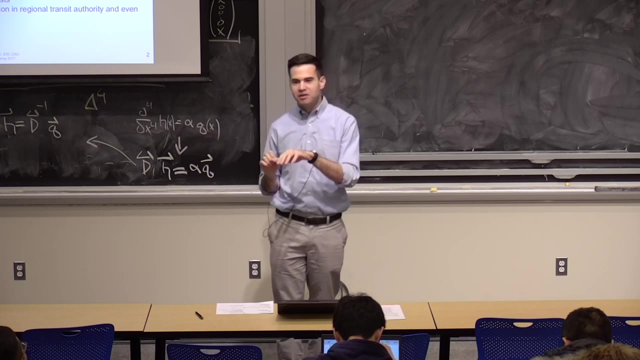 essentially partnering to subsidize public transportation service, And we know what the total cost of operation is. So how much is fair? How much is fair that each jurisdiction pay according to size, according to how many people- Often it's according to how many people ride? 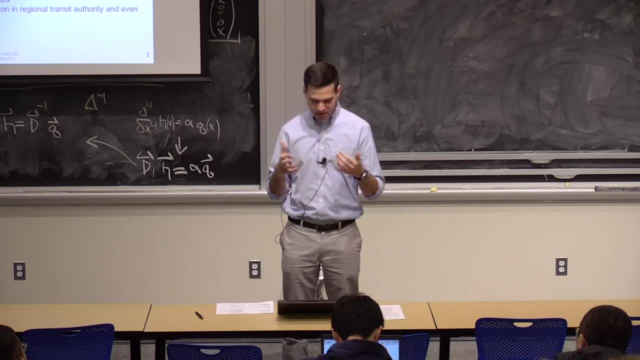 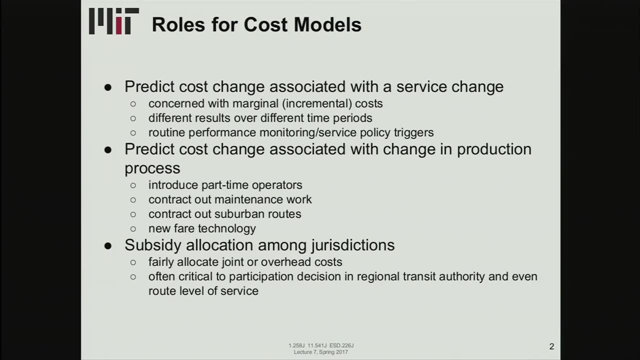 from those jurisdictions. So you might have a data collection to figure out how many people are taking buses from each of the jurisdictions. And then you need to allocate a cost allocation model to take all of the costs, including the things that are sort of more obvious, like the bus hours that operate on. 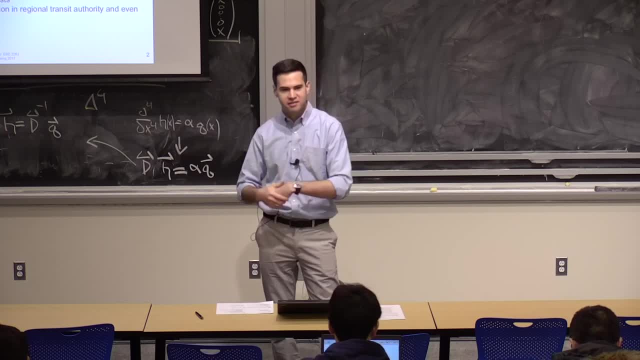 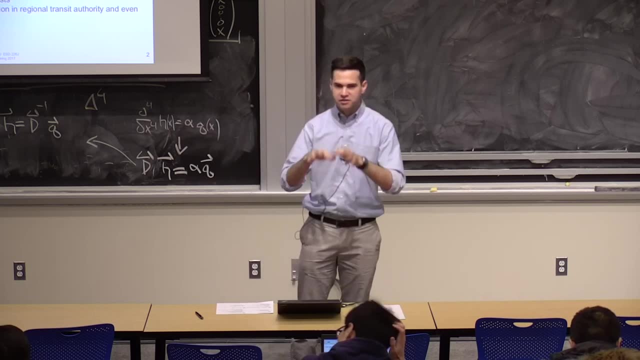 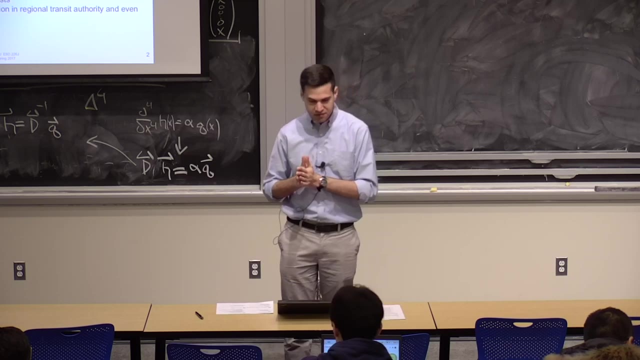 in those jurisdictions, but also things that are not directly connected to that jurisdiction, such as administration costs and facility maintenance and those things. So all of that needs to be allocated to each jurisdiction so that the costs can be evenly or fairly split, And doing that right is critical. 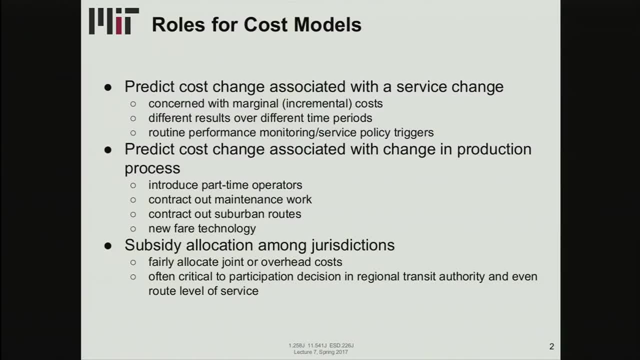 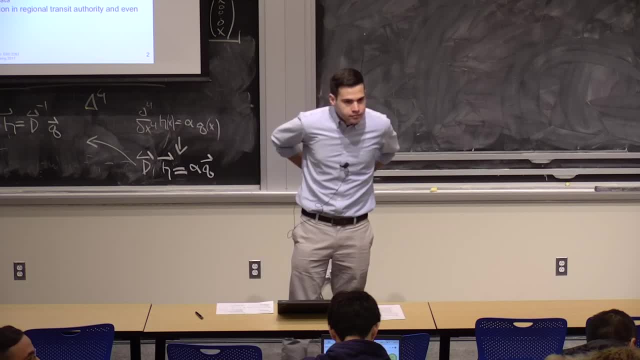 often even for the decision to participate or not in this program. Question For jurisdictions: you mentioned Washington. Would that be like Virginia and Washington DC, Yeah. Or in New York, it would be New York, the Port Authority of New York and New Jersey. Or do you also mean like counties? There are many examples of different structures, of how different jurisdictions come together to provide service. So in some cases you have many different operators. more commonly, in the west of the US, many different operators all providing service somehow. 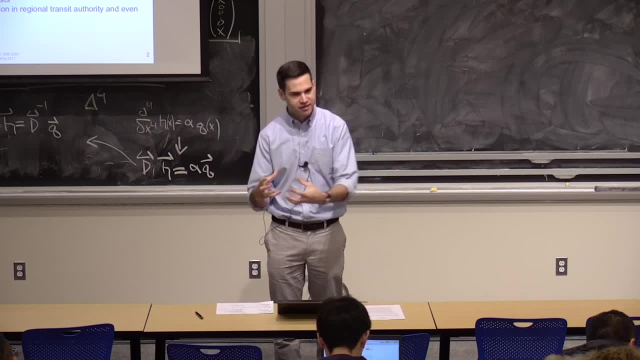 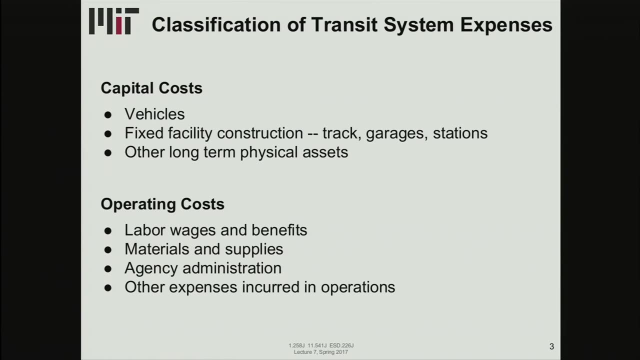 In other cases you have one major operator funded by different jurisdictions. So all right. So you might remember, when we talked about modal capacities and costs, that especially in the US, in North America, costs are divided into capital expenditures and operations expenditures. 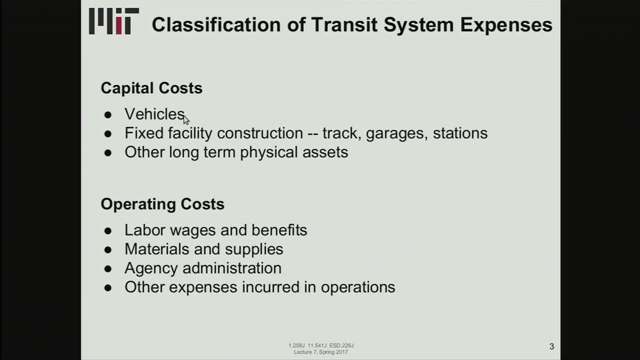 So capital costs have to do with the purchase of vehicles or the mid-life re-hauls of vehicles, heavy maintenance, the fixed facility construction, So construction or major repairs of trucks, garage stations, bus stops, things like that, And then other long-term physical assets. 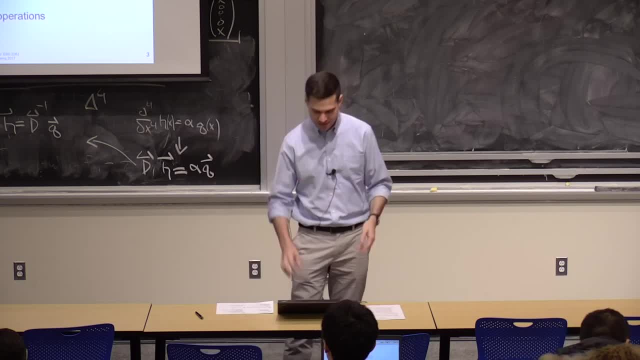 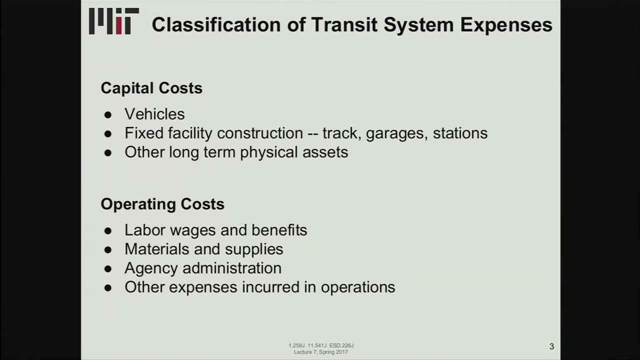 So administration, building things like that. And then there's operating costs, So those have to do with they're more proportional to how much service you output. So labor wages and benefits, materials and supplies. Materials includes fuel and tires and electricity. 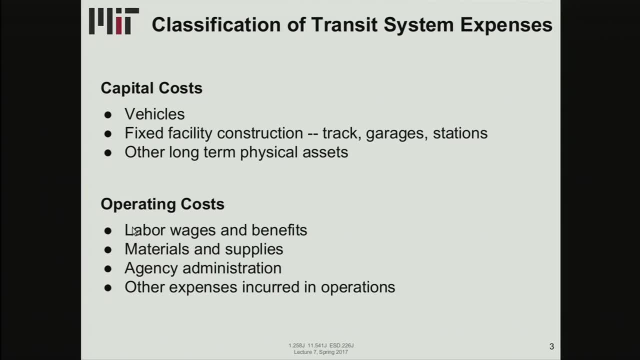 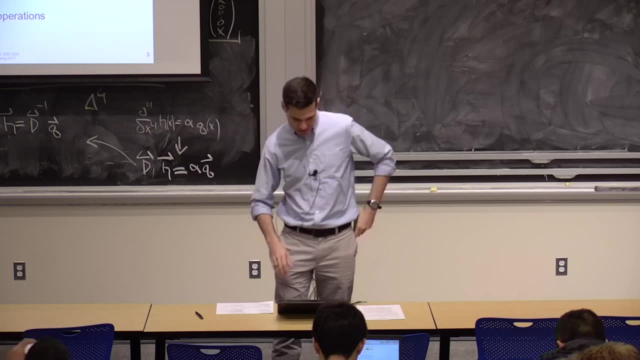 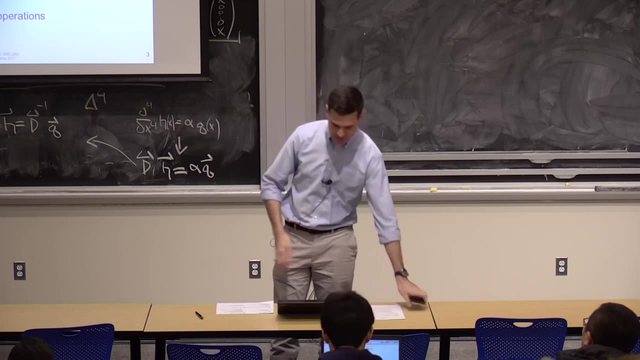 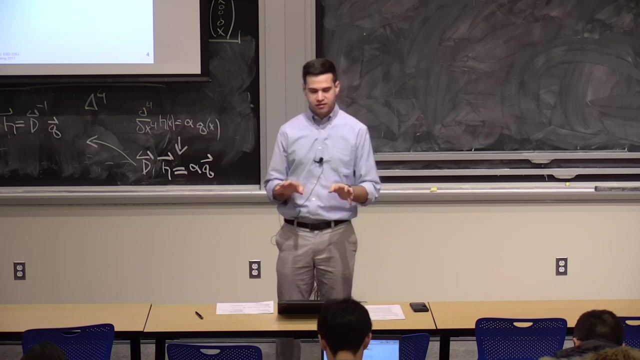 So to run the power metro. Then there's agency administration and other kinds of expenses of this nature. So it's important to keep those two in mind, because the cost models that we specify should take this into consideration and be able to allocate the capital and operating expenses. 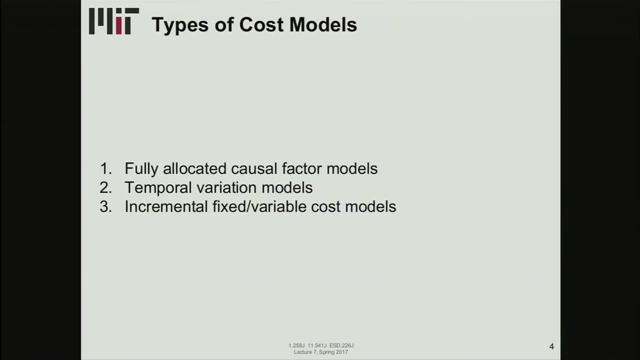 separately. All right, So there are three types Of cost models that we're going to discuss. First is the fully allocated capital factor model. It's the simplest of the ones we'll discuss. One of the problems with that model is that it allocates all the costs to some categories. 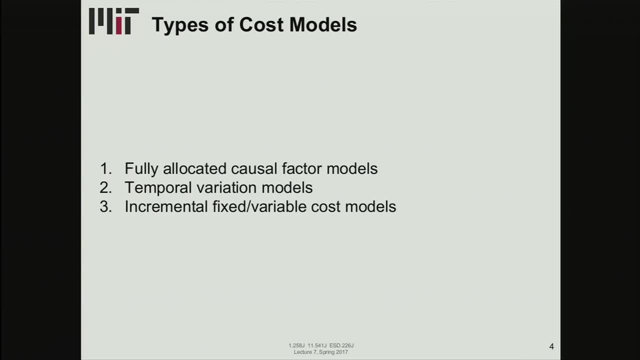 And it's not sensitive to time periods. As I said earlier, some costs vary a lot by time period. So the second model essentially is a variation or an extension of the first one, where we do take some specific costs that are very sensitive to time and capture. 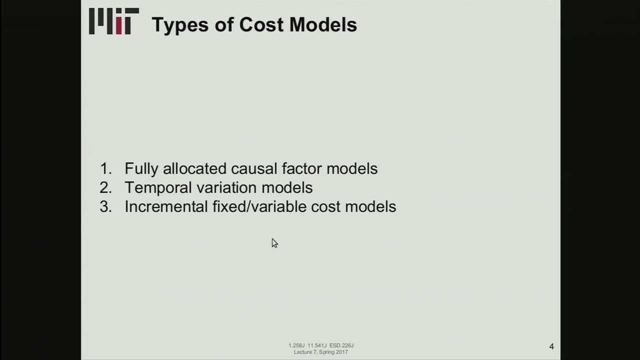 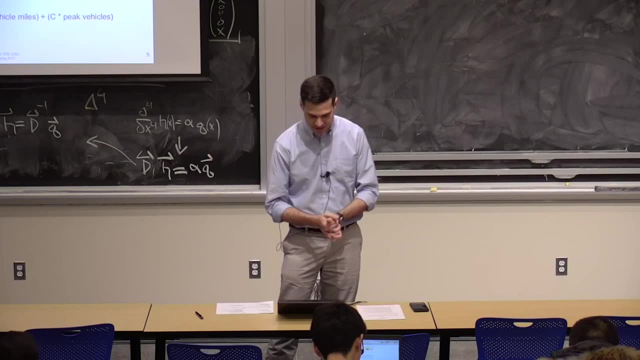 those differences over time, And then we'll talk about incremental, fixed, variable cost models. We're going to give examples of all of these, using MBTA bus from the 90s as an example. Let's start with the first one, the fully allocated capital. 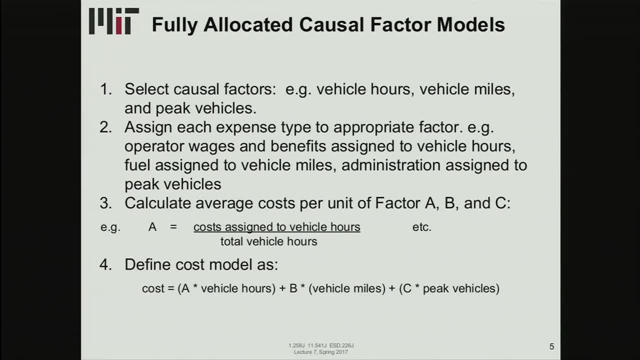 factor model. So here's what you do: You select some capital factors, So these are not necessarily. maybe capital factor is not the best term, but that's what this model is, This class is called. I would say these are explanatory variables more. 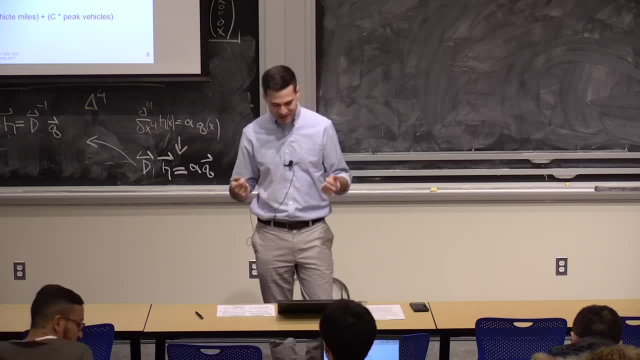 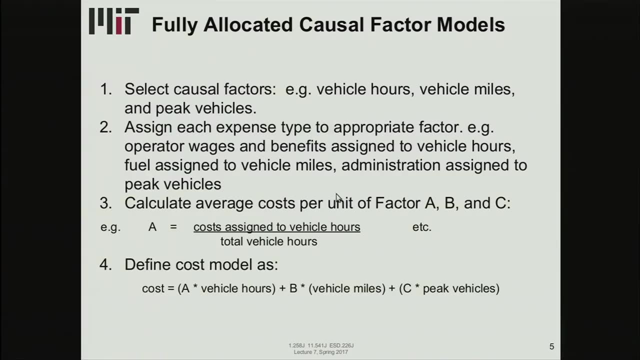 than capital factors. They don't have to cause the cost directly, but they are used as explanatory variables on a model of cost. So then you assign each expense type to each of the factors, So for example, operator wages and benefits. where would that go? 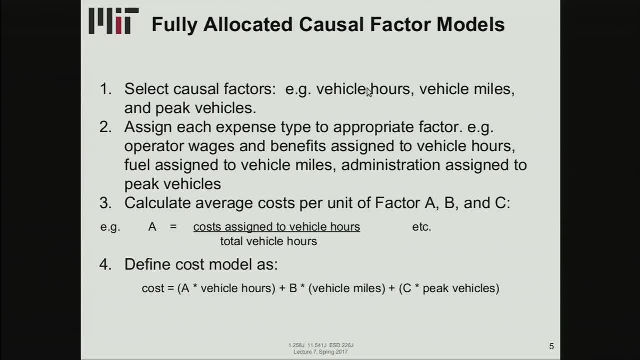 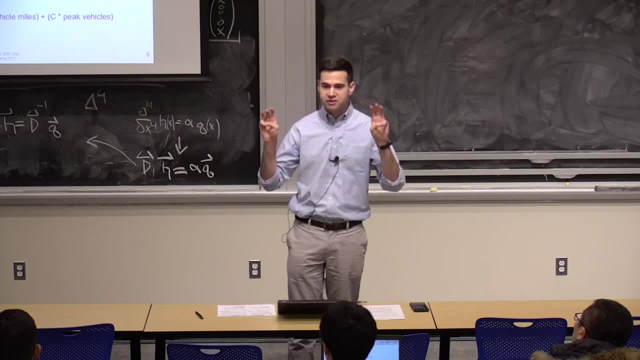 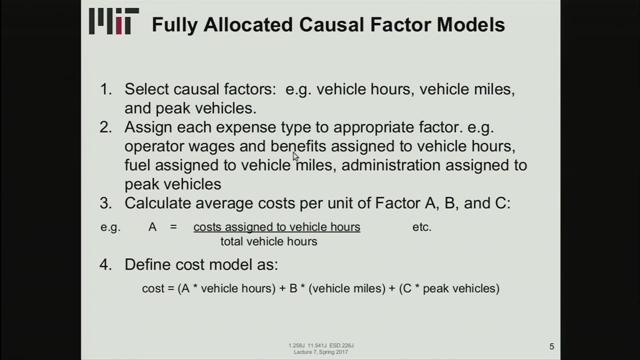 If you were thinking of three kinds of explanatory variables, vehicle hours being one, vehicle miles being the second and peak vehicles being the third. you're going to assign every cost you incur to one of those three. Then operator wages and benefits are more appropriately assigned. 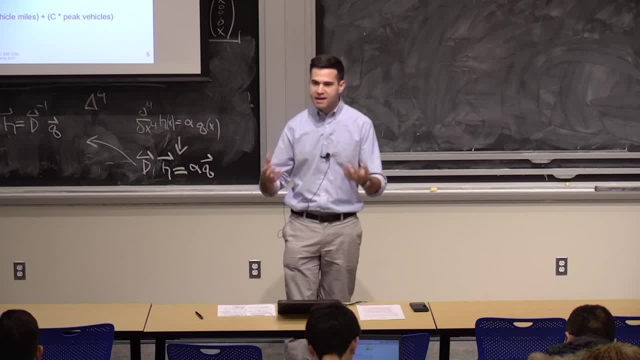 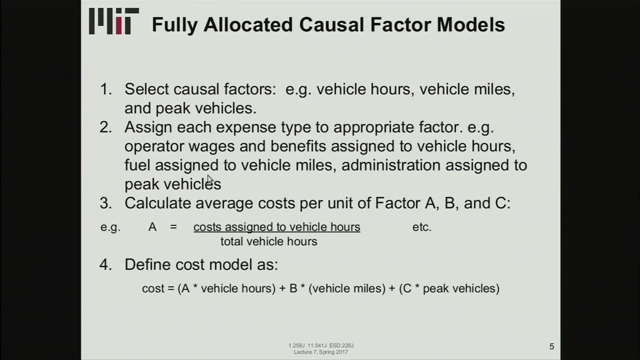 to vehicle hours, because you pay drivers by the hour, So this is the one that it relates to most closely. Fuel, so fuel, maybe a combination of vehicle hours and vehicle miles, or if you have to assign them to one, then vehicle miles. 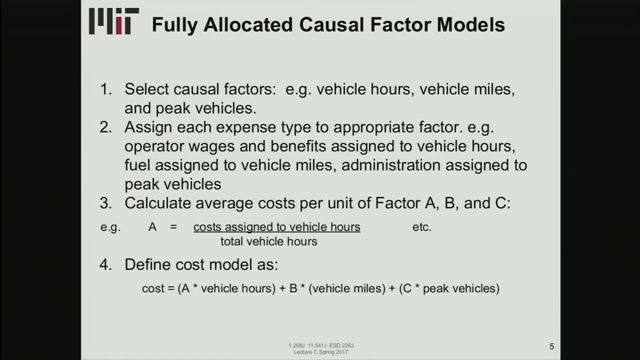 You think of the fuel mileage of vehicles, Right? So that's the one that most closely relates vehicle miles to fuel. And then administration. well, administration, you might want to assign it to peak vehicles, because peak vehicles is a proxy, for how big is this agency? 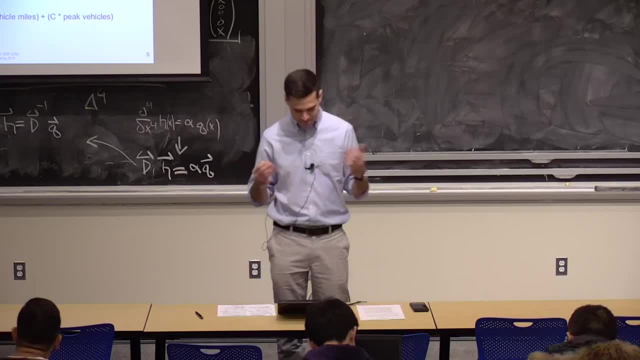 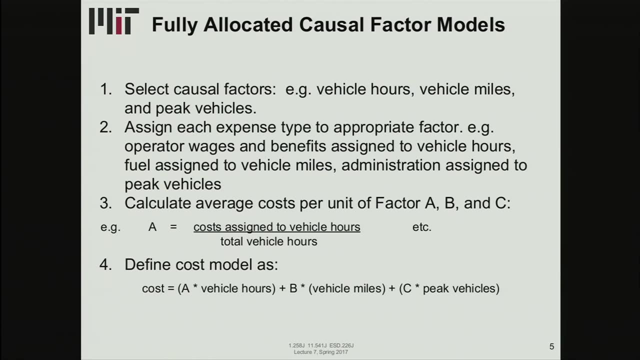 And the bigger the agency, the bigger the administration costs, right? So it's one way of assigning these things. So this is an example. right After you do all those assignments, you calculate the average costs. So for each of the factors, 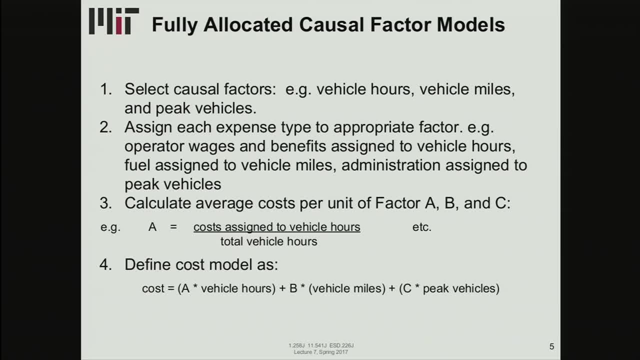 So you have, for example, the cost assigned to vehicle hours divided by the total number of vehicle hours and you have those unit costs. And then the cost model is simply each of those unit costs divided or multiplied by the three expiratory variables. that you included, right? So you multiply your unit vehicle hour cost by number of vehicle hours, your unit vehicle miles cost by vehicle miles and your unit peak vehicles cost by vehicles, And that is the total cost of the agency Questions. This assumes that you're somehow. 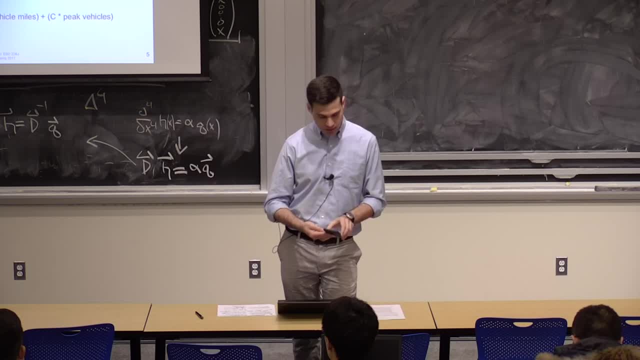 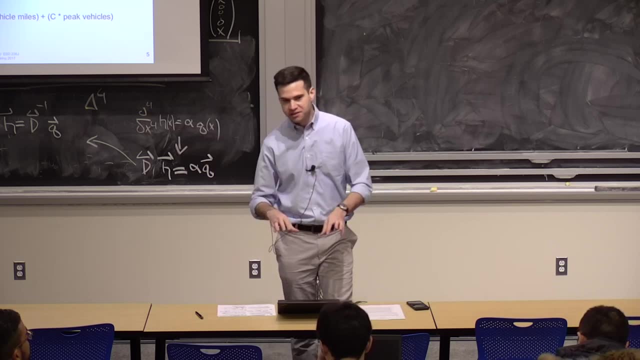 able to split the data into those categories. to say, the costs assigned to vehicle hours are x. Yes, So that's one of the characteristics and perhaps weaknesses of this kind of model: that it requires judgment of the person to assign first, to generate these classes and these expiratory variables. 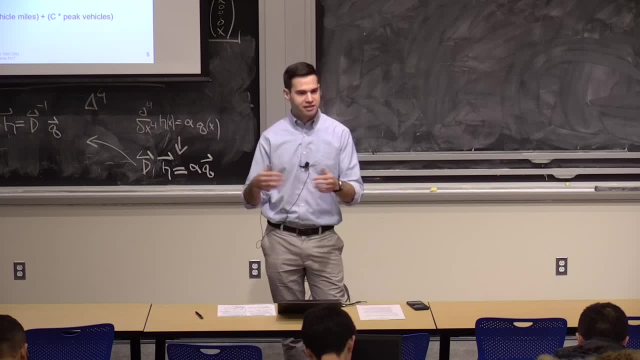 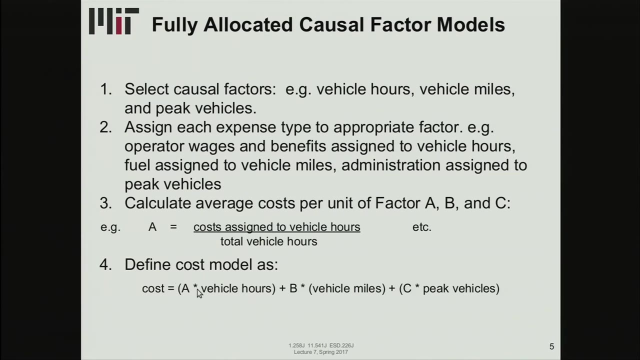 and second, to assign them to each class or each account in a letter Right To each of these expiratory variables. But these models are used in the industry. So if you plug in the number of vehicle hours and vehicle miles and peak vehicles that you used to estimate this model, 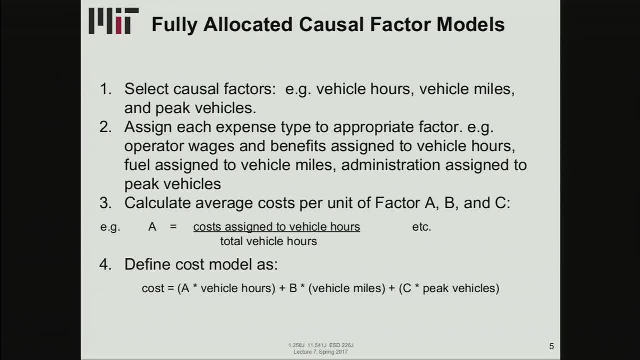 then you're just going to get the total cost of operations, or total combined cost, on the same period that this data came from. But, more interestingly, if you are considering expanding service and that will increase vehicle hours, vehicle miles and peak vehicles, then this model. 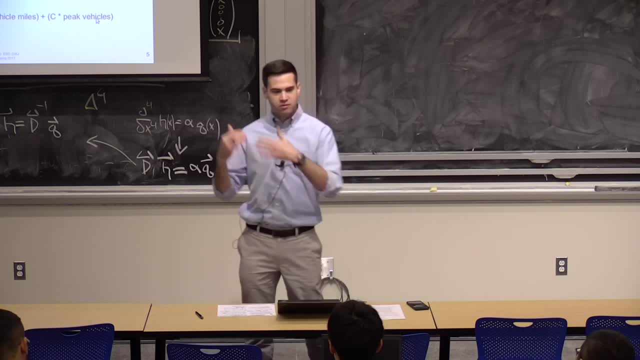 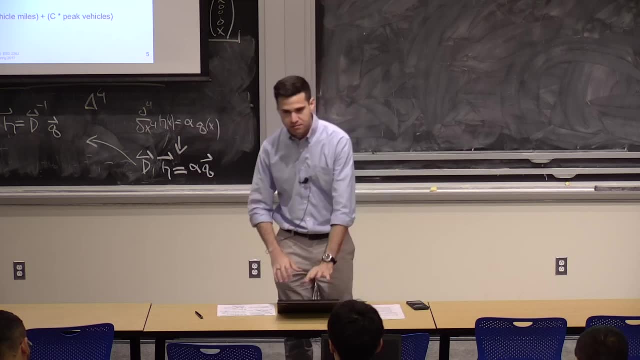 will work in some ways to forecast what the total cost will be after you grow your agency Right. So this is one application of this simple model. Is there a time unit that you're supposed to use, like a full year, to catch yourself? This is up to you as well. Another judgment call Shouldn't be one day, but because you want to see all the kinds of expenses. So I think a year makes sense, a fiscal year right, Because you'll have to put out a statement when you do accounting on a fiscal year basis. 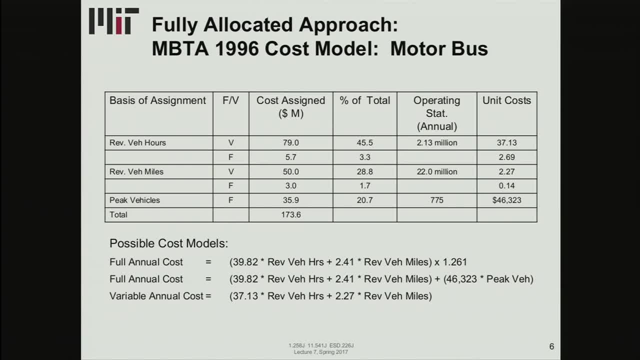 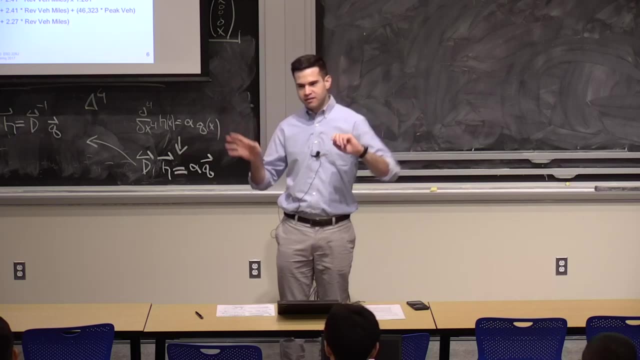 OK, so here's an example from 1996 of bus and the MBTA. So we have those three variables that we talked about: vehicle hours, vehicle miles And peak vehicles. We divide each of those into variable or fixed, So some of the expenses are considered variable. 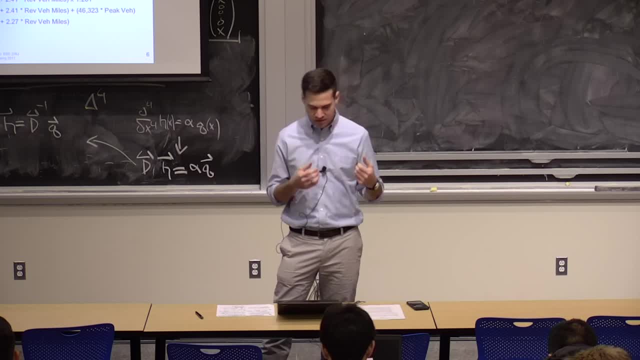 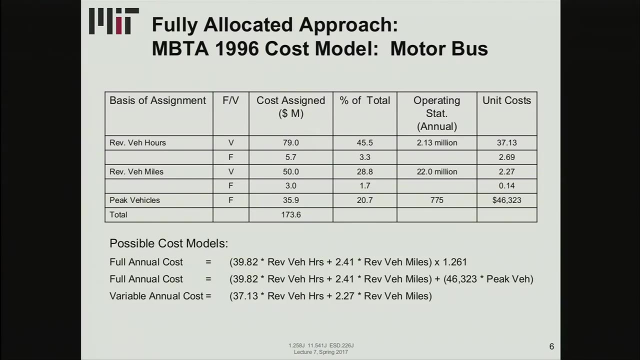 because they sort of scale up more linearly as you increase the number of vehicle hours And others are more fixed expenses. You wouldn't expect to get extra fixed costs by adding a few buses, right? So one example of that is if you get 10 more buses for a new. 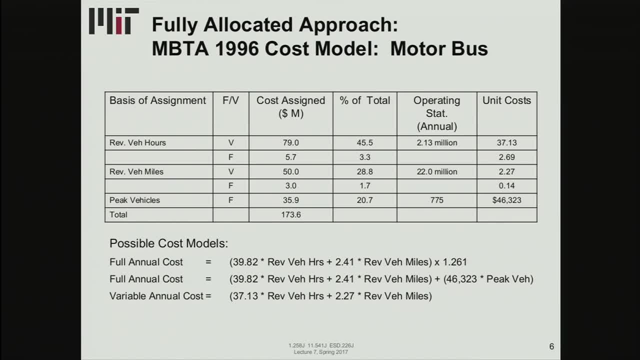 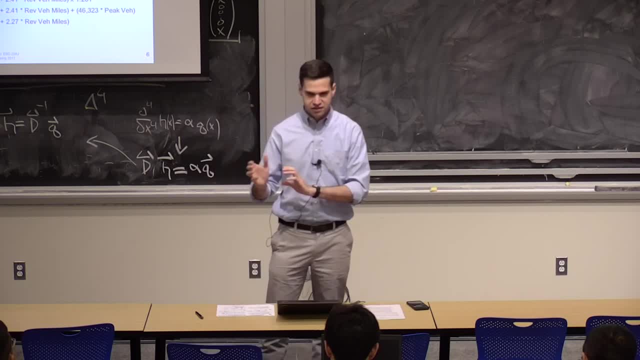 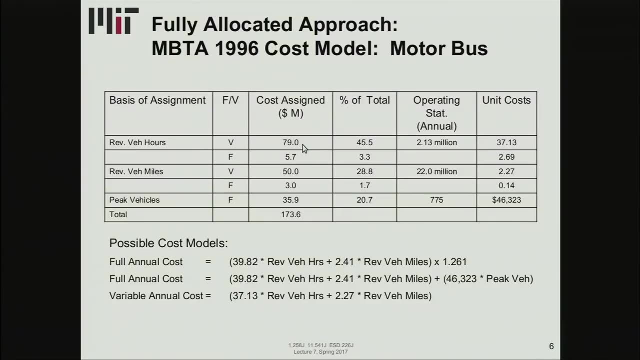 bus route, you don't need a new maintenance facility, right? So your maintenance facility might be considered a fixed expense And you might want a variable cost model to predict the changes of that small change or that marginal change. So that's why we divide things into fixed and variable. 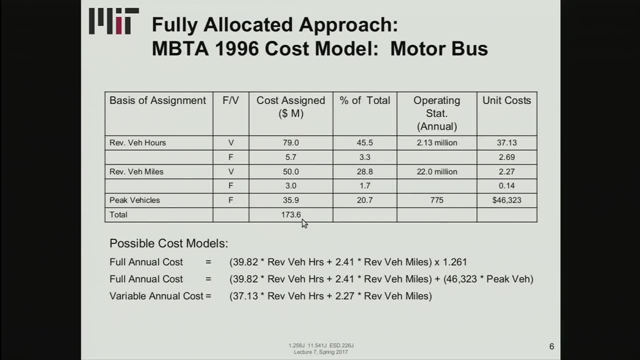 The total cost to be allocated is 173.6 million And we divide it over the six categories, the three variables, And they're fixed and variable variants. Here we have the percentages of each and the unit costs, right, So now, what are possible cost models following this approach? 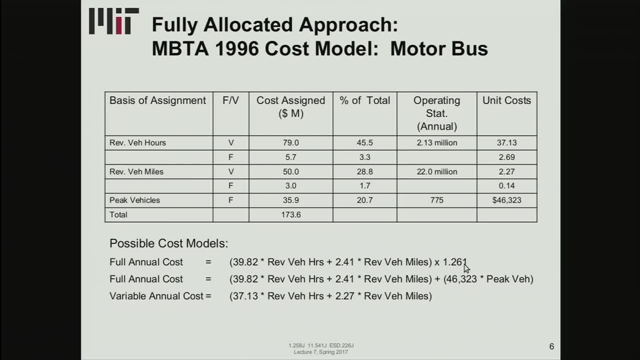 A first and simple one. a very traditional model is the first one listed here. So 39.82, which is the total unit cost of revenue vehicle hours, It's the sum of 37.32.. 13 and 2.69 times the number of revenue vehicle hours. 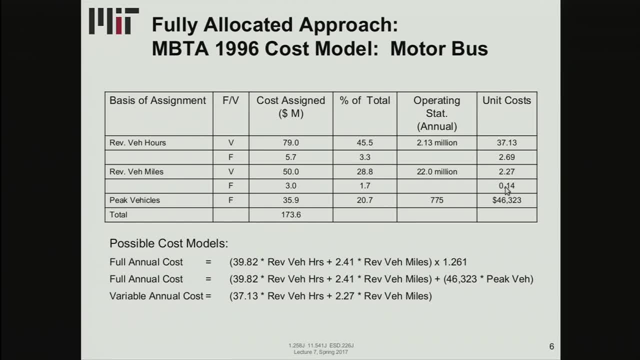 And then 2.41, which is the sum of 2.27 and 0.14 times revenue, vehicle miles, times some factor, And that factor essentially here we have. we're not capturing the difference between fixed and variable costs, right. 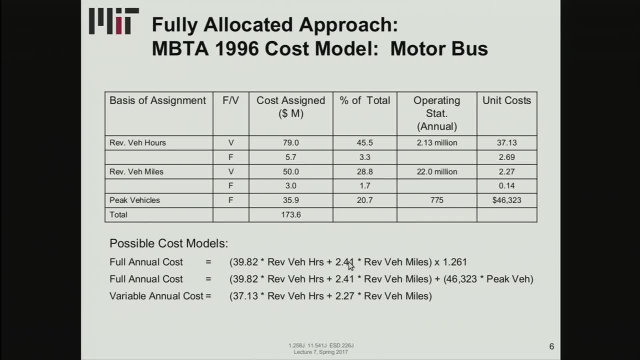 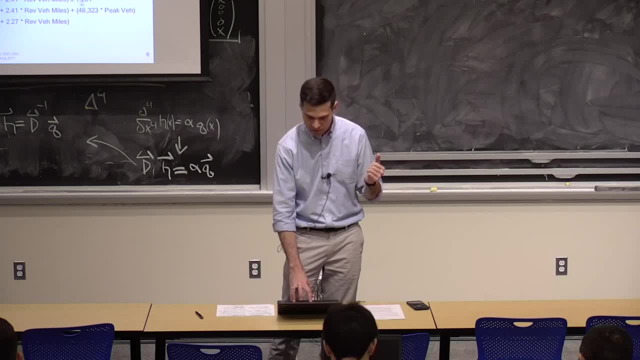 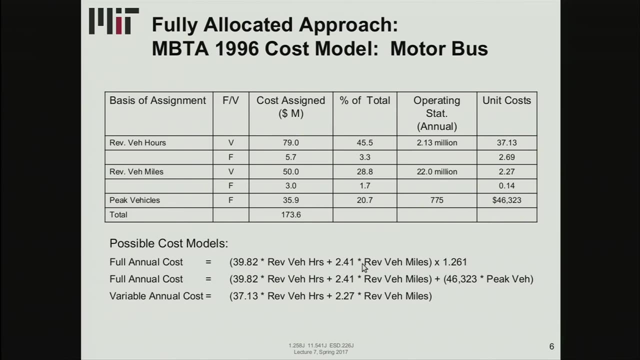 So that's why we add them up here: 39.82 and 2.41.. The other characteristic of this model is that it does not have peak vehicles as an explanatory variable right. So we address that with this adjustment factor. If you take the total cost, which is 173.6,. and you divide it by the sum of the unit costs for revenue vehicle hours and revenue vehicle miles, you get 1.26.. And that's the adjustment factor. Any questions with that approach? Sorry, so the 1.26 is calculated by doing what? 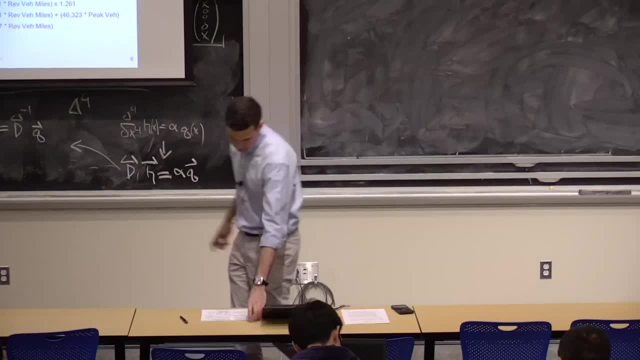 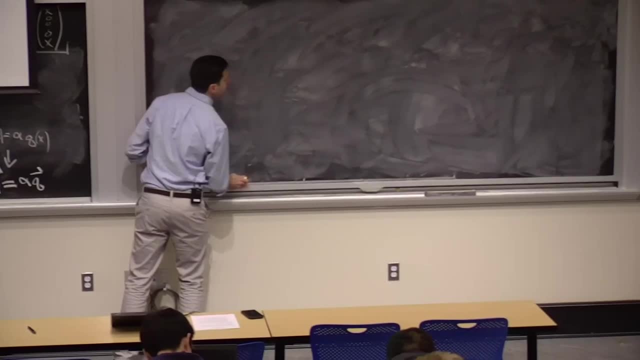 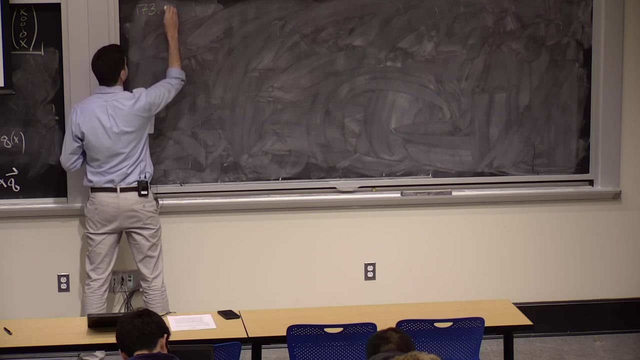 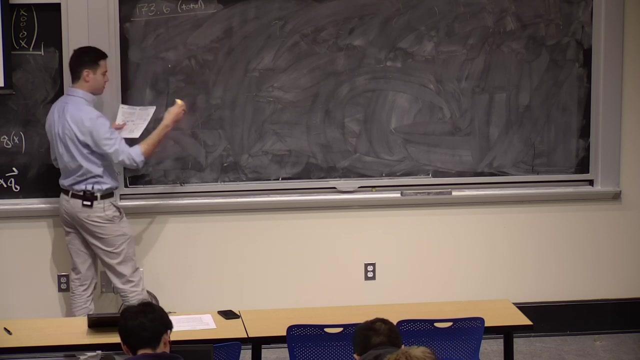 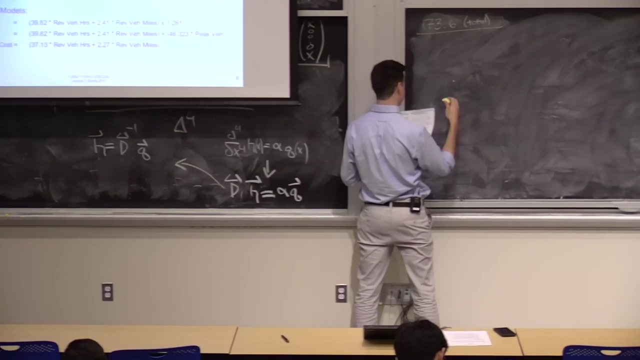 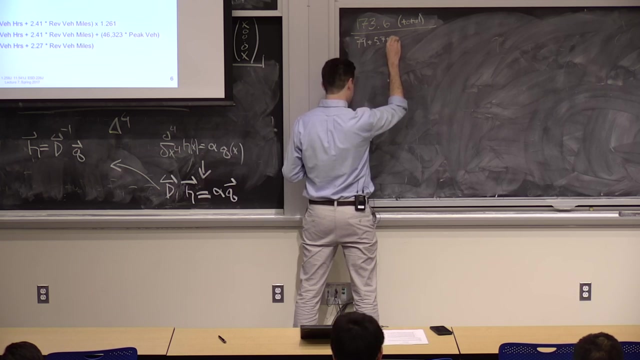 Let me write that down for you. So you have a total of 173.6, and that's the total, And you divide it by the total number of unit costs that you are capturing with explanatory variables, which is 79 plus 5.7 plus 50.. 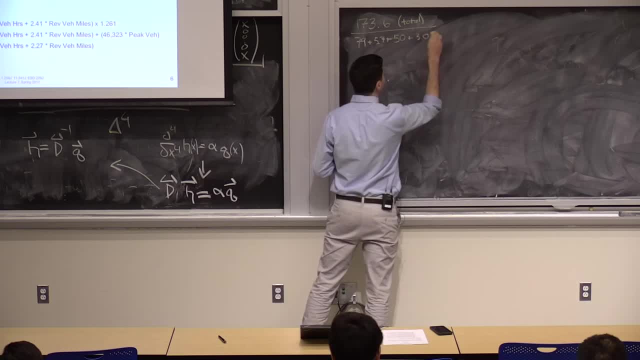 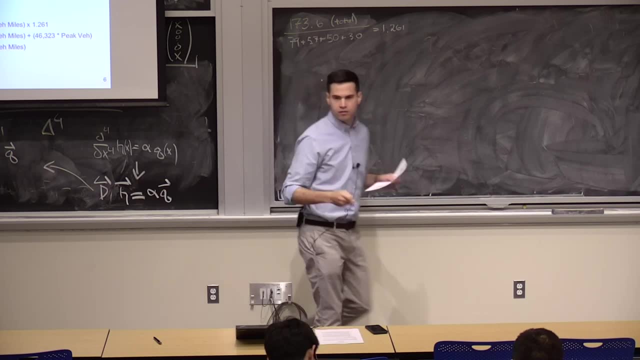 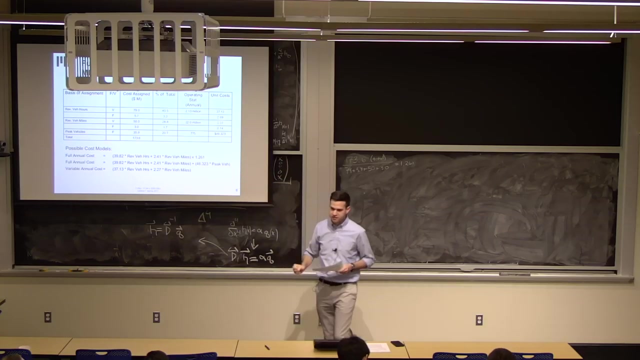 Plus 3.. Plus 3.. No, it's plus 3.. And last, equals 1.261.. No, OK, so we're dividing the total by the amount that we did capture and then the factors of the model. So this is a very simple model of a full annual cost. 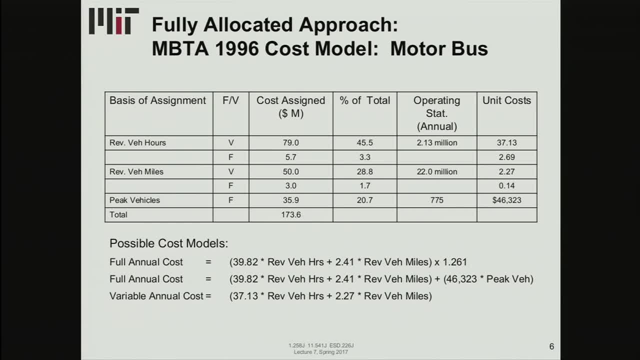 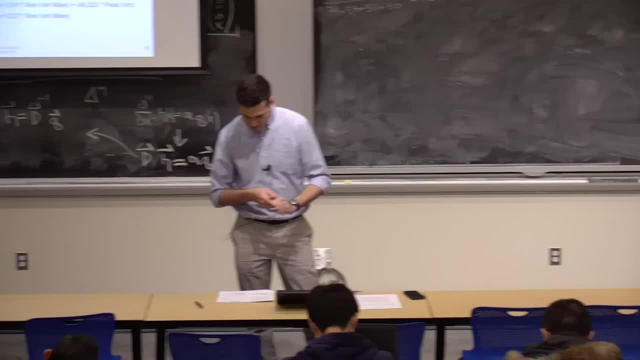 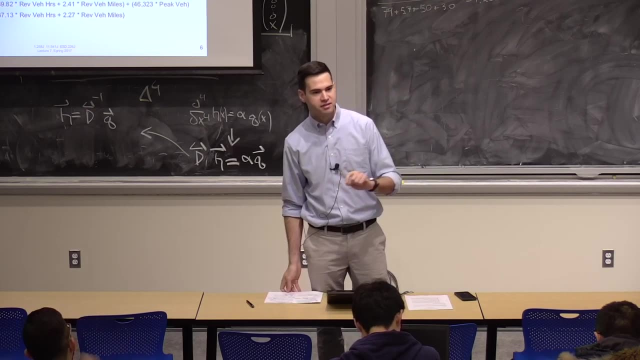 for the agency. We're looking at the fiscal year And it's sensitive to two variables, It's not sensitive to time period And it's mixing fixed and variable costs. So this model may not be the best one for some applications. What's the intuition behind using 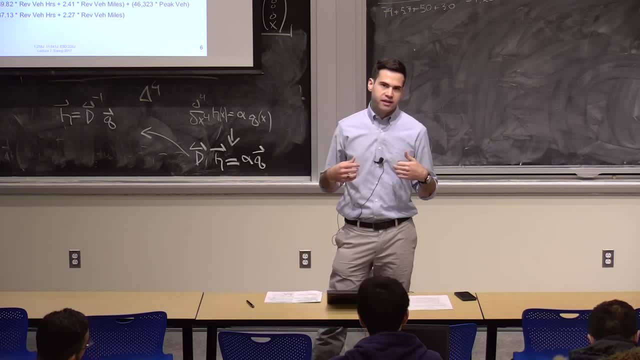 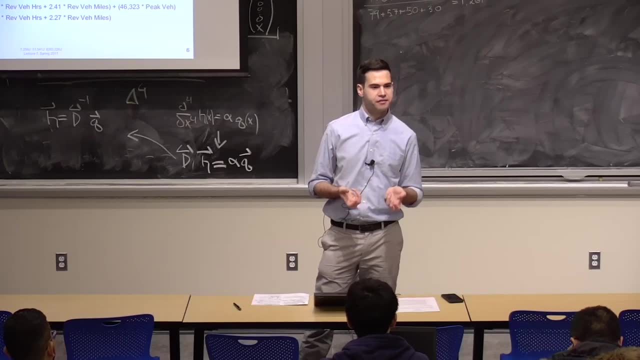 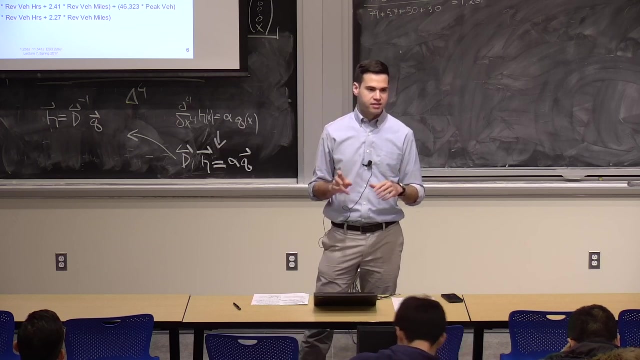 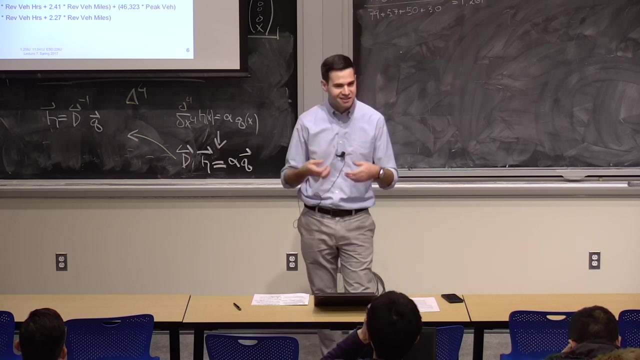 vehicle hours and vehicle miles. It's something that agencies always measure and report. So it's something that there's already a data collection effort for it. If you think about especially the traditional obligations without automatic data collection, there's an effort to measure anything you deliver or collect. 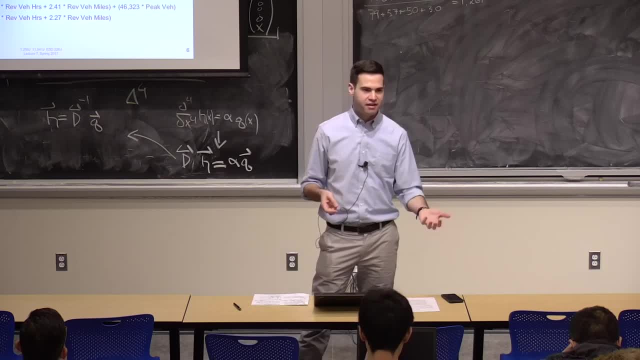 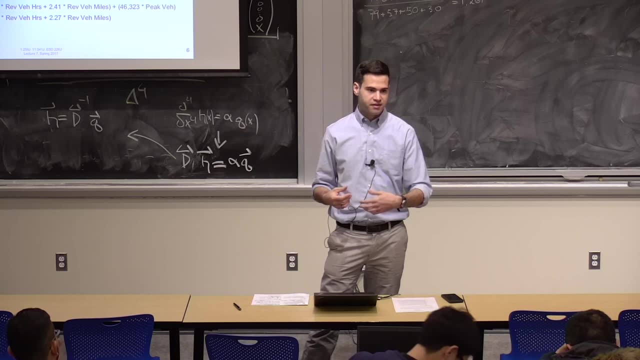 how much, How much output you produce, And so we already have that. It's something that then you can use an explanatory variable And it relates to service right, So it's your service output. So, if you want to, these are variables. 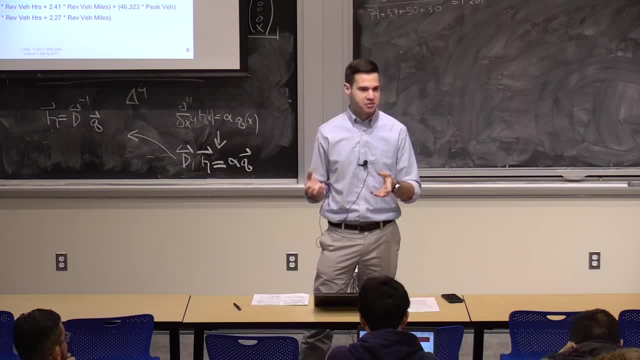 that are also going to be found in any service planning proposal. in some way or another, If you extend routes, then that increases both of these, right, I guess? my other question was: what's the intuition behind vehicle hours being relatively more expensive than vehicle miles? 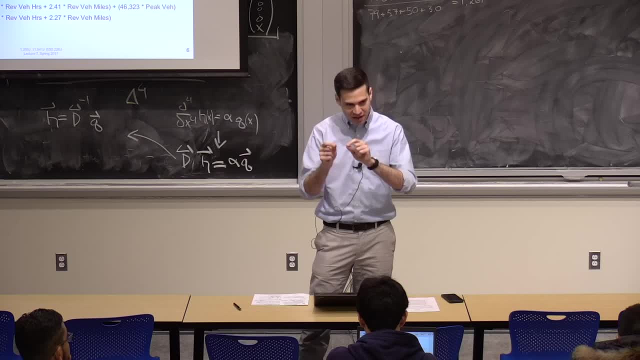 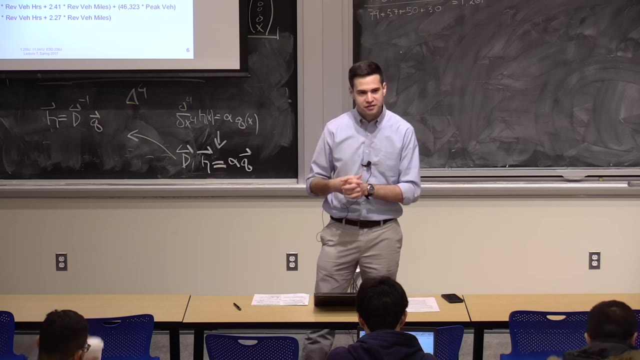 That depends on how you assign each of these cost categories to it. It's not that like operating a bus Well, I mean in this case. wages and benefits are, a principle, one of the key costs for the agency, And that's being reflected entirely in vehicle hours. 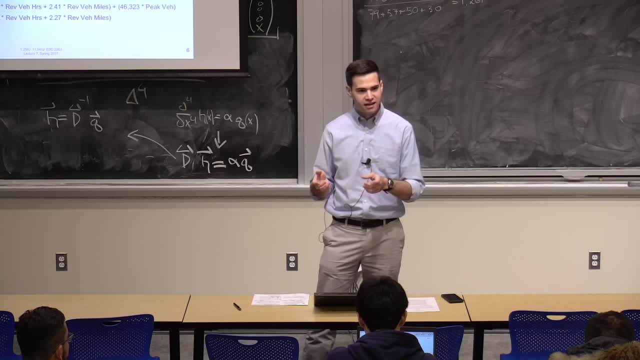 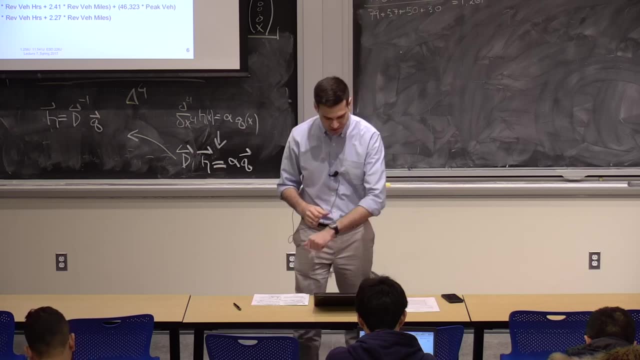 And potentially fuel is a second one, And that is at least partial, And that's actually covered by running vehicle hours. It could be, I'm not sure, in this model. if it is, I suspect that everything was assigned to vehicle miles. 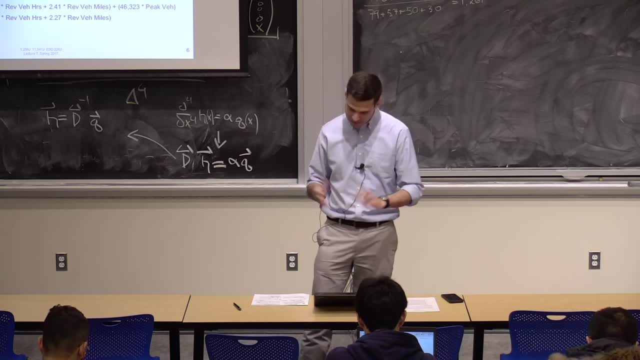 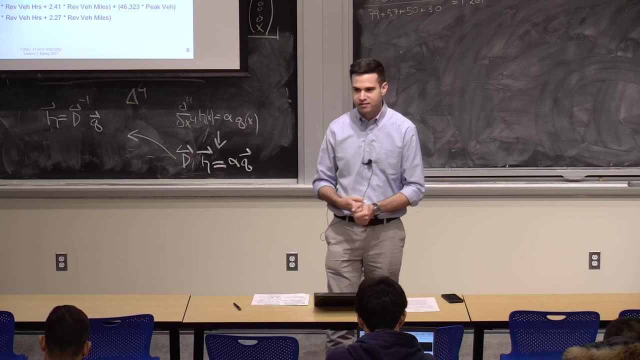 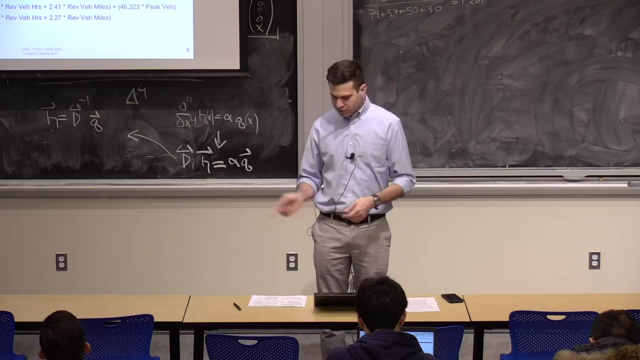 But it could be. So yeah, vehicle hours is the proxy for more things And more costs are being assigned to that variable. Eli, Can you give some examples of variable and fixed costs? Well, yeah, We'll actually see more of those later in the lecture. 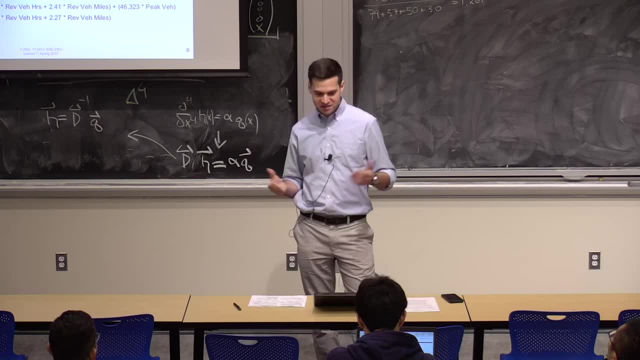 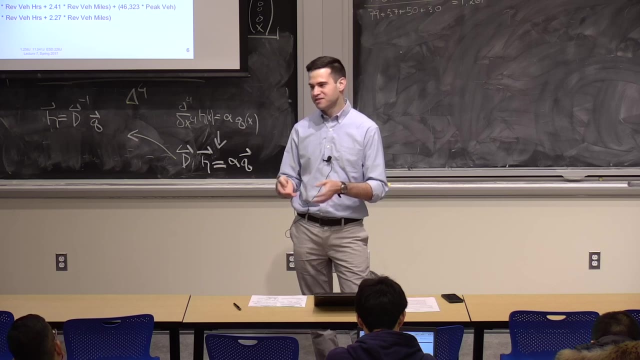 But variable costs. fuel is variable right, Because as you drive more you consume more, And if you all of a sudden operate less service, then you'll see that drop immediately. A fixed cost could be the administration costs for let's. 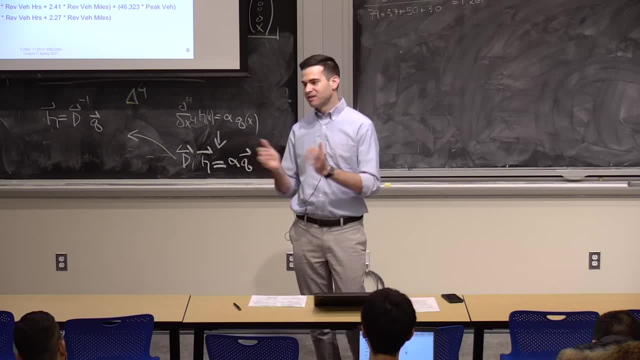 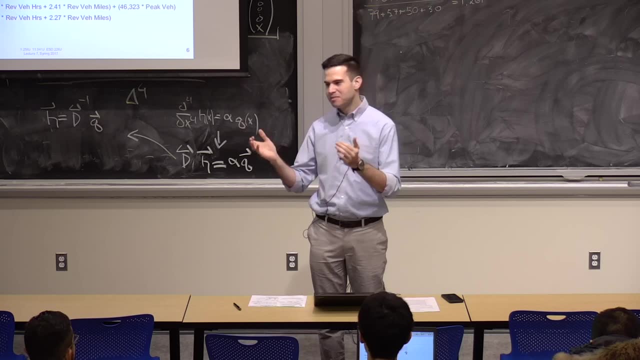 say a bus, And that's going to be your service planning team, right? So you've hired people. And if you drop service a little bit, you're not necessarily going to fire people. Or if you expand service, you're not necessarily. 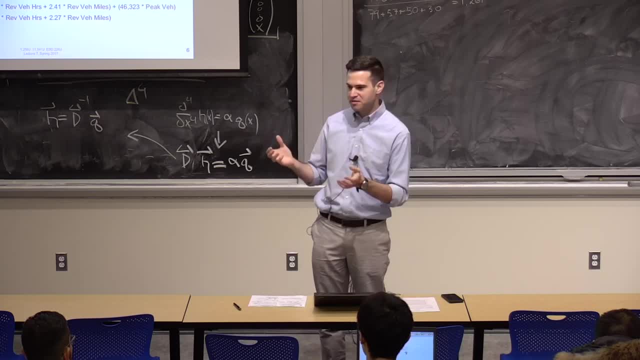 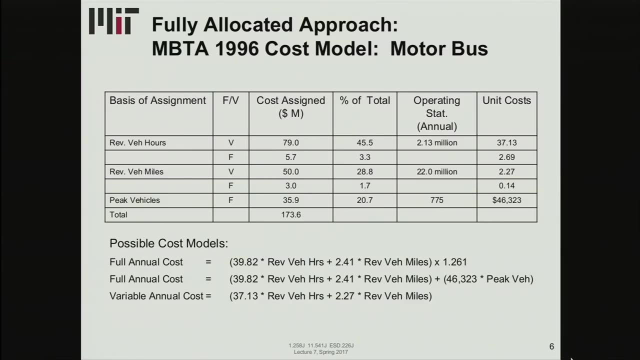 going to hire a bunch of people, Or you may not need new offices for them. So all those things are more fixed. Thanks, OK. OK, second model. So here we have the same first part of the model. Using the adjustment factor, we directly 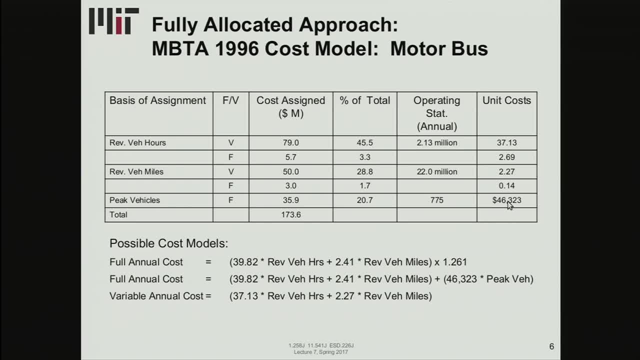 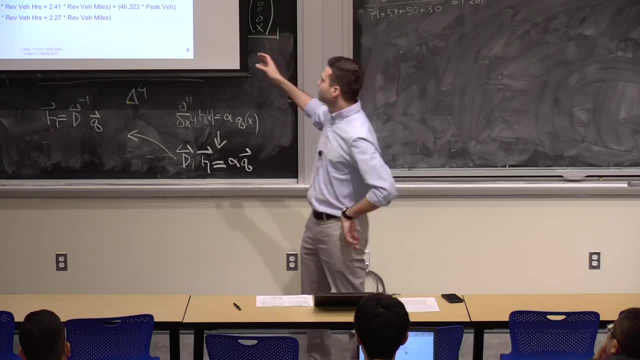 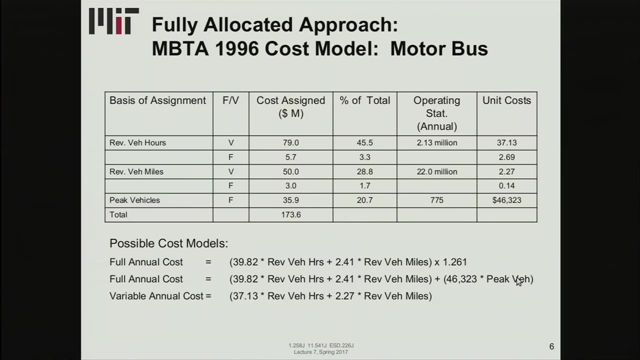 take the unit cost of peak vehicles and add it in, So now we have a model that is sensitive to peak vehicles as well. OK, And we don't need the adjustment because all of the things that have been assigned to vehicles are being directly related to vehicles. 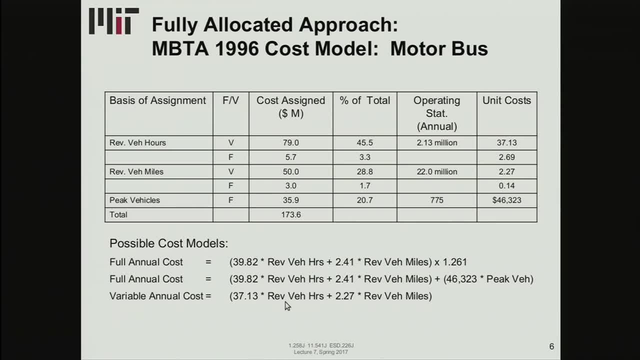 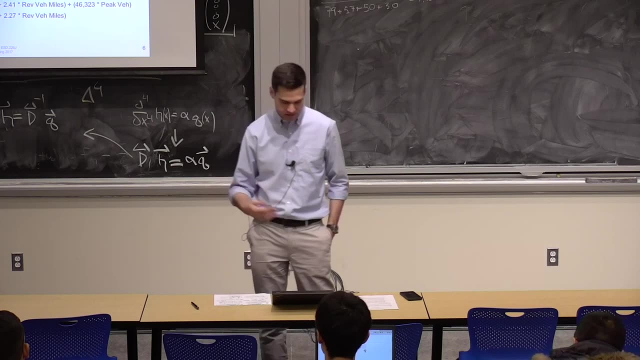 So it's a simple variation And here we have a variable annual cost model. So these first two have all of the costs. It's fixed and variable. But for some applications you're only interested in variable annual cost, And I've given the example of minor expansion in service. where you add a little bit of service or remove a little bit of service and you wouldn't expect to incur fixed cost as a result. So here we then only consider the unit costs of the variable portion of revenue-viable hours, which is 37.13 and 2.27 for revenue-viable miles. 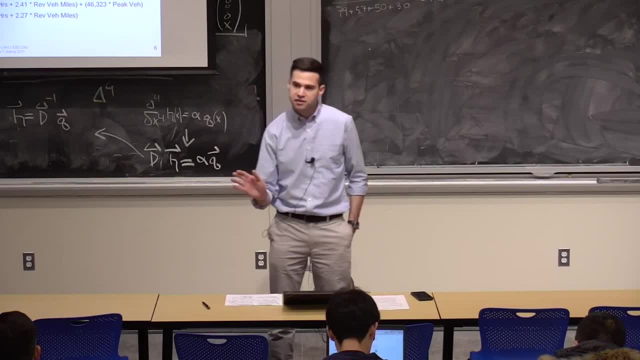 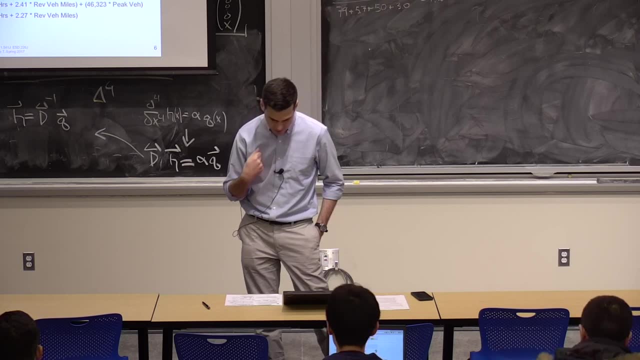 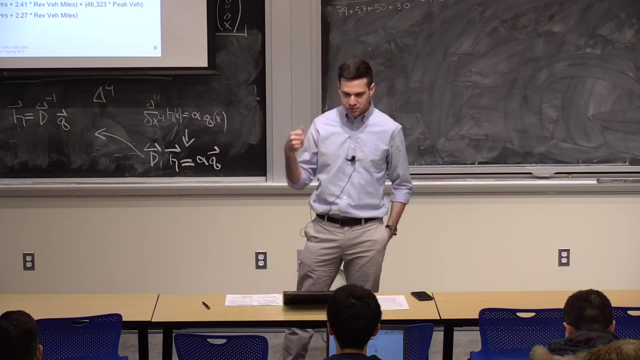 OK, Any questions on these simple models? OK, as I mentioned before, one of the key weaknesses of these models is that they're not sensitive to time periods, So it's much more expensive to operate service on the peak than it is off-peak. 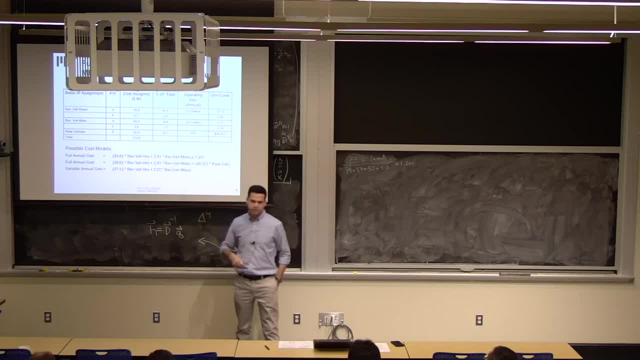 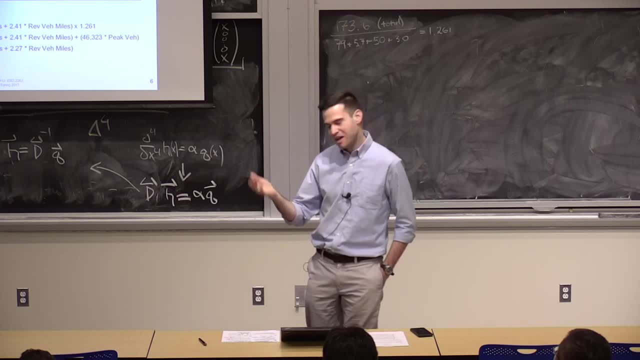 So if you were to use, say, the variable annual cost model for the bus routes 70 and 70A, and now you want to expand it to say go to Kendall or Lechmere or somewhere else, and you have a greater number of revenue-viable hours, and revenue-viable miles. maybe if you expand service proportionally throughout the peak and off-peak, you're fine. But if you only expand service on the peak or do it disproportionately peak-off-peak, then this model will not capture those differences very well. 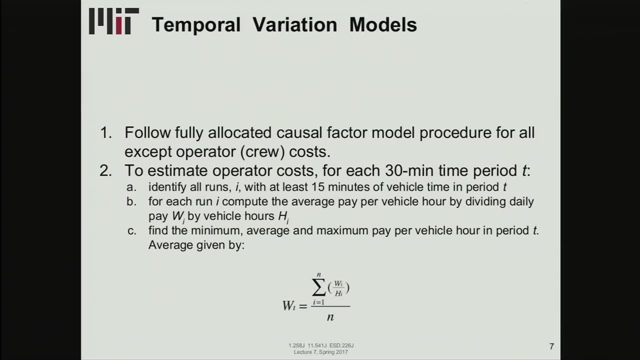 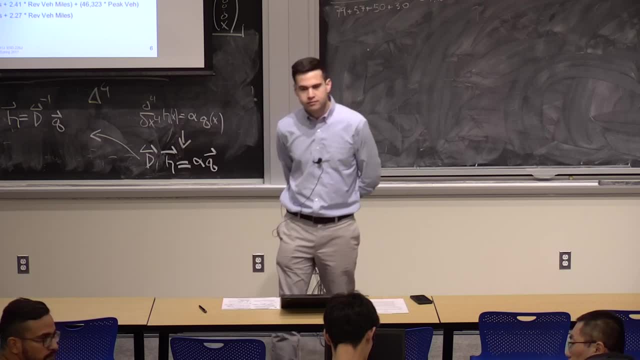 And for that we need a temporal variation model, which is our next, Just a second. But why wouldn't it capture it? Because, suppose I add service, Suppose I add a bus in the peak, So now peak vehicles, that gets impacted. 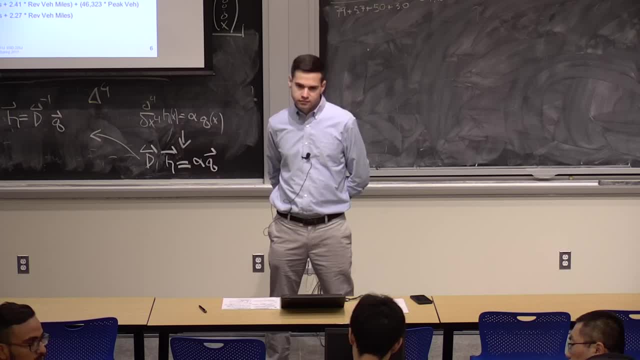 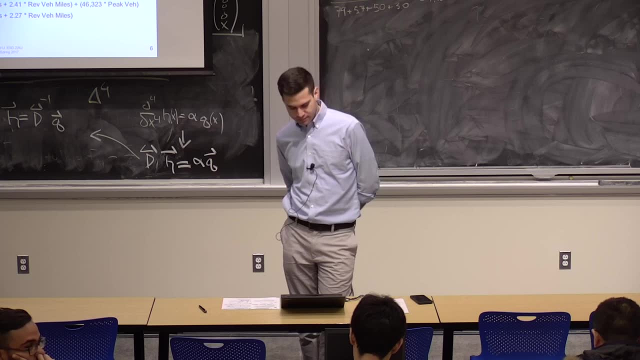 And suppose I take fuel and I say, OK, fuel affects revenue miles, but also it affects revenue hours. I put fuel in twice, both in the hours and the miles. Now I can also take into account the fact that the bus is sitting in traffic and burning fuel. 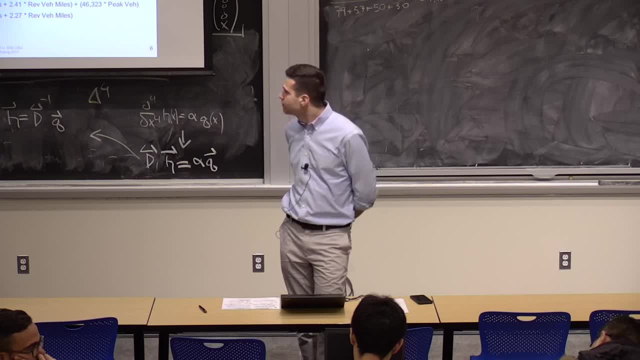 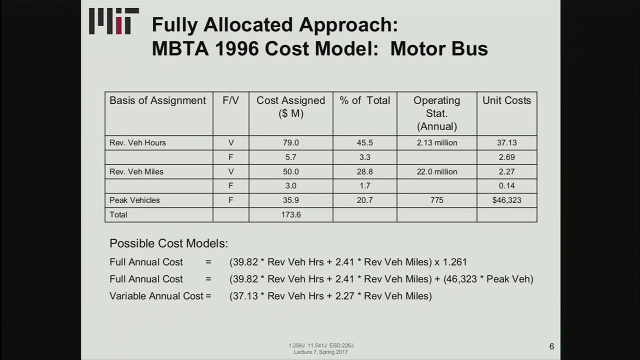 but I'm taking that into account. So why is this model? necessarily It goes back to the question: is: why does this model not adequately capture peak versus off-peak costs? So it goes back to this: calculating average costs by factor. So these are averages. 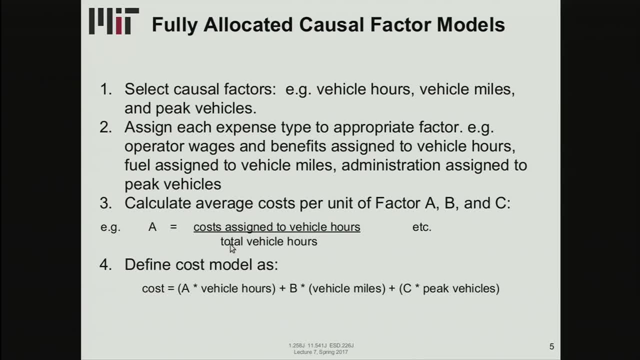 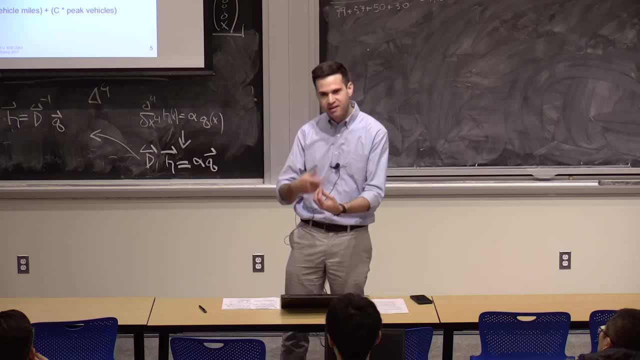 We're taking averages of all the vehicles at all times of day and dividing by explaining them with an explanatory variable, that is not necessarily what is directly costing it. So especially driver costs are going to vary a lot by sort of peak off-peak. 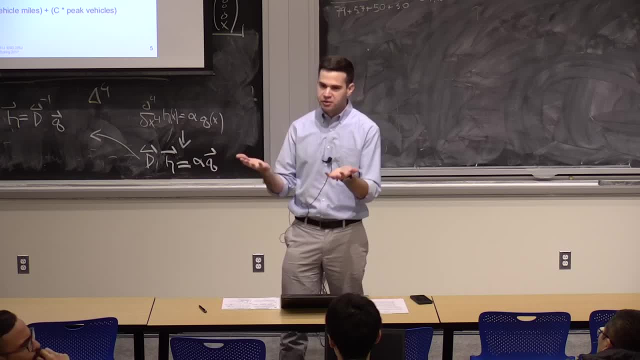 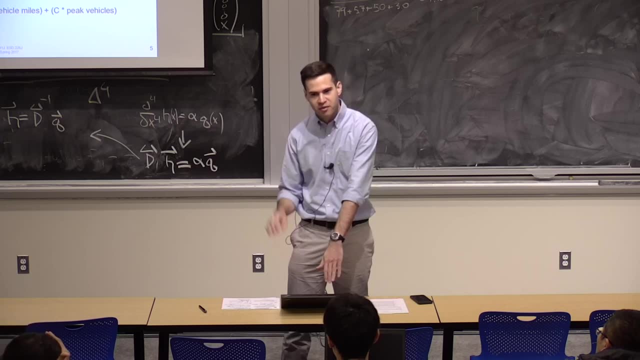 And we're taking an average. So if you increase service proportionally, you're fine, But the unit cost is not reflecting the difference between peak and off-peak, So it's the unit cost itself more than the independent variable that you put in, which is what you're saying. 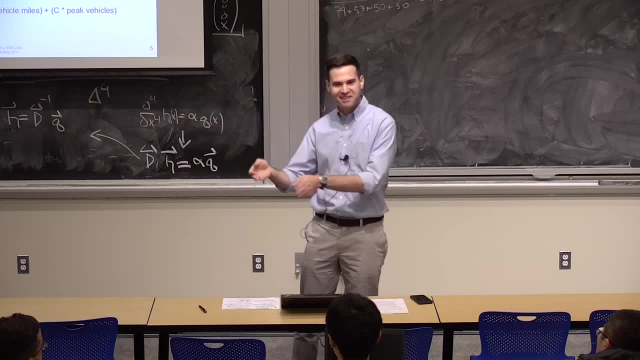 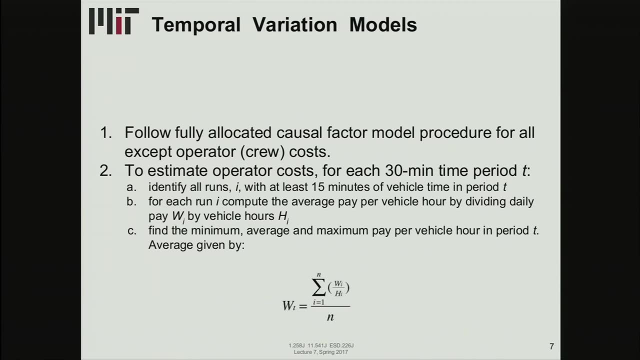 You're saying I can measure the independent variable precisely, so I can plug it in here. Well, but your factor is average And that's it OK. So the, So the approach of this model, which is an extension of the first one, 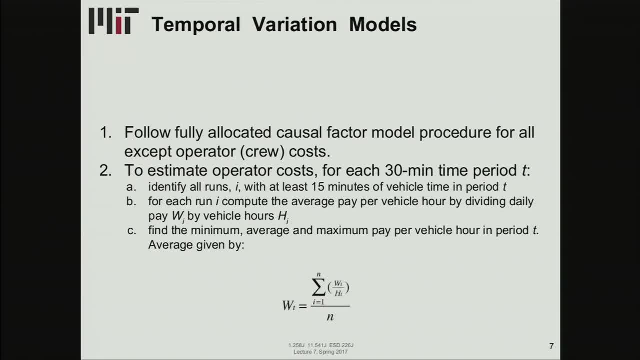 is to do everything that we did, except for driver costs, because these costs are very sensitive to time of day. And for those costs, for crew costs, we take the day, We divide it into 30-minute periods And then we look at all runs. 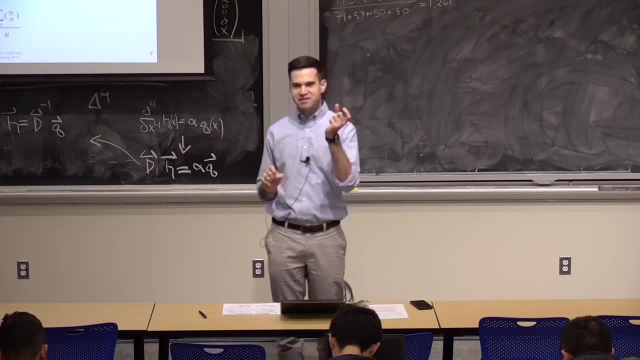 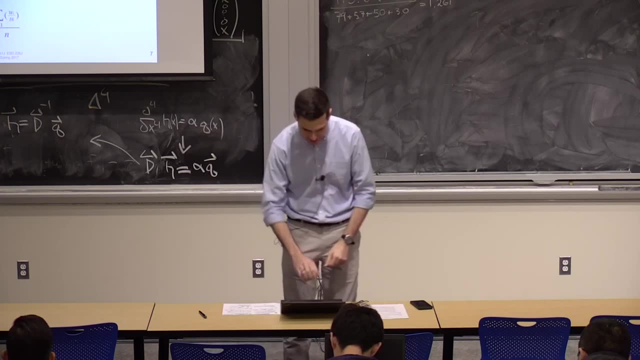 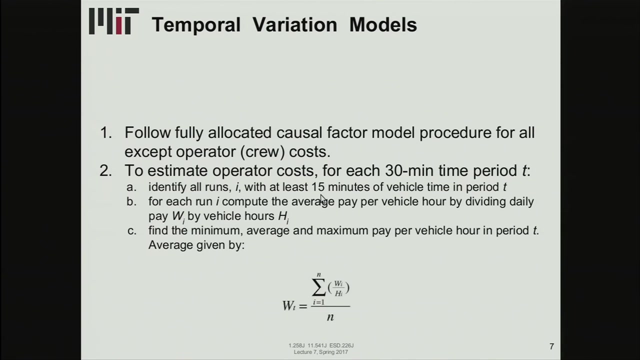 Now, a run is what a driver does in a day, It's their shift, It's a sequence of trips that are being operated by a single driver And we look at all runs and all periods And, for each period, any run that. has at least 15 minutes in that period gets included in that period. And then we compute the average pay per vehicle hour by dividing the daily pay by the number of vehicle hours over all runs in that period. So each of these runs is going to have a different cost. 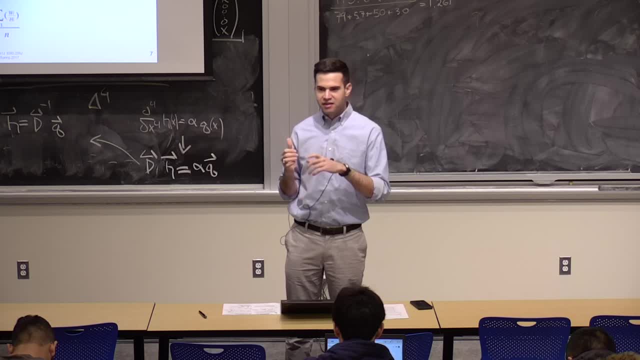 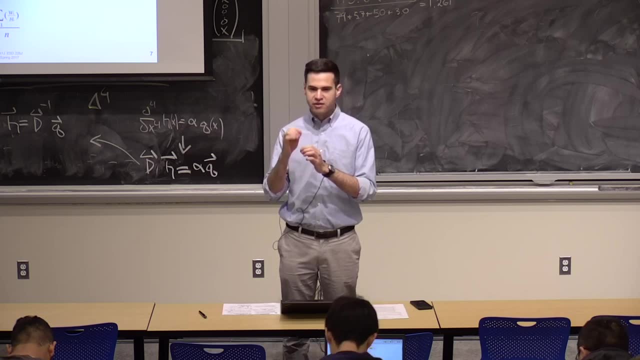 Some runs are going to operate more in the peak And they're going to have more overtime, for example, or more spread penalties- And we'll talk about those now- And so those runs will be more expensive. Other runs that are straight are going to be less expensive. 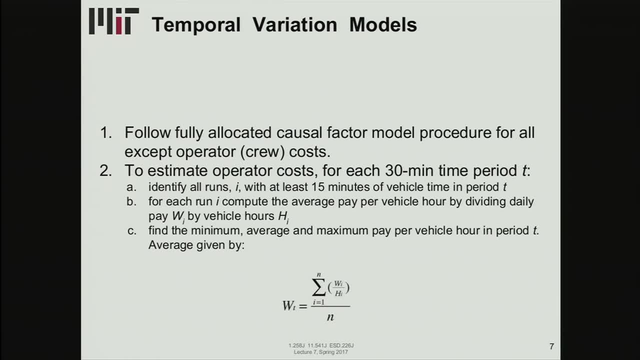 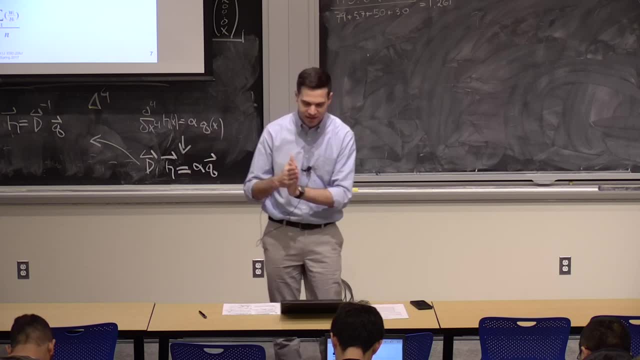 And you can calculate an average for each 30 or 15-minute period. So now we have an average again, but it's by time of day, for a small bucket of time And then for each of those we find, and the minimum, the average and the maximum. 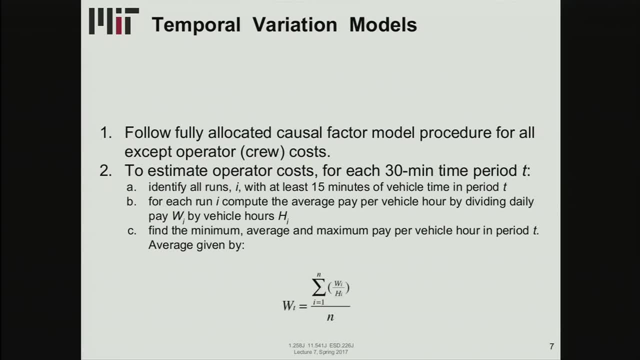 So we're not only going to look at averages, We're going to also look at the distribution of costs along each period. And this is just an equation for average. What we have here is the sum over all runs in a specific period. This is the wage, the total pay for that run, divided. 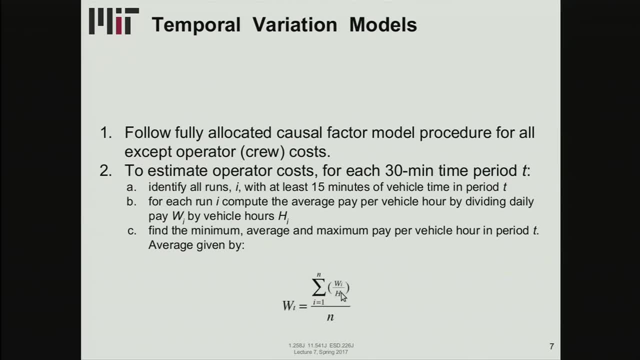 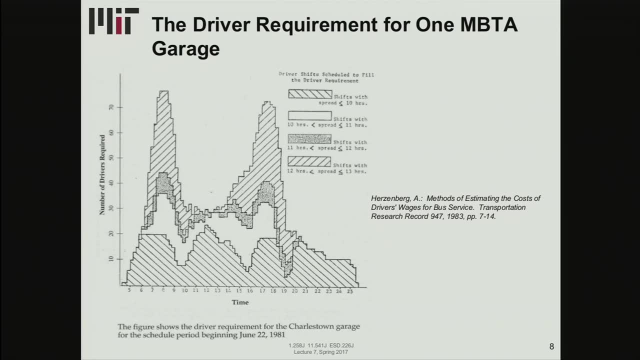 by the number. We have hours for that run, So we compute the average. If we look at the driver requirements for the MBTA back in 1983, the early 1980s, this is what we get. So many more drivers are required in the am. peak and the pm peak than are required off-peak, or early in the morning or late in the afternoon and evening. Why is that? We've talked a little bit about it already. So you provide more service. Why do you need to provide more service? 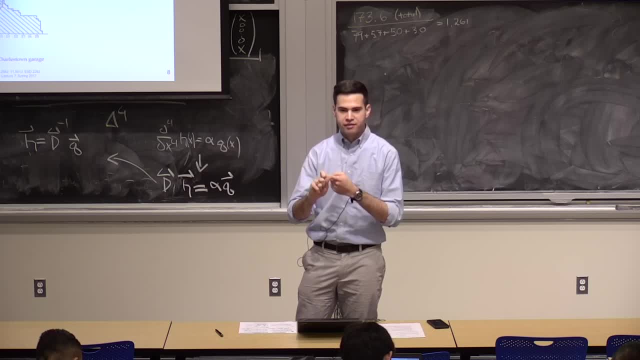 Because that's where the computers are moving. GABRIEL SANCHEZ- Because there's more demand for it, right? So if you provided the same level of service, your buses would be too crowded And you would not deliver enough capacity. What else? They're also in traffic more, So buses are in the traffic, GABRIEL SANCHEZ- So every trip that you run takes longer And it's stuck in traffic And the dwell times are longer, Right? 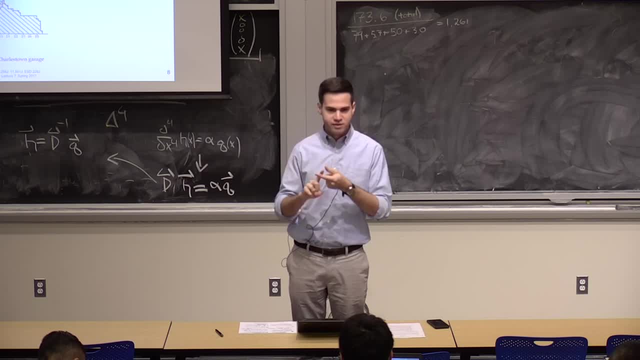 So OK. So if you need more, if you need to provide more frequent service and each run that you do, each trip that you run is slower, then that means that you have a greater cycle time and a greater frequency and therefore a greater vehicle. requirement from your first assignment, right? And of course you need drivers to drive those vehicles, So your driver requirement also goes up. Great. So what's wrong with the time? What's inconvenient about the timing of the peaks? Right, Because they're eight hours apart. 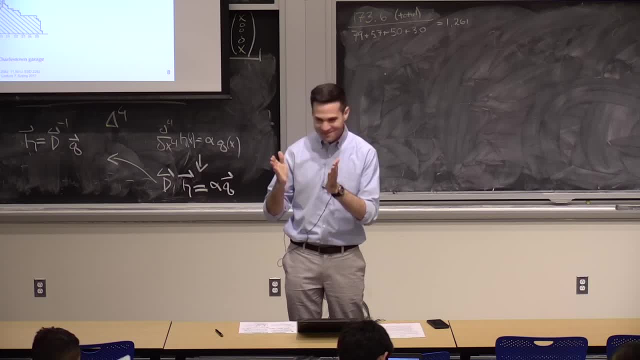 GABRIEL SANCHEZ- They are eight hours apart. And how long are shifts? typically Eight hours, GABRIEL SANCHEZ- Eight hours long, Great. So if we hire someone to start their shift at 6 AM? 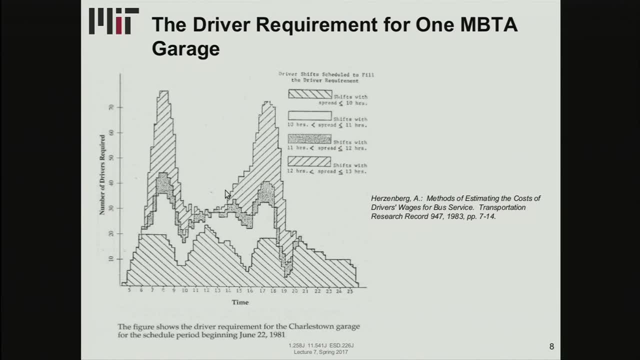 they can't cover the PM peaks. They only cover the AM peak. OK, so what do we do If one option is to hire part-timers? So use full-time employees for the base and then hire part-timers for the peaks. 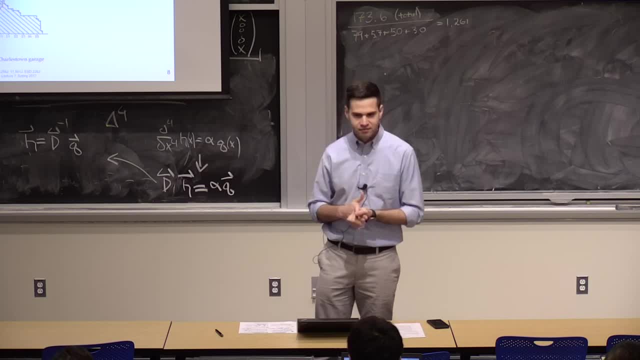 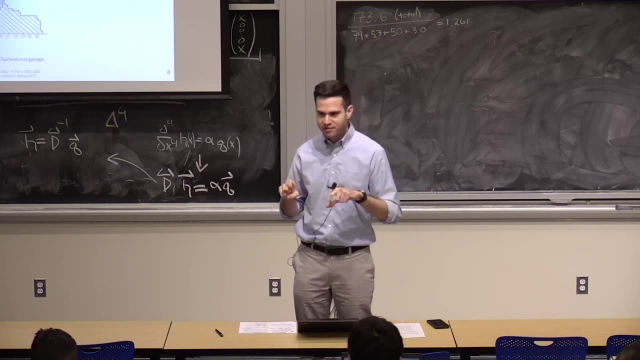 That's the least expensive, That's the most efficient option. But unions don't like it because if you have a high percentage of part-time drivers, then it's not to the benefit of their union employees. If you don't allow part-timers or you. cap the allowance on part-timers, then the agency is required to hire full-time employees to cover the AM and the PM peak. And if you only do that, then that's terribly inefficient because you're hiring for eight hours. Then you can only operate two or three. 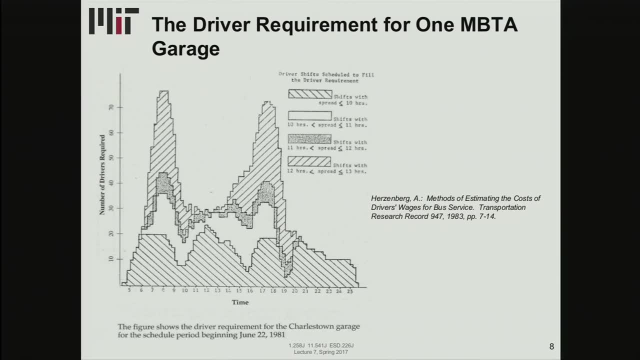 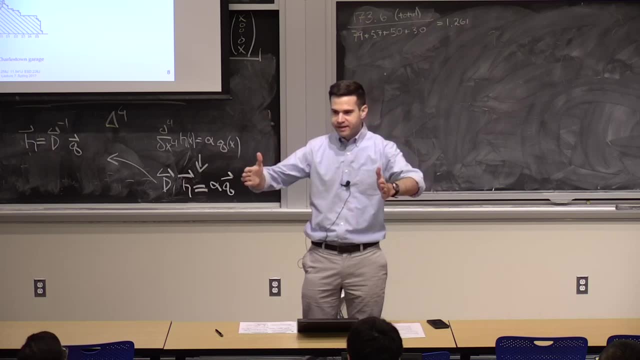 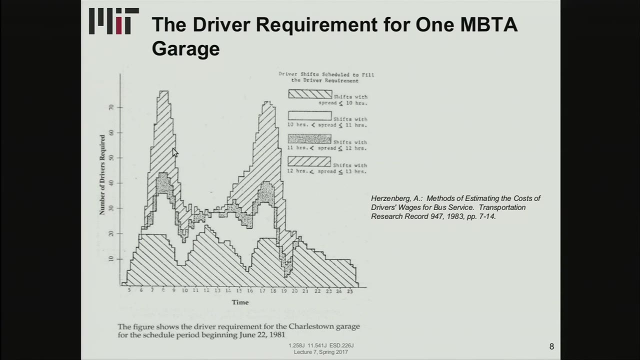 That's all that you need that driver for. But there is some arrangement. You can actually have shifts that have a break in the middle of the day, And these are called spread shifts. So some of these shifts operate for two or three hours in the morning, have a long break during the day. 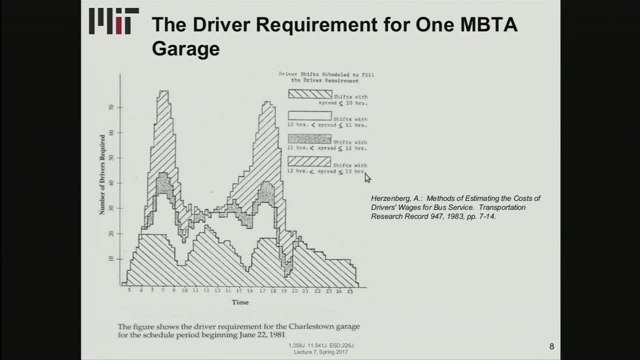 and operate for two or three hours in the afternoon, And often. GABRIEL SANCHEZ- Yeah, That's the best way to do it. GABRIEL SANCHEZ- Yeah, That's the best way to do it. 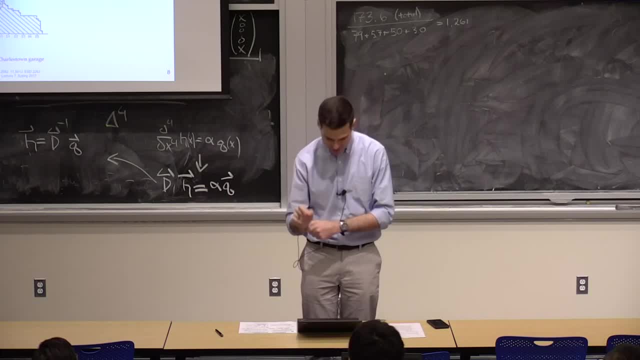 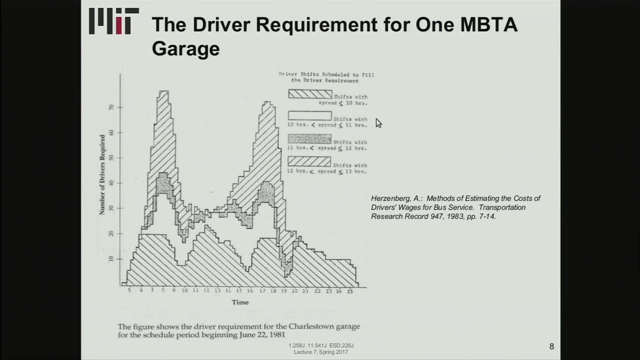 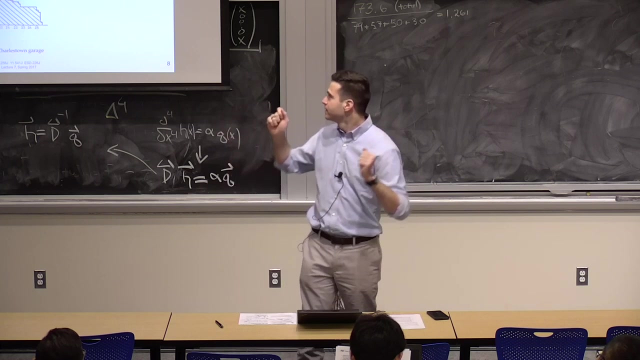 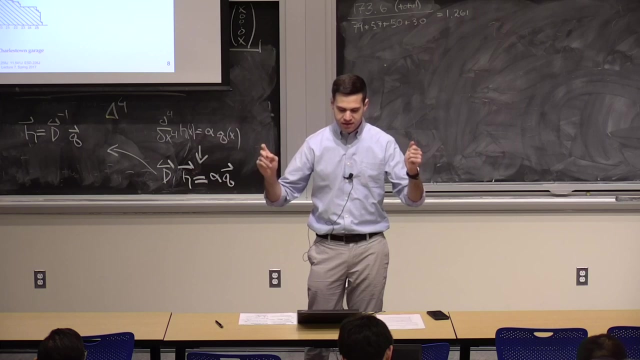 Often these shifts are paid a spread penalty. So in this example, what we have in white here are shifts that last between 10 hours and 11 hours. So the spread is the difference between the checkout time and the check-in time, And shifts in white here have a spread between 10 and 11 hours. Those drivers are paid a 50% premium for any hours above 8 hours. And then there are these other shifts that are between 11 and 13 hours. So 11 and 12 in dark gray and 12 and 13 shaded diagonally. These shifts are paid 100%, So they're paid double for any hours in excess of 11, in this case. So that's going to drive. That's going to drive costs up because if you look at the total pay for that shift over the day. then the unit pay per hour for each of those drivers is higher And if you look at any time slice of the day, peaks are going to have many more of those drivers than off-peak. So the average across the drivers on any bucket of time. 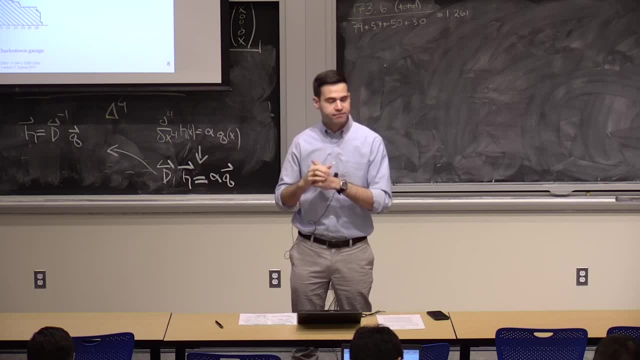 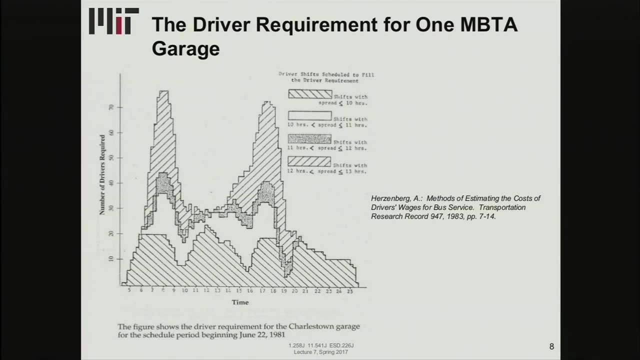 that's 30 minutes wide, is going to be higher. So could you explain maybe for, like, let's say, I'm a driver that runs the shifts with 12 hours less than the spread 13 hours. the bottom one, GABRIEL SANCHEZ- This one, yeah. 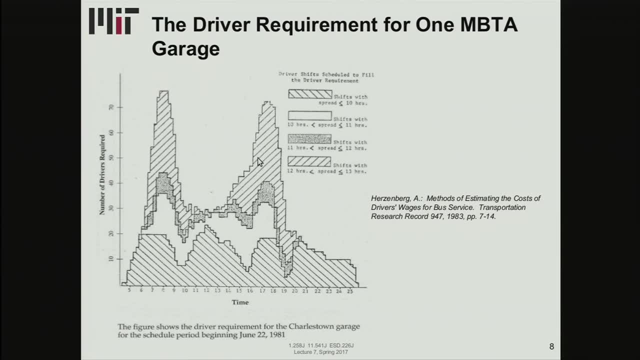 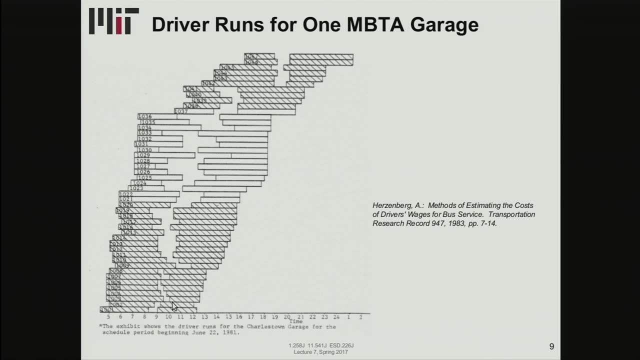 So what? they're driving the peak ones. yeah, GABRIEL SANCHEZ- When would I work? And then what hours would I get paid for? Excellent segue for the next slide. So here we have, essentially the runs by driver. 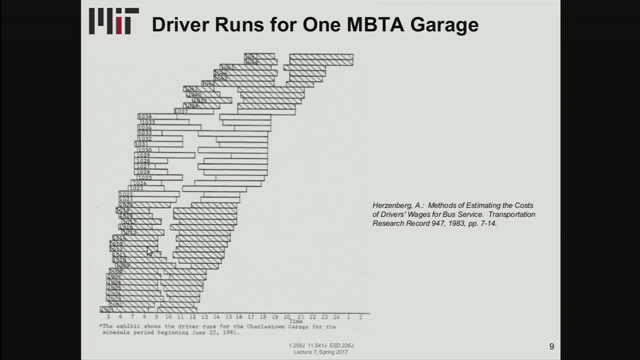 And you can see if you draw a line here: this is 8 AM, So AM peak, And then this is 5 AM. GABRIEL SANCHEZ- OK, This is 5 PM right around here. So you see that if you draw a line between 8 and 5 PM, 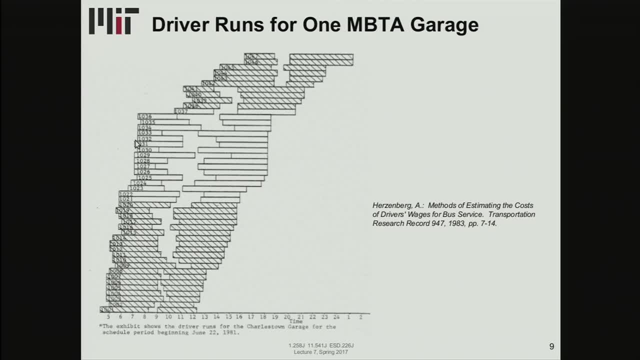 these are the shifts that start during the AM peak right And those shifts have the biggest spreads. So any one of these rows is an example of one run And you could be one of these drivers. So if you have this day, you check in at 630.. 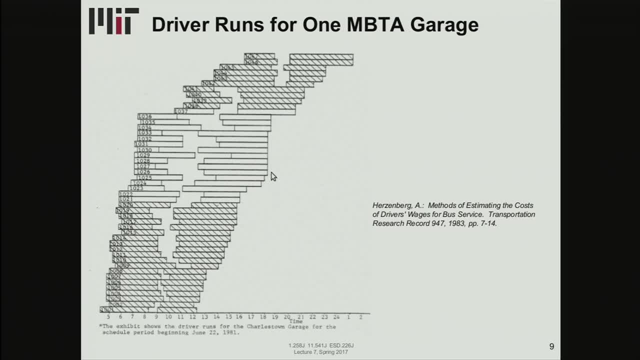 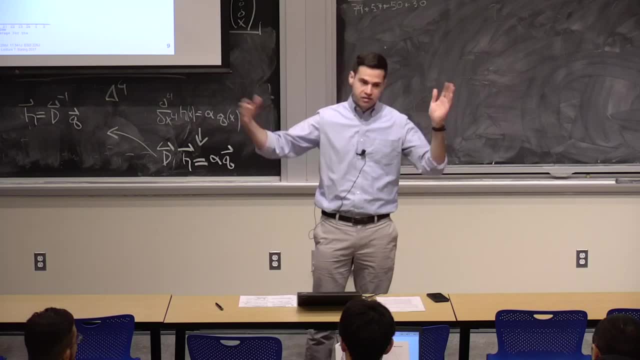 You have a pretty long break during the day And you check out at 8, at 6 PM, So you do an hour in the PM peak And you could have longer ones too. There will be some rules that prevent excessively long ones. 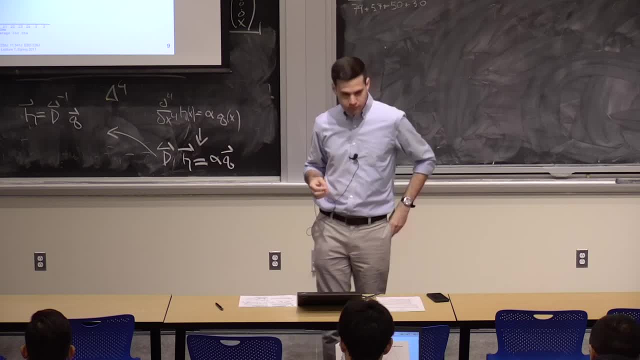 GABRIEL SANCHEZ- And when you were saying I get paid 50% more as a bus driver, do I get paid 50% more for only the hours that I'm working? Yes, GABRIEL SANCHEZ-, OK, yeah. 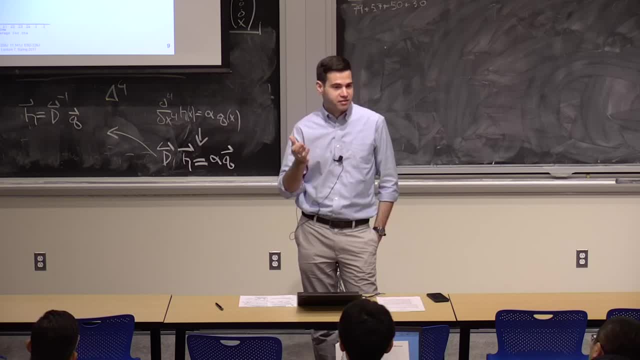 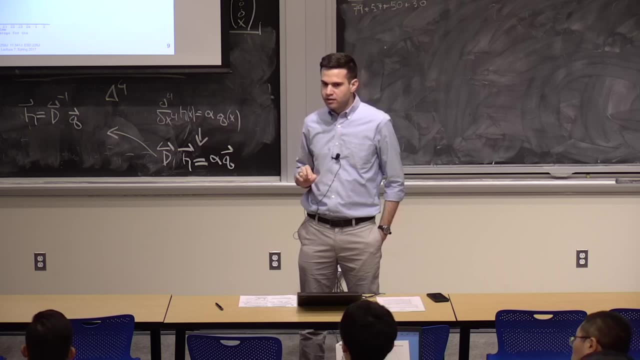 Yes, And that will vary by agreement. So that's specific to this labor area. GABRIEL SANCHEZ- But like we are in a competitive- I mean during the shifts- So you are paid the spread penalty And you are paid. There are a bunch of rules. No matter how many hours you work, you're paid a minimum of eight. There's a swing pay bonus, So if you start your day somewhere different than you end the day, then you have to pay the person- I think 30 minutes extra for their driving. 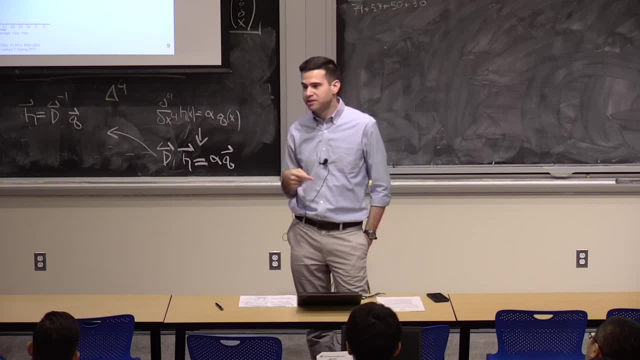 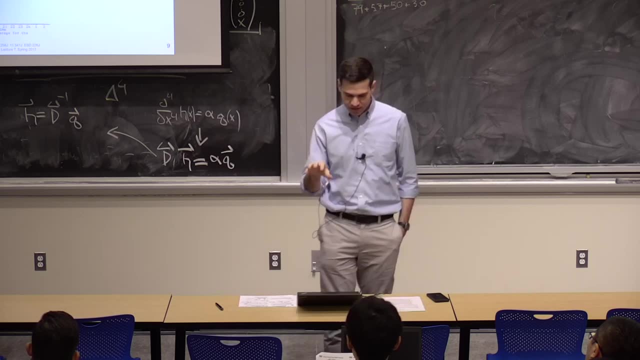 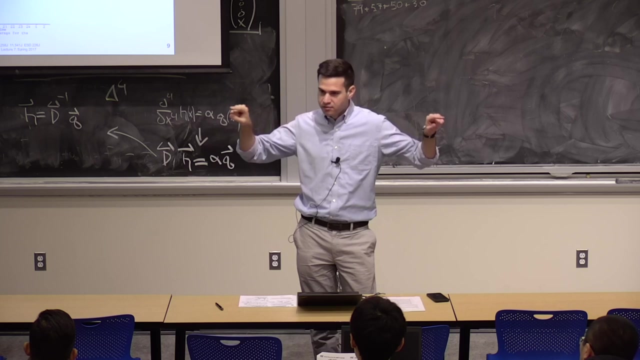 time or whatever for getting to the other location where you potentially left your car. So there are Compensations for all of these things, And the point here in this cost modeling lecture is that these drivers with large spreads cost more. So we want to build a cost model that recognizes those differences, especially with regards to driver hours. So we expand service and require more driver hours, more in the peak than in the off-peak. then we need to account for those differences. Here is a graph by time of day of the wage. 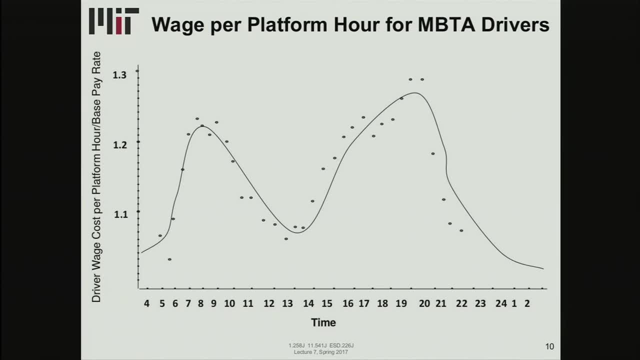 cost per platform hour, just by hour, divided by the base pay rate. So off-peak, you see that the average is very close to 1. But if you go to the peak then you're paying an average of, say, 25% higher. Because some of the drivers are straight shifts but there's a mix of drivers that are spread, large spread, and being paid some spread penalty, So that drives the costs up. OK, here's an exercise to solidify this concept. Before that we have a question. Is it uncommon that the employees stay night at his workplace? I mean that someone starts working at night and drives on buses or trains and they fall asleep And after that they restart their job And they work in the morning. So for safety reasons, a lot of labor agreements. require, and any work rules require, a minimum amount of break between the end of a run and the start of the next one, And that could be 12 hours or it could be. So where that person sleeps is up to them. I suppose most of them go home. But you can't. normally the rules won't allow you to have a run that if you end service at 5, you won't be able to check in at 8 again. If you do a full day that end at 5 AM. you're probably not going to be allowed to start the next full day at 8 AM, because that's not a long enough break and that would be unsafe. I say this because in Japan it is very common to have some place to stay and provide them. 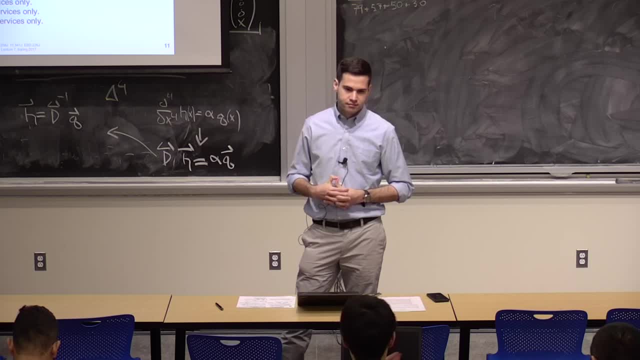 And also it enable us to Run the very late night service and RV morning services. So yeah, I'm just curious about this. I didn't know about that. I'm interested to learn more about it, But would people want to do that every day? or would they be expected to do that once a week? It depends on the shift, but no one continues that kind of shift. You just live at work and you know You would just live at work and do your whole life not doing anything. 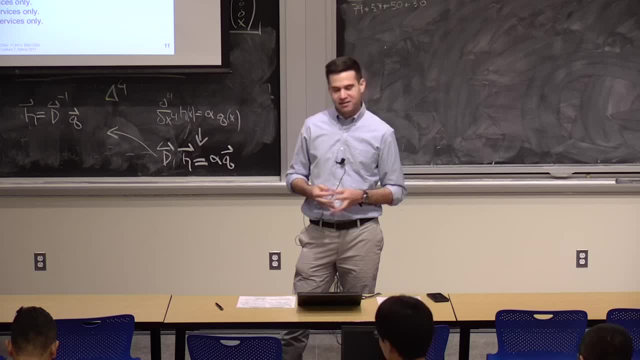 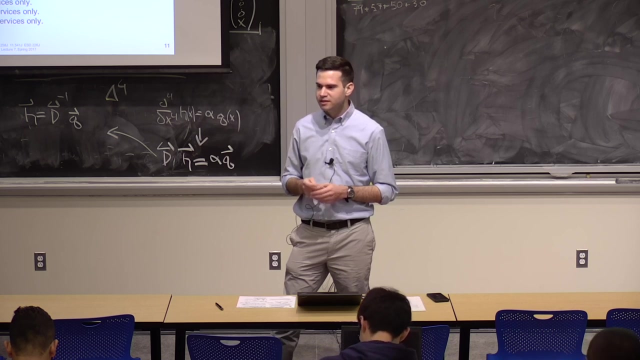 No, So it's a combination. So yeah, these are maybe cultural differences and work rules differences across countries. I'd love to learn more about it. If you have any reference that you can send me, that'd be great Sure. Any other questions? 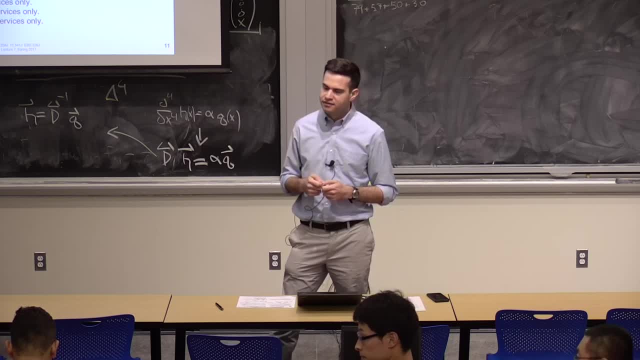 Ari, I think you had a question. Oh, I was going to say, based on Chicago, which runs overnight service, there's so few enough shifts that basically everything that's overnight is a straight shift, And I think when you bid for an overnight shift, 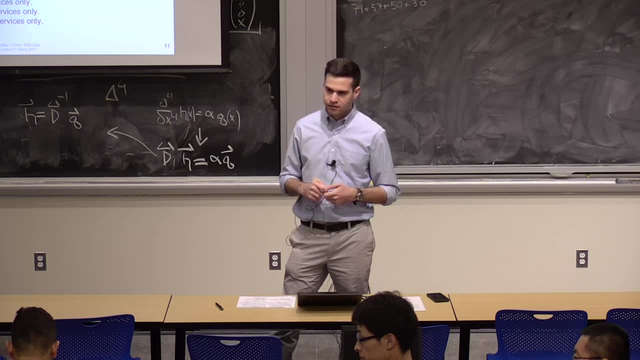 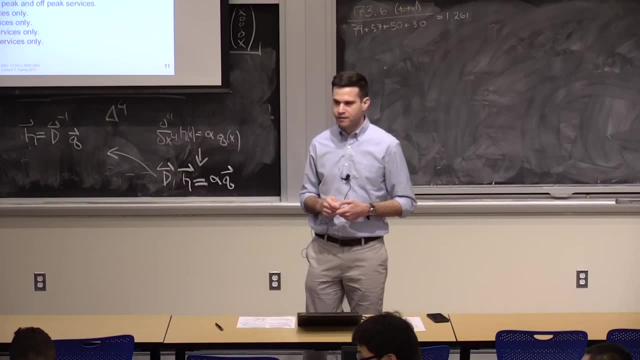 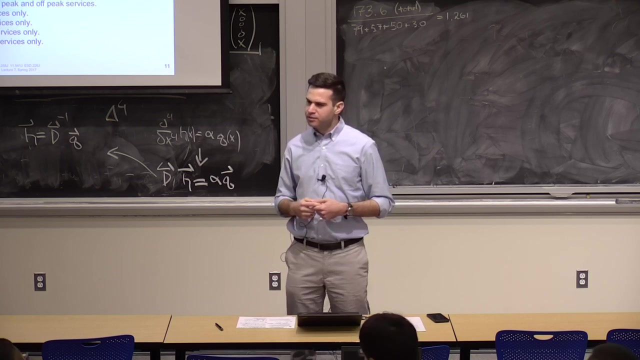 you basically get all overnight, So you keep on sort of that rhythm overnight in a day. And there are some operators that really like the overnight shift because it provides they can care for kids during the day or just like working outside. I don't know what the labor rules are there, but some. Presumably they also get a premium for taking the. There are usually premiums for running on holidays or running late at night, So the least desirable runs might have an extra premium. There's an extra premium associated to compensate for the inconvenience or the undesirability thereof. 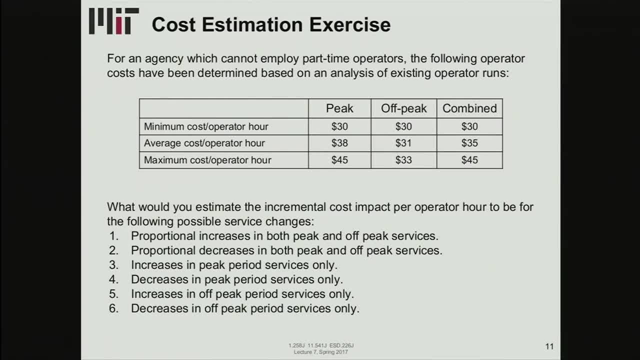 Great. So we have an example here where we've done this exercise And we've looked at all periods of the day and we've looked at the minimum, the average and the maximum unit costs for drivers. so crew for peak, off-peak. 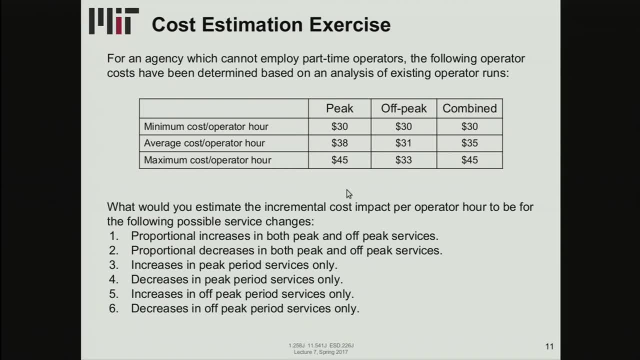 and the combination of peak and off-peak. Six different scenarios, and we want to choose the unit cost for each of these. So let's go one by one. So what happens if we want to increase the peak and the off-peak service proportionally? 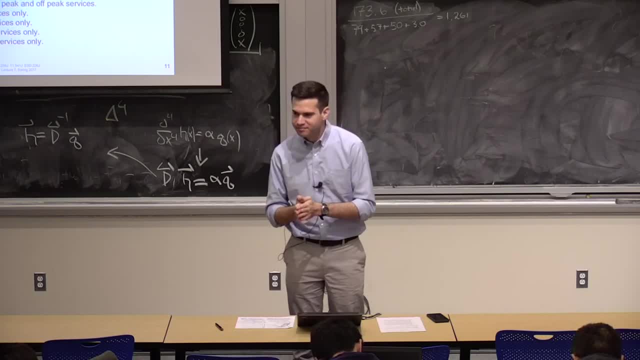 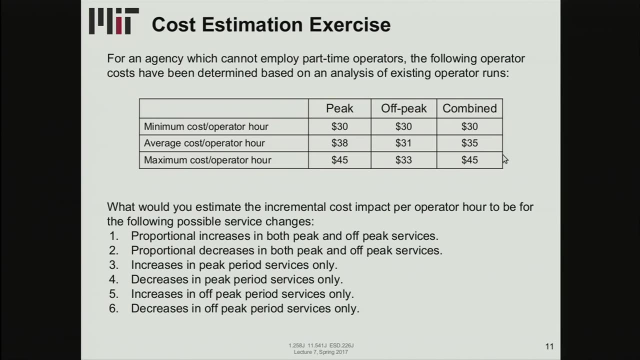 Which unit cost. from this matrix would you use 1.. So we're here in combined agreement? yeah, And from combined would you take minimum average or maximum Average? Average combined: Yeah, OK, And why is that? 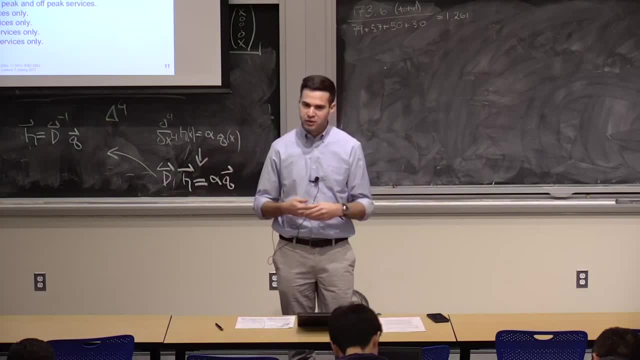 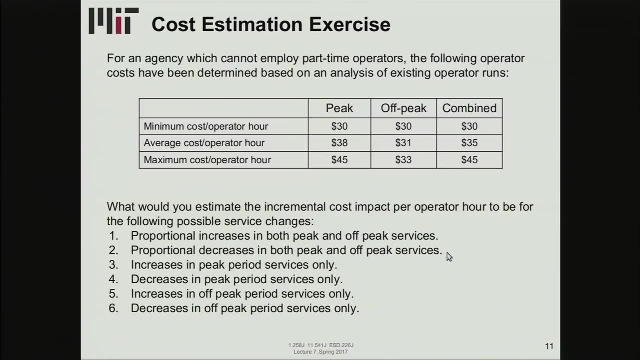 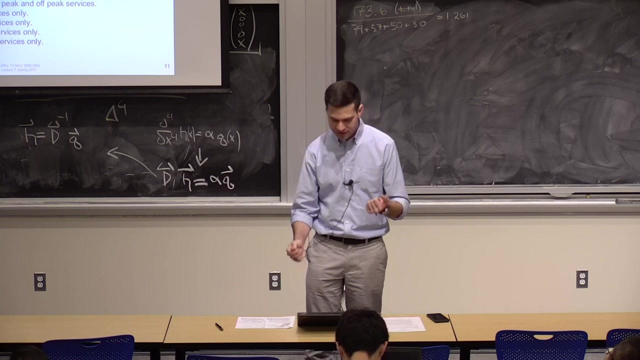 Because it's proportional on both ends and we don't actually need the temporal variation model for this, so we can go with that. What if it's a proportional decrease in both peak and off-peak? Would we use the same one? Some people are saying the same one. 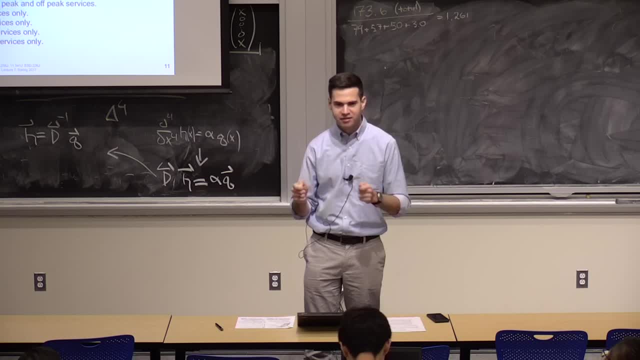 You're saying minimum combined, We have one minimum combined. What's your idea for minimum combined, Minimum maximum, average cost or average cost? Reach out OK. When you say minimum cost or average cost, is that for the peak period or is that for the small pay? So if it's peak, it would be for the peak hours. If it's off-peak, it's for off-peak hours, But minimum maximum average within the peak hour. then there are some drivers that are paid more on average. and others that are paid less Because some of them have spread penalties and others don't. So even in the peak some are straight shifts and those are on the low end Questions. Well, I guess, wouldn't you want to use? 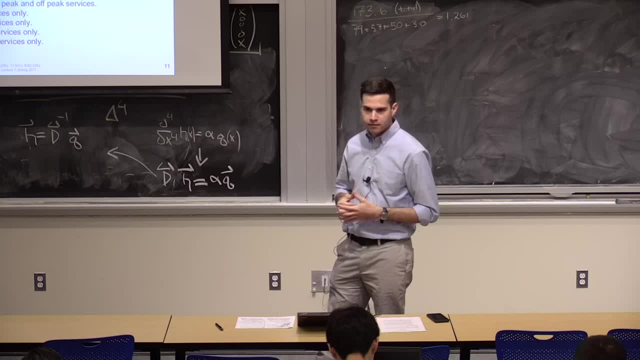 if you were going to add to the peak, was it a bad assumption to assume that it's going to be more expensive than your most? GABRIEL SANCHEZ- We're getting to that. So the third one is increases in peak period services only. 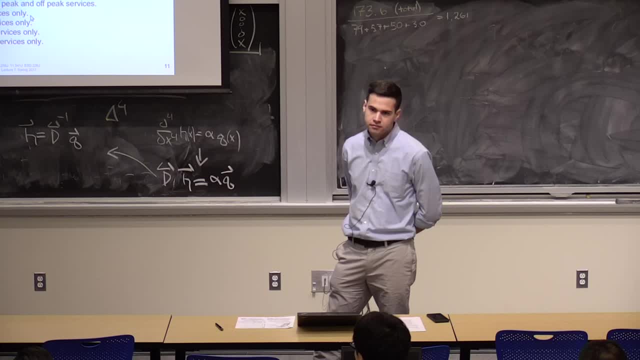 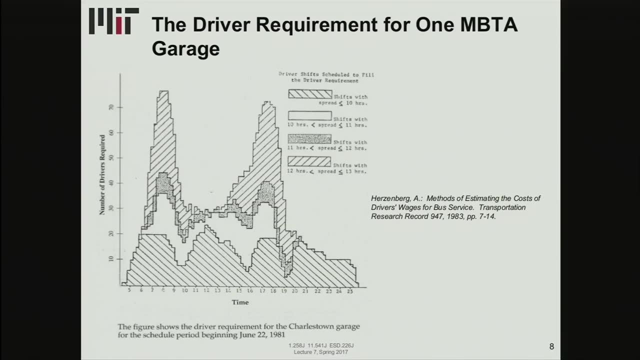 But I guess, when even combined, wouldn't you want to use the max or the min because it's incremental? GABRIEL SANCHEZ- The idea is that if you increase things proportionally, then you're going to have the same mix that you have. 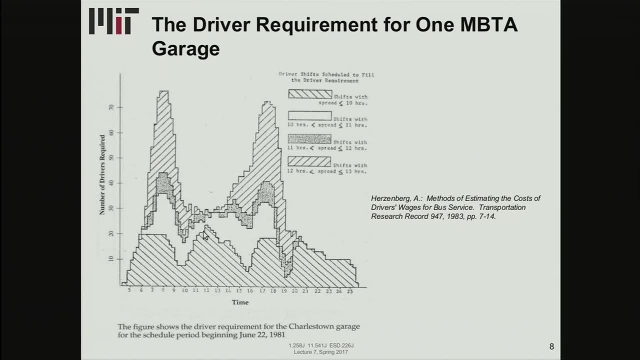 now, but a little more each. So if you add service, both peak and off-peak, in proportion, which means that if there is twice as much peak service, then you're going to add twice much more peak service And then you're going to have the same distribution. 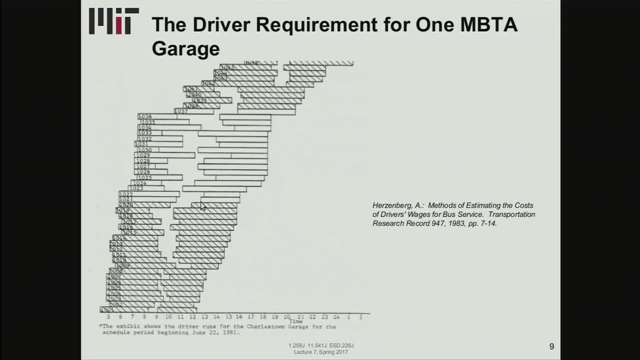 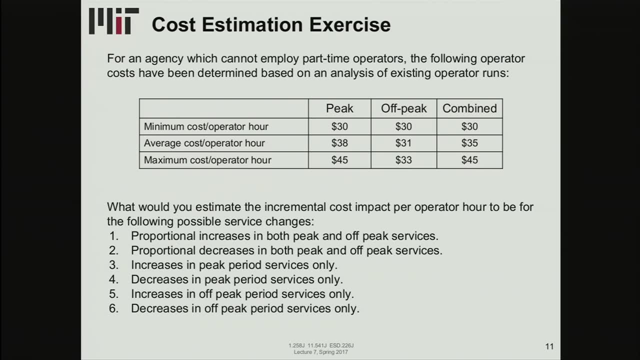 of spread penalties and therefore the same average costs. But now we go to the next question, which is increases in peak period services only. Which of these would you use? Max GABRIEL SANCHEZ- We're hearing max, and I assume for peak? 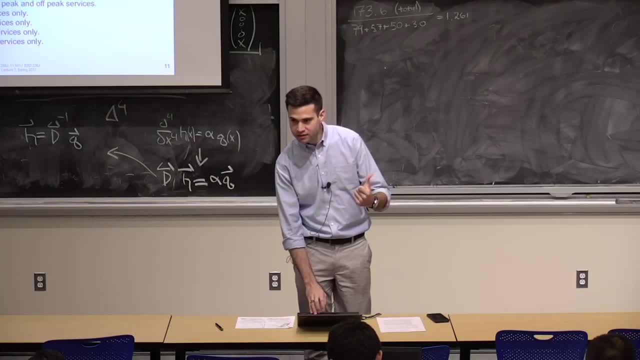 Max for peak, Yeah. GABRIEL SANCHEZ- Any other ideas? Peak average: GABRIEL SANCHEZ- Peak average: Two ideas. GABRIEL SANCHEZ- OK, what's the bait? 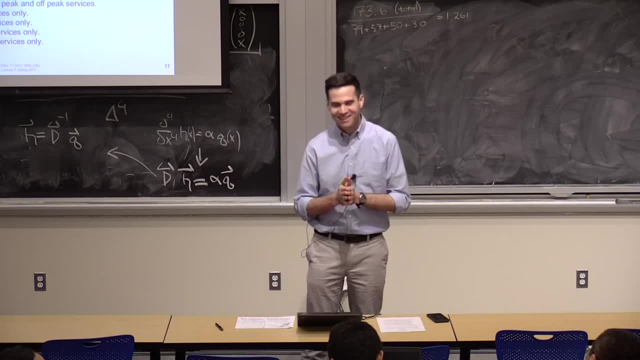 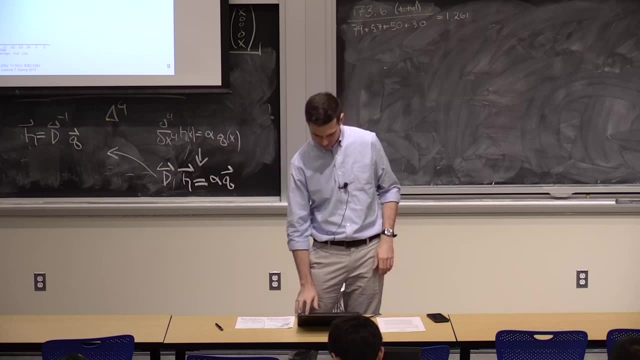 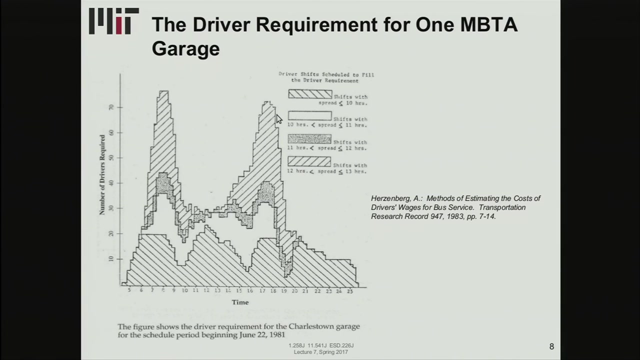 GABRIEL SANCHEZ- OK, That's good, All right. so basically, if we're increasing in the peak period, only we're going to have to do more of these spread shifts to do that, And those are our most expensive shifts. 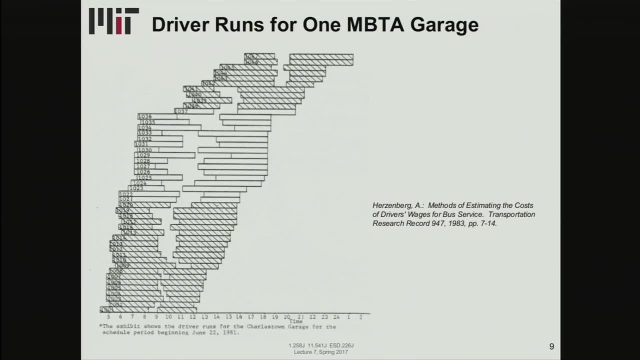 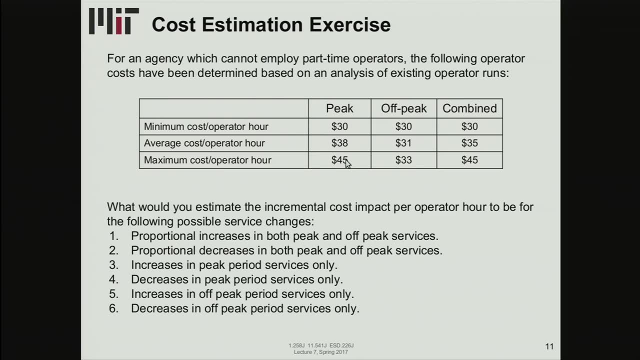 GABRIEL SANCHEZ- Yes, Are you convinced, Convinced? GABRIEL SANCHEZ- OK, good, So great. So $45, right, The maximum of the peak. What if it's a decrease in peak period service? 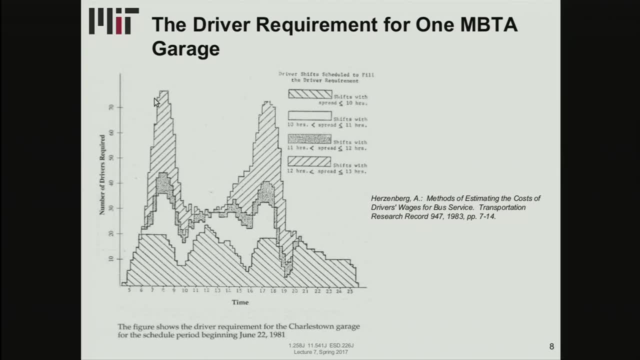 So now we're coming back here and we're only taking the top, of the top off, And we're not going to do that. GABRIEL SANCHEZ- Yeah, We're not doing anything to the off-peak. 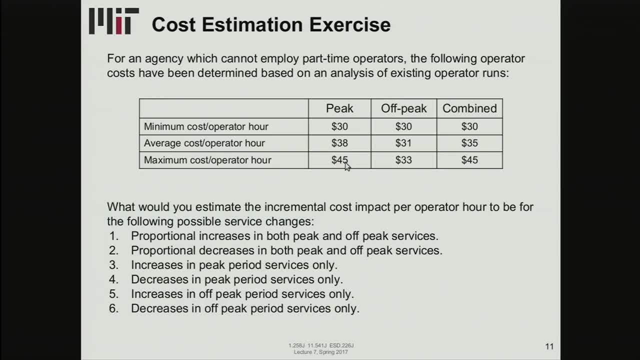 I like the name. The inverse, GABRIEL SANCHEZ- Same 45 going down now, right, OK, great. OK. increases in off-peak period services only. So now we're leaving the peak where it is. 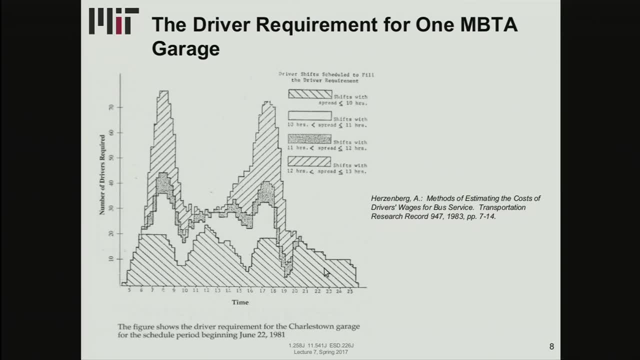 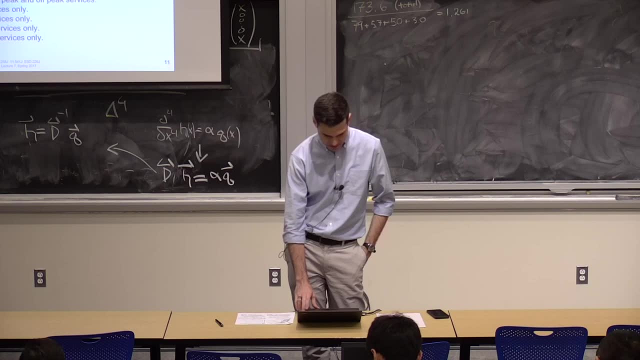 and we're decreasing service, off-peak, So here, and maybe at night, Decreasing. so GABRIEL SANCHEZ- Decreasing- Is it decreasing or increasing? Increasing? GABRIEL SANCHEZ- Let's start with increasing. yeah. 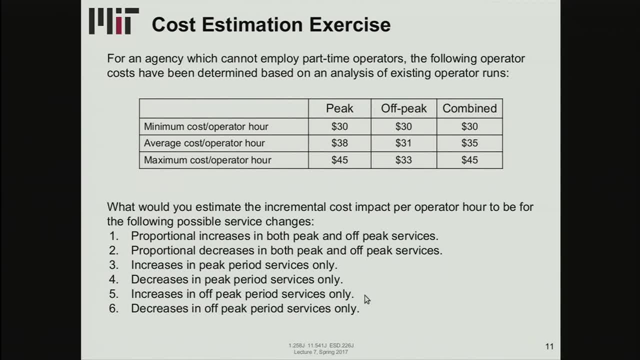 OK, OK, GABRIEL SANCHEZ- Then maybe minimum in off-peak. Yeah, GABRIEL SANCHEZ- OK, That's actually the high end of what it could be. So off of the cells here. yes, that's the one. 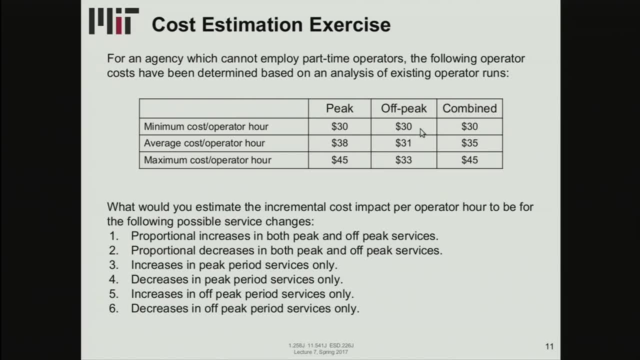 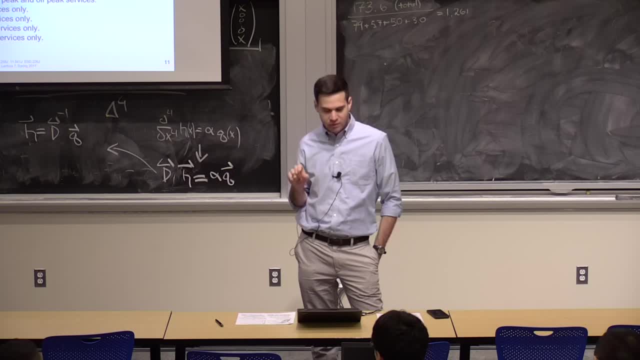 that you should pick. You should use the minimum off-peak, But it could actually be closer to zero. If you're depending on the cost structure and the spread penalties, you will be able to convert some of the drivers that are peak to non-spread shifts. 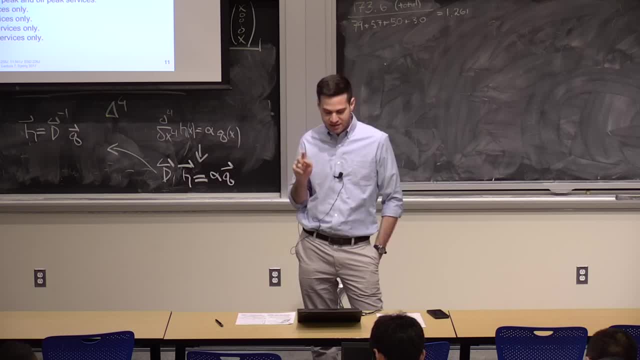 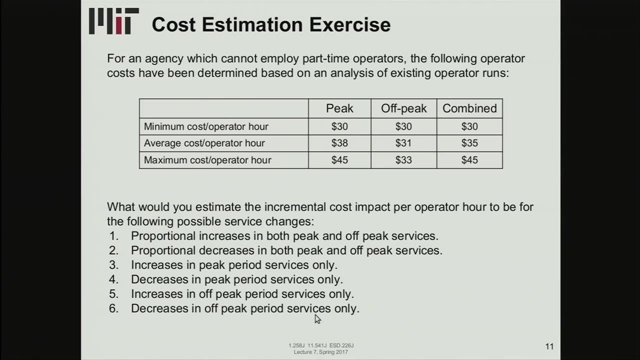 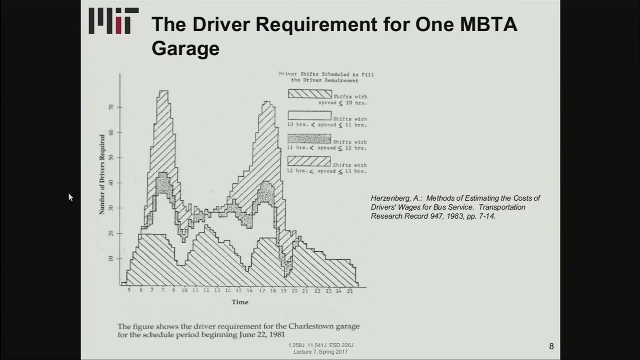 So you'll get straight shifts from these drivers And that may actually compensate so much that it's a free conversion. So what about decreases in off-peak period service? GABRIEL SANCHEZ- OK, GABRIEL SANCHEZ- So now we are actually decreasing. 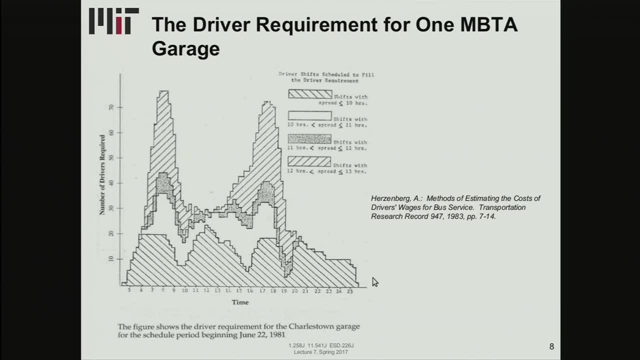 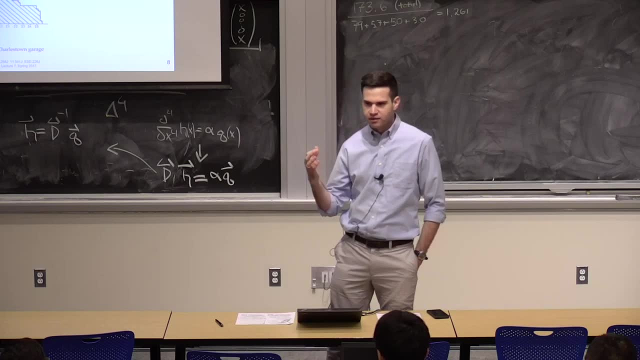 the off-peak and doing everything the same Toward. GABRIEL SANCHEZ- Well, two things happen. Presumably. off-peak services are straight, runs, right, They're not spread. So if you remove those but keep the peak-level operation, 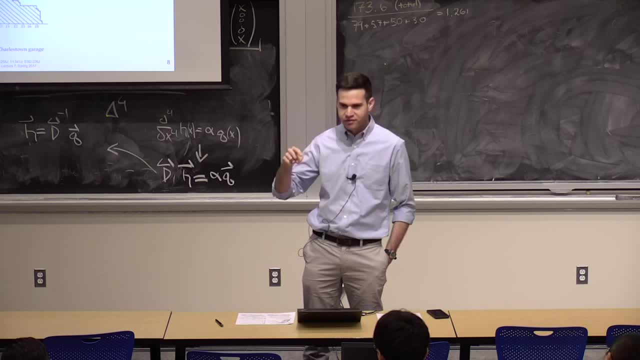 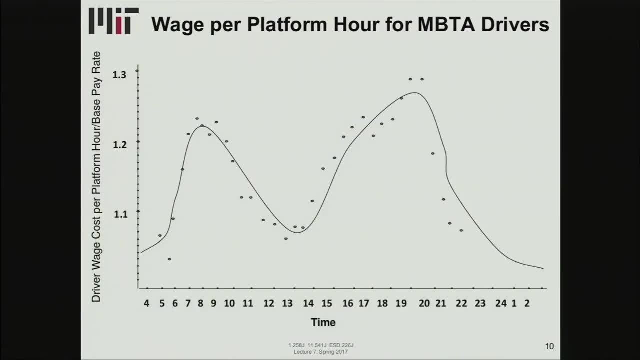 the same, then, for any of those that you remove, you have to add in the most expensive ones. OK, So what was the net effect? Maybe 15 bucks, GABRIEL SANCHEZ- It's probably going to be close to zero. 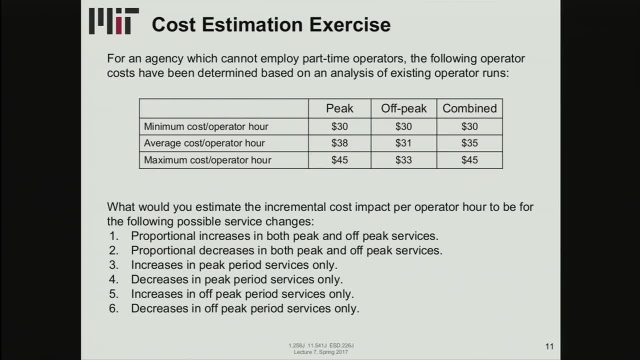 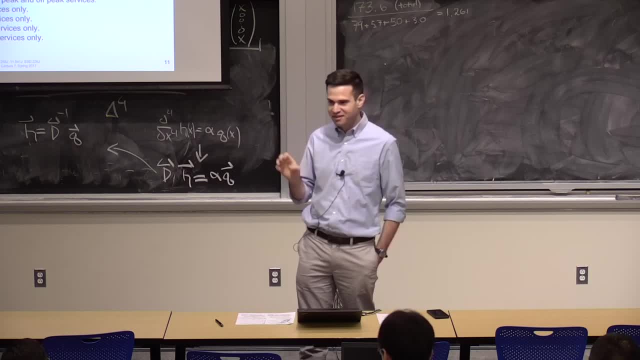 again because of this effect. OK, GABRIEL SANCHEZ- But can you explain why? GABRIEL SANCHEZ- And again, this depends on the specific costs for the labor agreement and the spread penalties and everything. But it gives you an idea. So if you only decrease off-peak service, then you have to remove a few of the straight runs and not pay them the full day, But you have to then get, you have to convert some of the existing spread runs to excuse me. 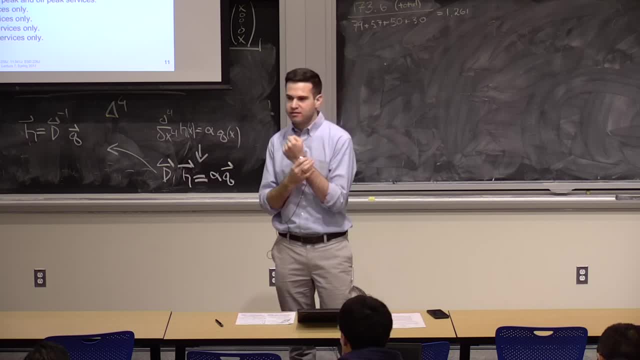 straight, GABRIEL SANCHEZ- To from straight to: yeah, Yeah, GABRIEL SANCHEZ- To the spread: yeah, So why is it in that cost of zero? then, GABRIEL SANCHEZ- Because you. even though you are reducing the number of driver hours, you will increase the proportion of the most expensive ones only in the peak, So you might not wind up saving any money. GABRIEL SANCHEZ- Exactly Where would you put it in the matrix? 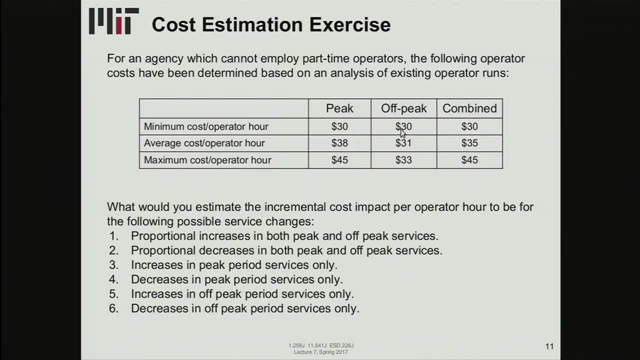 GABRIEL SANCHEZ- Well, it's not in the matrix But if anything, you would look at off-peak minimum, But it's going to be in the range of 0 to 30. And again, depending. 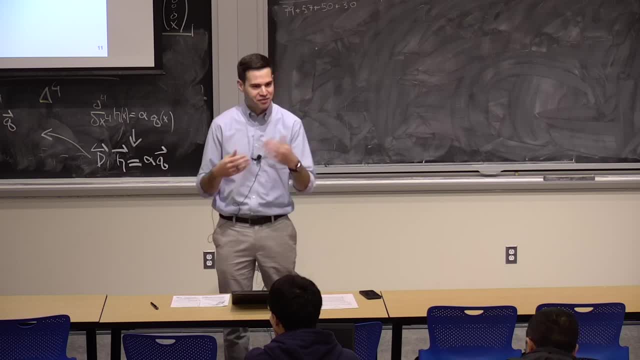 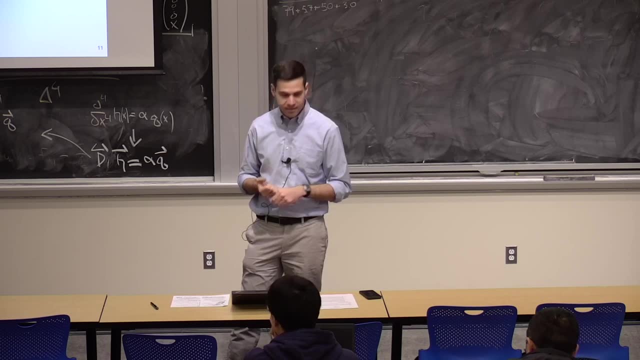 on the specific numbers. it could even be that you have to pay more or many things can happen. You're saying that it was going to be like the off-peak minimum and the peak maximum? GABRIEL SANCHEZ- Yeah, it could be. 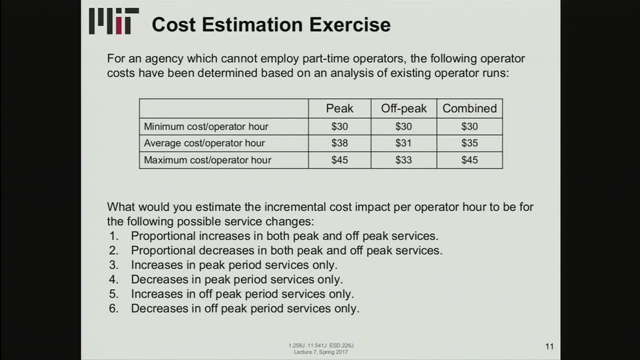 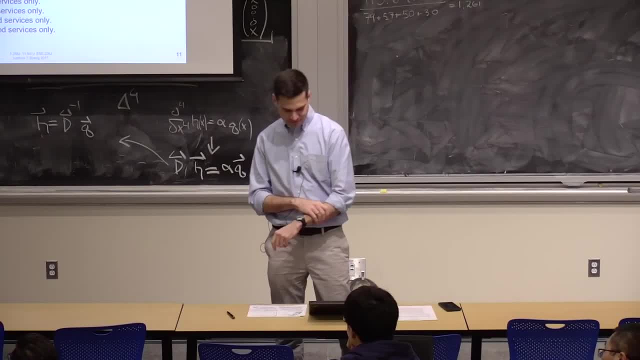 That's a good idea. So, but again, it depends on the specifics And this is a cost model that isn't so precise, You're saying, because you're not actually increasing peak service, but you're proportionally increasing it. GABRIEL SANCHEZ- Not proportionally. 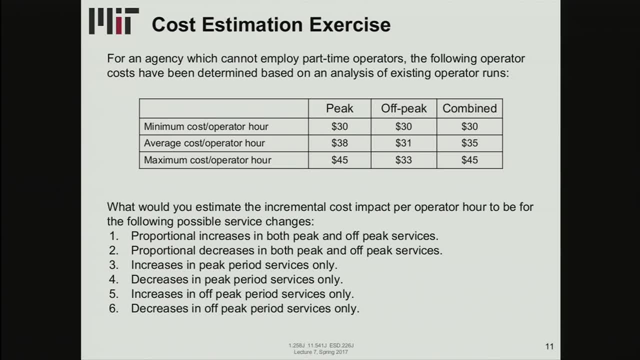 We're just decreasing the peak and not touching the peak. GABRIEL SANCHEZ- But then it's proportionally more of your hours of peak. Yes, exactly, That's why it's going to be more expensive. GABRIEL SANCHEZ- Exactly, yeah. 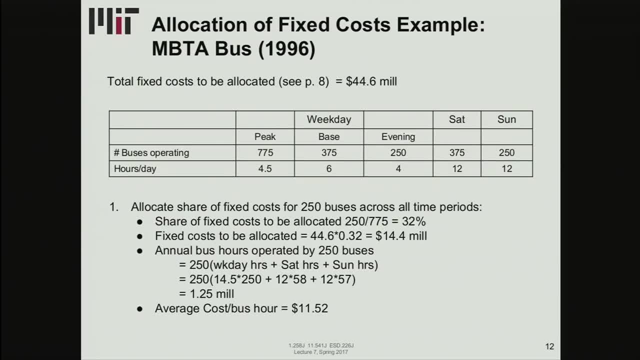 All right, Watch this out, GABRIEL SANCHEZ- So that was good. There's a mistake in this slide. Please fix it. It says here: see page 8.. It should be see page 6.. So from page 6, the total fixed cost to be allocated. 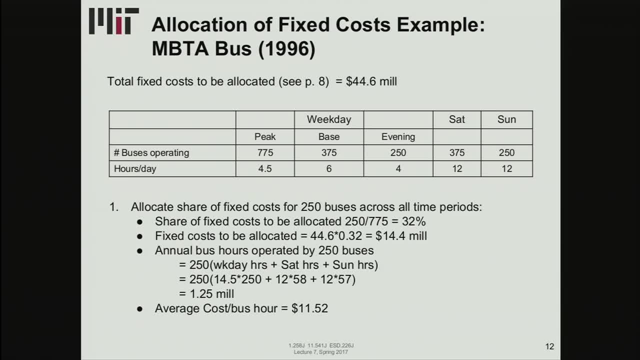 is $44.6 million- Right So, GABRIEL SANCHEZ- And that is the sum of where we want to allocate fixed costs. So that is the sum of all the fixed costs that appear on page 6, which is 5.7,, 3, and 35.9.. 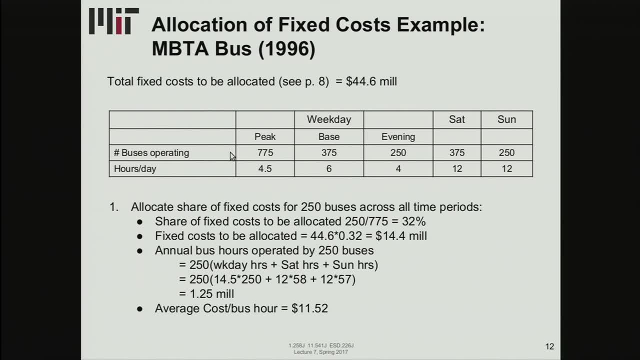 That adds up to 44.6.. And now we have here number of buses operating on the peak, on the base, on the evening, Saturday and Sunday. the number of hours So: peak hours: 4.5, six base hours, four evening hours. 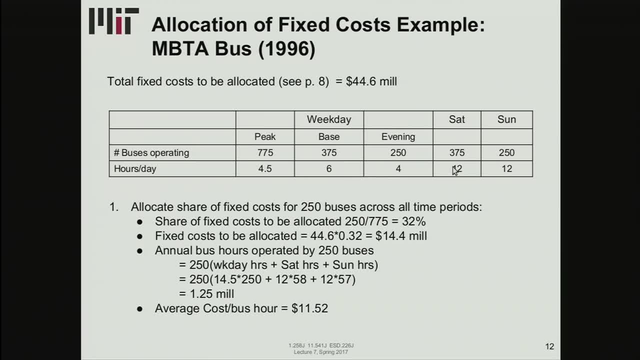 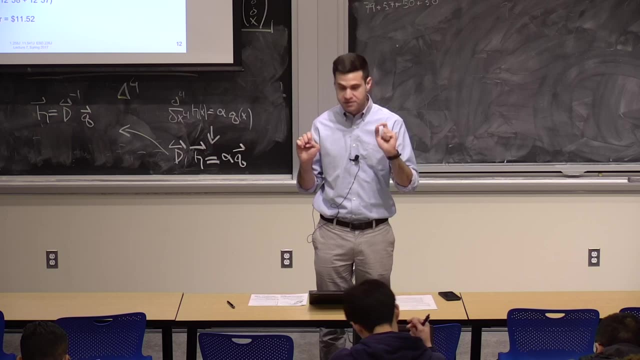 for a total of 14.5 hours per week For a weekday, 12 hours operating Saturday, 12 hours operating Sunday. And the objective of this model is to take the fixed costs incurred by the agency and allocate them to vehicle hours. 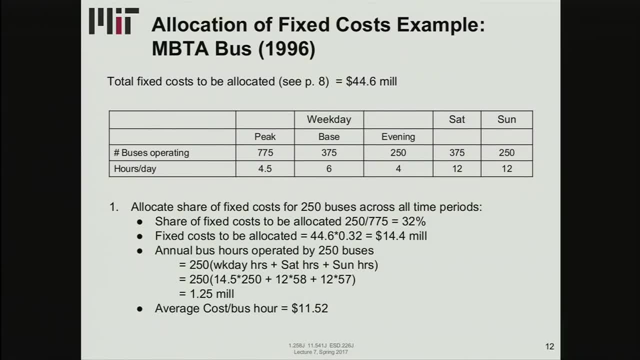 Right. So let's do that. We have to do this allocation, And we can start with. one way of looking at this is these evening buses: 250 evening buses are also operating in the base and in the peak right. Then there's an additional 125 buses. 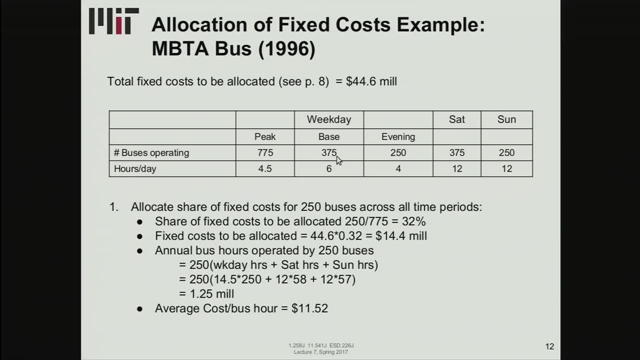 that are operating only in the base during Saturdays, right. And then there's an additional 400 buses that are operating only in the peak during the weekday. OK, So let's allocate costs to the 250,, the additional 125, and the additional 400 according to how long they operate. 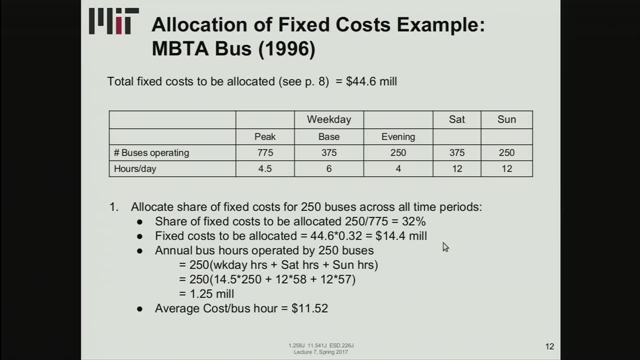 and how much it costs, based on the unit costs that we calculated in this example. So we start with 250 buses across all time periods. What's the share of fixed costs to be allocated to them? It's 32%. It's 250 buses divided by the total number of buses. 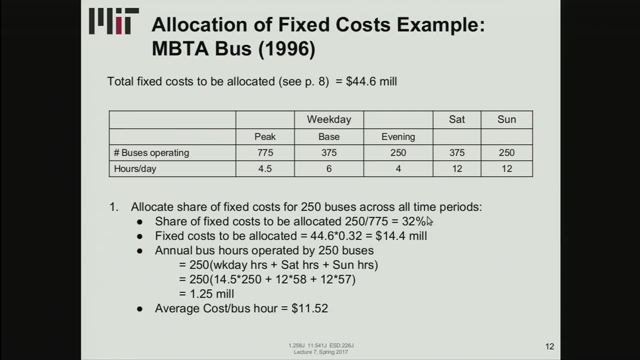 which is 775.. That's 32%. 32% of the total cost is 14.4 million. That's how much money we want to allocate to these buses And how many bus hours are operated in the whole year. Well, there's 250 buses. And we want to add up the hours operated during weekdays, during Saturdays and during Sundays, for the whole week. So there are roughly 250 weekdays in a year, 58 Saturdays and 57 Sundays. Those add up to 365 days And there are 14.5 hours during the weekday. 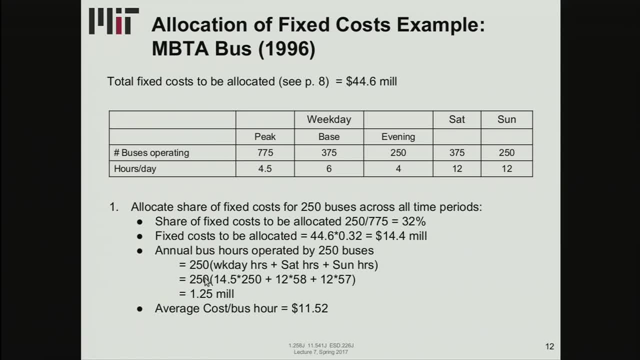 and 12 on the weekends. So we add those up, We multiply by the number of buses and we get 1.25.. 1.25 million bus hours for the whole year. And if we divide the $14.4 million by 1.25 million bus, 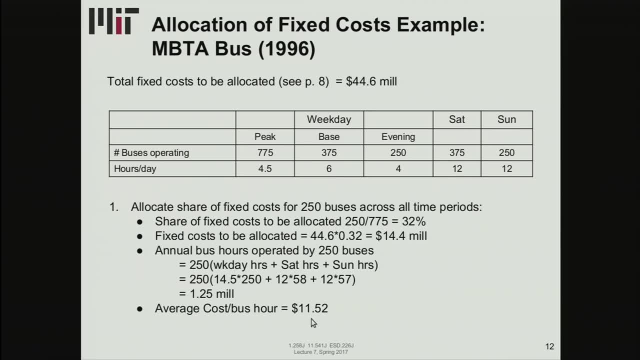 hours, we get an average cost per bus hour of $11.52.. And that's the base, which is the only thing that applies in the evening and Sundays, And it is a portion of what applies in Saturday, weekday days and peak, but only a portion. 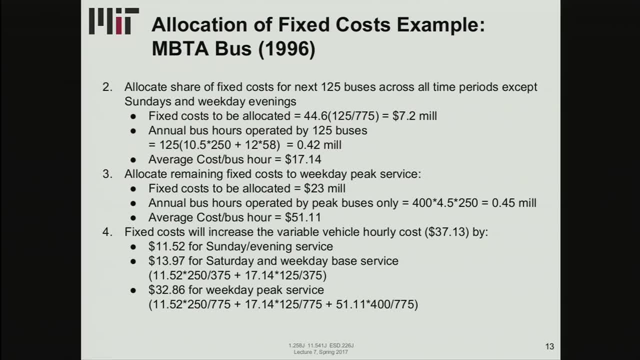 So now let's move To the next 125 buses operating on all time periods except Sundays and weekday evenings. So how much money do we have to allocate? The $44.6 million total divided by the additional 125 buses, divided by the total number of buses, that's $7.2 million. 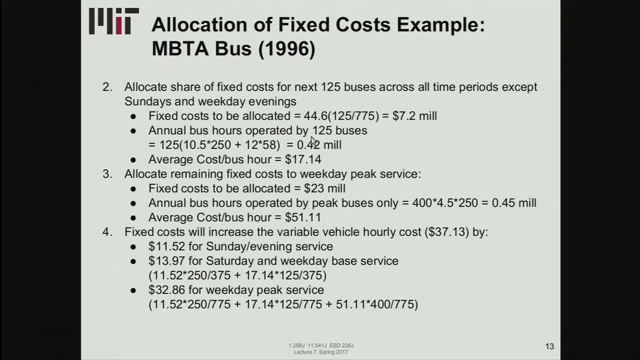 How many total bus hours are operated by those 125 buses? Well, it's the 10.5 hours Excluding the evening during the weekdays times- 250 weekdays, plus the 12 hours on Saturdays times, the 58 Saturdays. So that's 0.42 million bus hours. 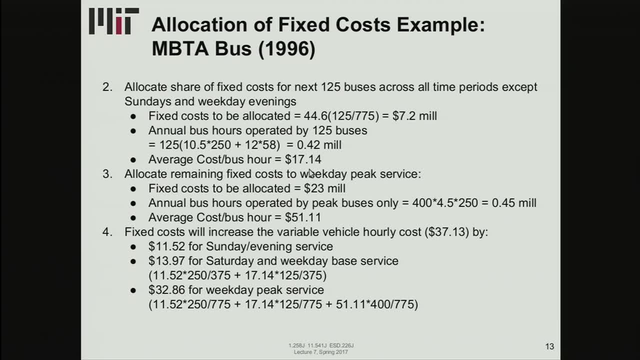 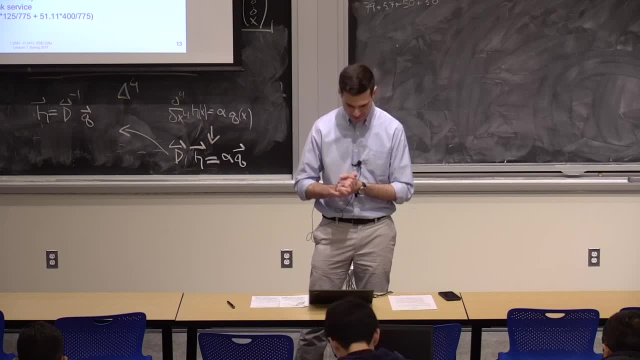 And 7.2 divided by 0.42 is $17.14. average cost per bus hour. Do you follow Any questions on this? OK, now let's do the peak. That's the most expensive part. So how much do we have to allocate? 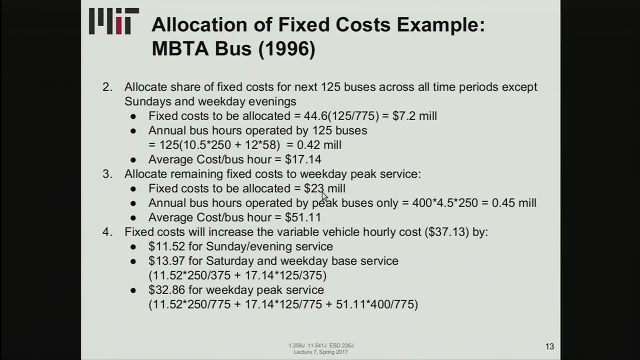 It's $23 million. How do we get that? 44.6 total times 400 divided by 7.25.. And how many annual bus hours do we operate during the peak? It's 400 additional buses only in the peak times, 4.5 hours. of the peak times, 250 weekdays And that's 0.45 million hours and 23 million by 0.45.. It's $51.11, average cost per bus hour or per peak bus hour in this case. So now we have unit costs for peak the base. 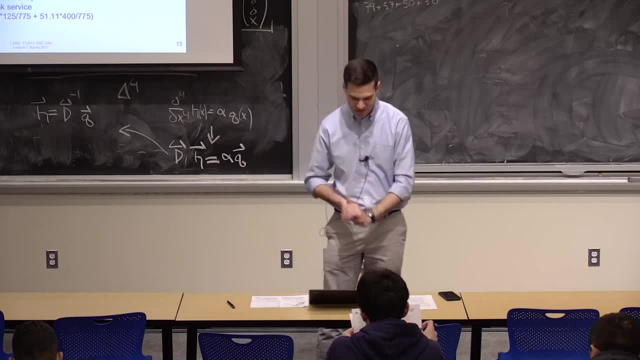 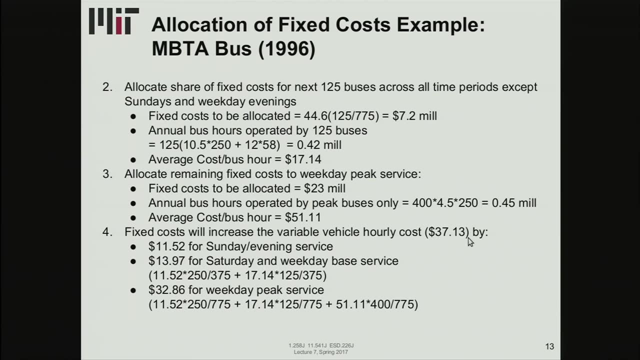 and then the off peak, the evenings and Sundays operation, which is great. So the variable vehicle cost was 37.13.. We had calculated that from the previous model that you can find on page 6.. OK, And now we can adjust these costs. 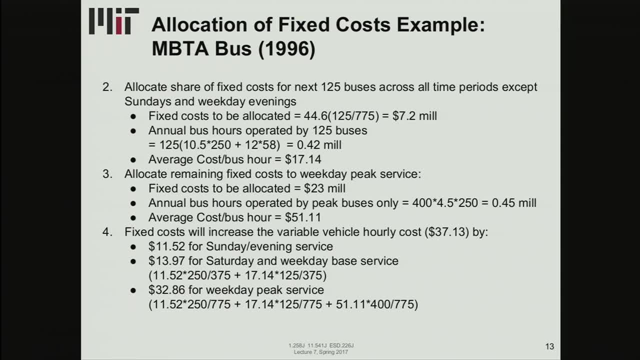 by time period, which is what we want to do. We want to have a model that is sensitive to time periods. So for Sunday evening service, we will increase the $37.13 by $11.52.. For Saturday and weekday service: 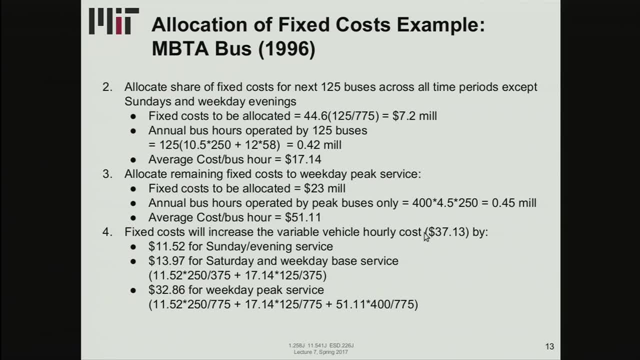 we want to increase the cost- the base cost of 37.13- by $13.97.. And for weekday peak we want to increase the base cost by $32.86.. And notice that when we look at Saturday and weekday, we have to combine the two unit costs that we calculated. We have a portion of Saturday and weekday base service is from the first 375 buses And the portion of it is from the additional, more expensive 125 buses, And when we do peak, the same thing applies. So we start with the 250 base bus. 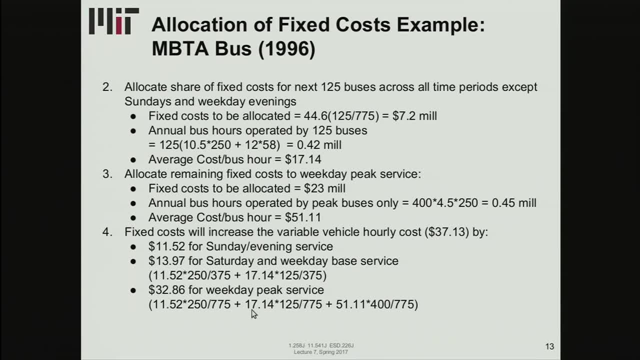 We add the buses at $11.52.. Then we add 125 at $17.14. And then we have the peak of the peak buses, which are 400 times the unit cost for those buses, which is much higher. And that's the total cost, the total unit cost. 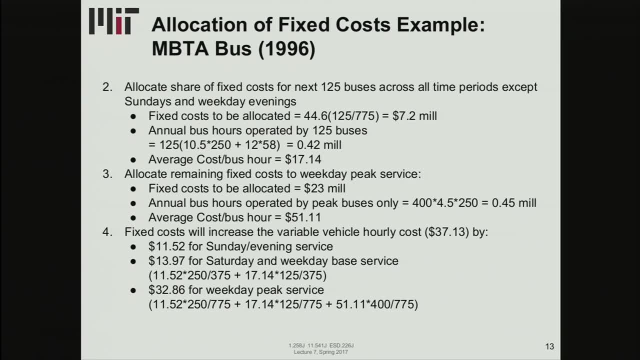 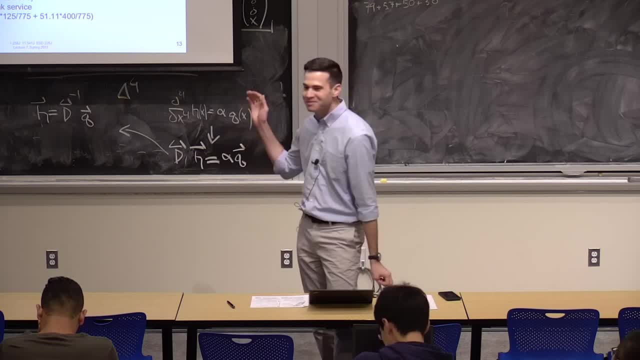 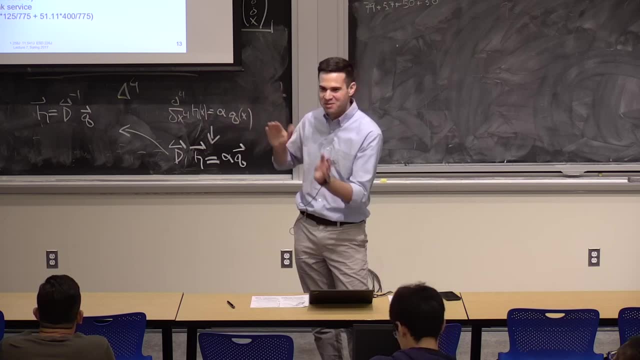 for a weekly peak service. OK, Questions on this. You have a question, Eli? OK, This is all sort of written here And all the numbers are copied from from previous slides, So you should be able to follow this on your own. 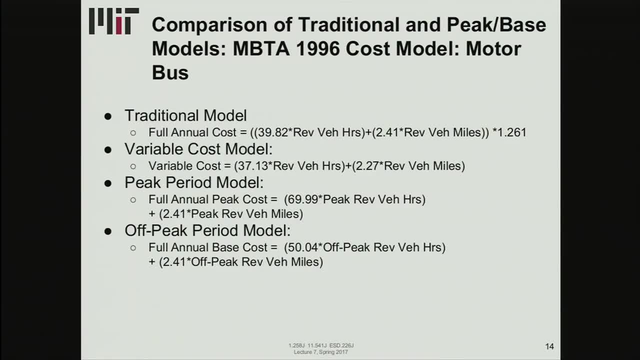 if you're a little lost, But if not, come see me after class and we can talk about it. OK, so now let's compare the models. We started out with a very traditional, simple model And the first one we gave, which was full annual cost. 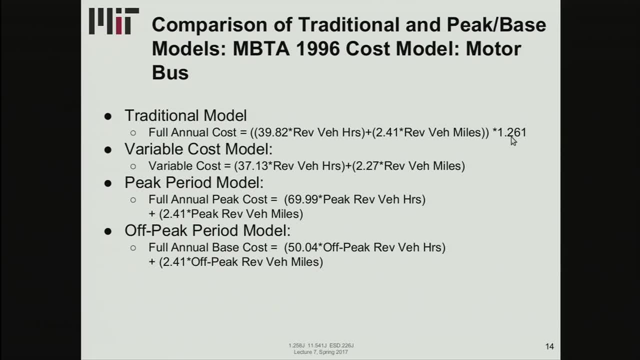 and it had this factor which accounted for the fact that we weren't including the peak vehicle, the costs associated with peak vehicles. So that was the first example. So we also had in that page a variable cost model which only accounts for variable costs. 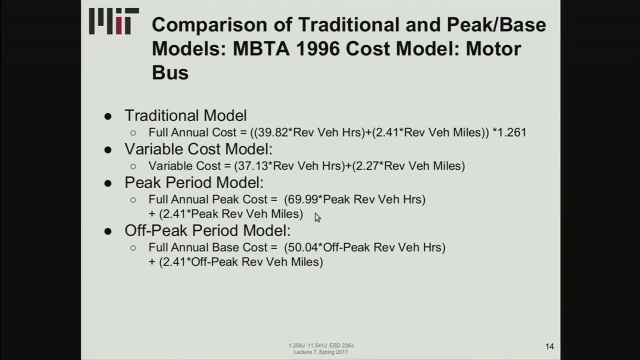 so it excludes fixed costs. And now we can look at the peak period model and the off-peak period model. So we make an adjustment to the first model, which to this variable cost model, with the unit cost that we just calculated. 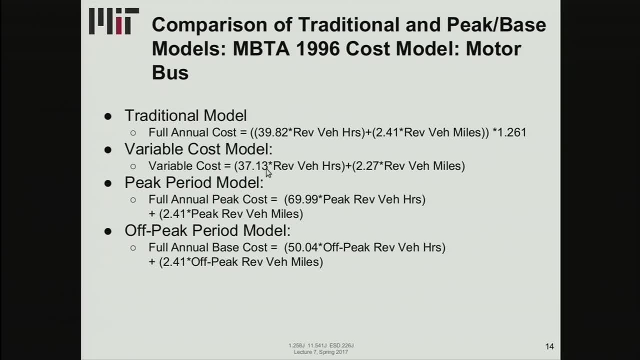 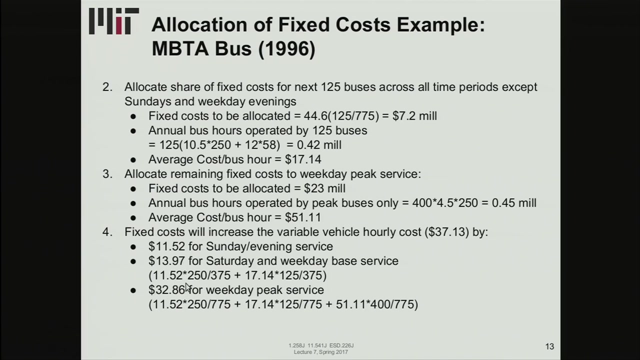 So So if we take the $37.13 of revenue vehicle hours that was in our initial variable cost model and we add the unit cost for peak revenue hours, which is $32.86 from right here, so that's the weekday peak service. 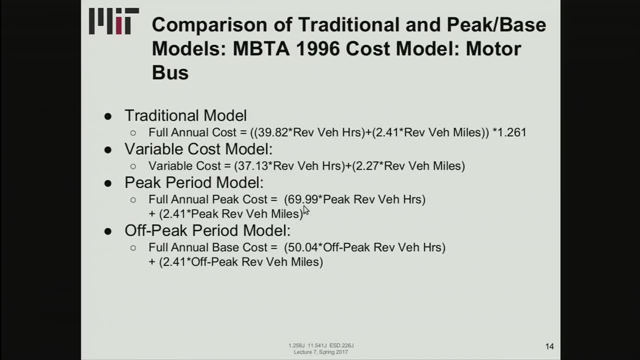 unit cost, then we get $69.99.. So now that becomes our unit cost in the week And we add the $2.41.. $2.41, let me give me a second here. That comes from page 6 directly, I believe. 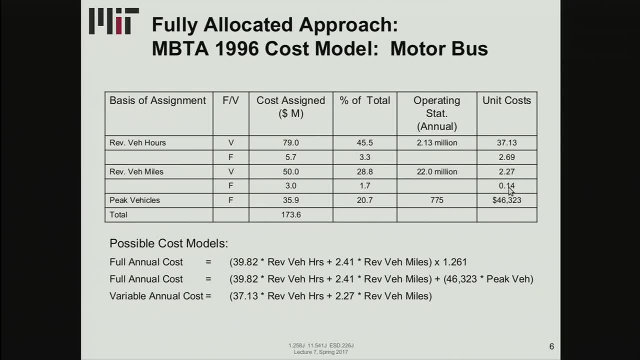 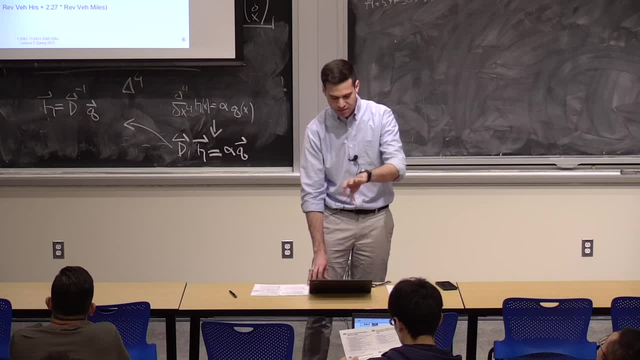 Yes, So that's the combination of $2.27 and $0.14, because we're not counting the total time. We're only doing the temporal difference on peak vehicle or revenue vehicle miles. We're only doing it for revenue vehicle hours. 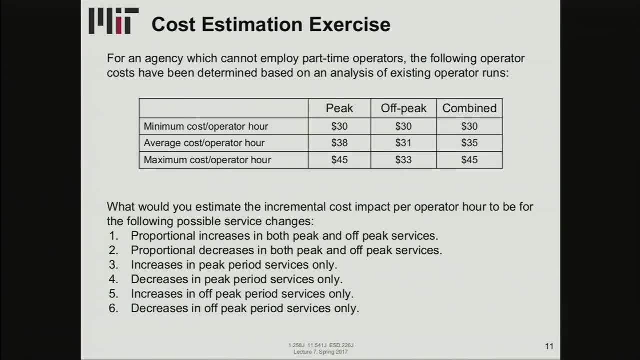 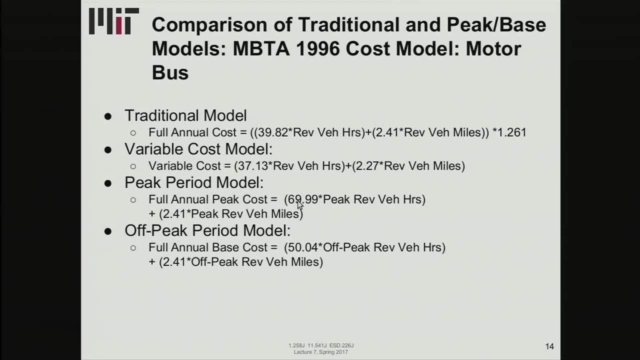 It's for driver costs, and driver costs were associated with hours, not miles, So that stays the same. So this is our full annual peak cost model And if we want to increase peak-only service, we use this model, not the other one. 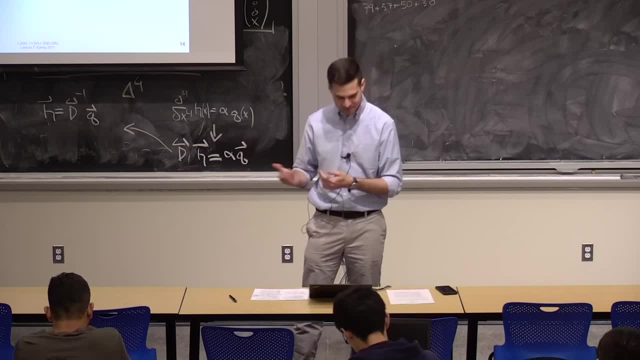 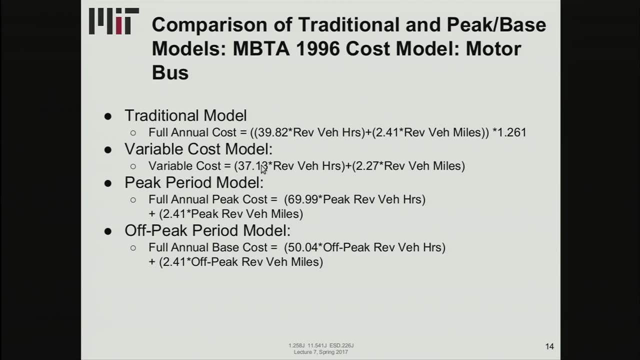 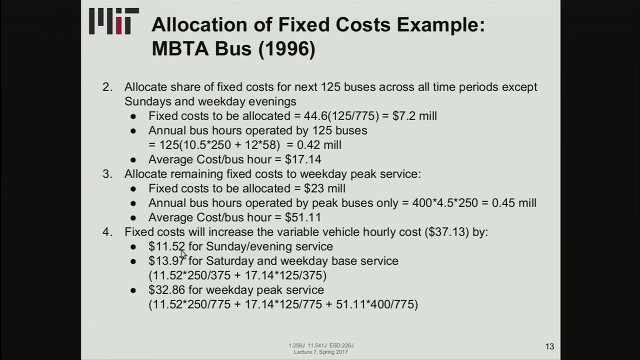 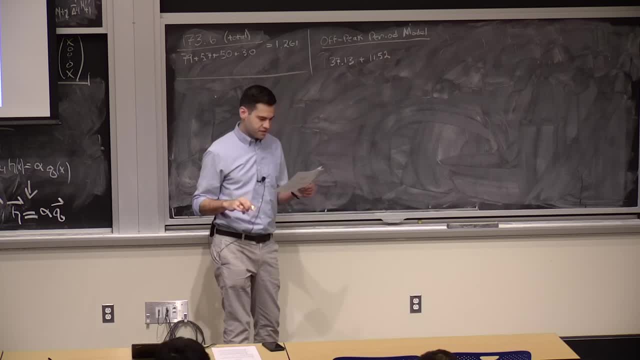 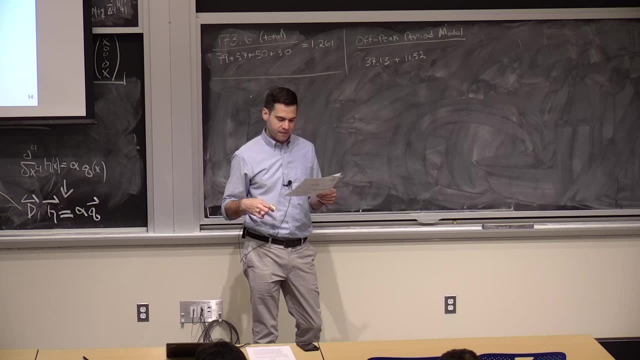 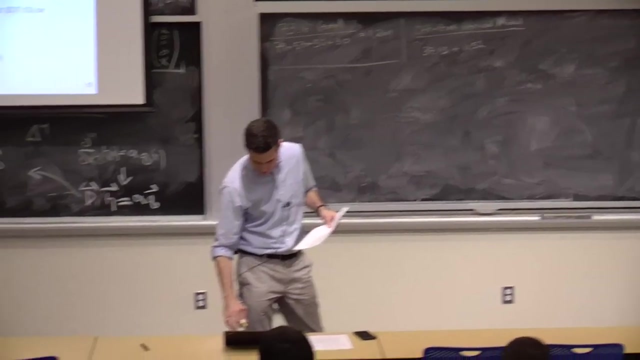 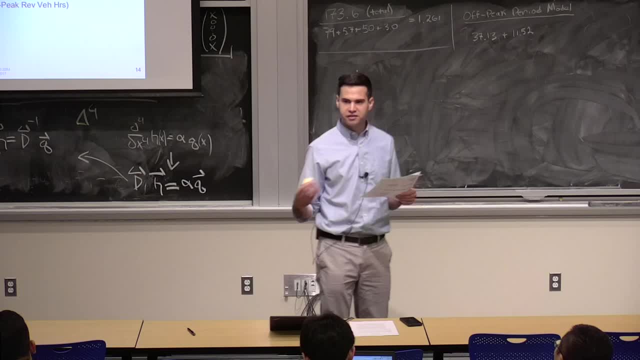 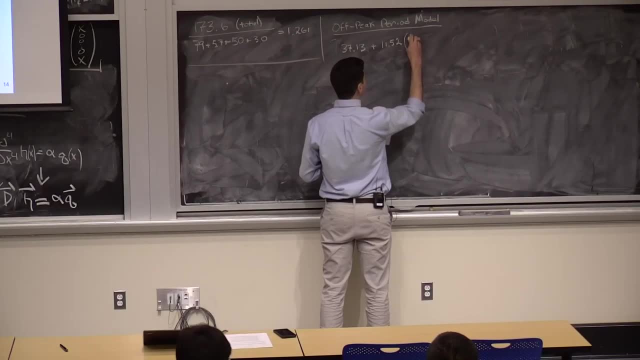 only So. the question is, how many Sunday and evening service hours are there in the whole year? Well, the proportion is this one that I'm writing down: It's $11.52.. This one that I'm writing here: $16.84 divided by $3,880.. 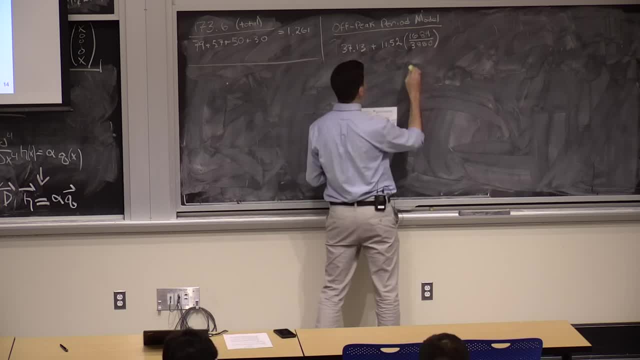 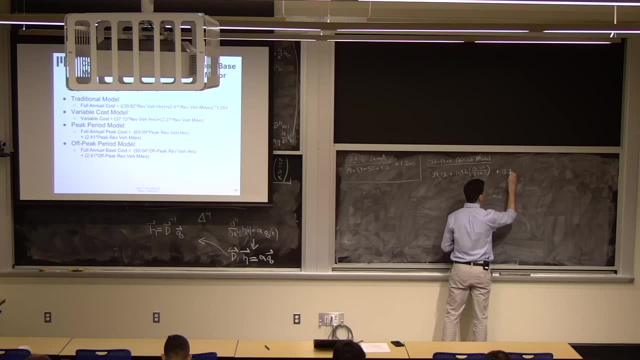 And I'll calculate that too in a second. We also want to add the other cost, which is $13.97.. And the proportion of that is 2196.. And the proportion of that is 2196.. nine six divided by three thousand eight hundred and eighty. 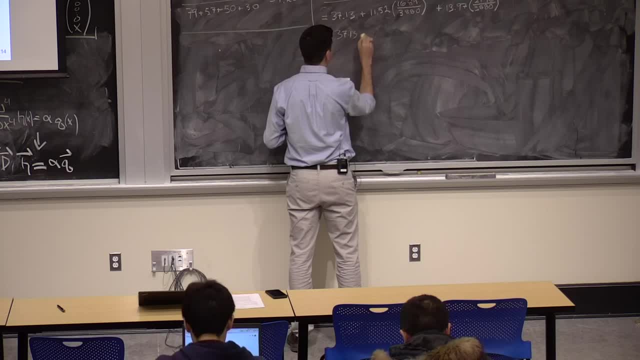 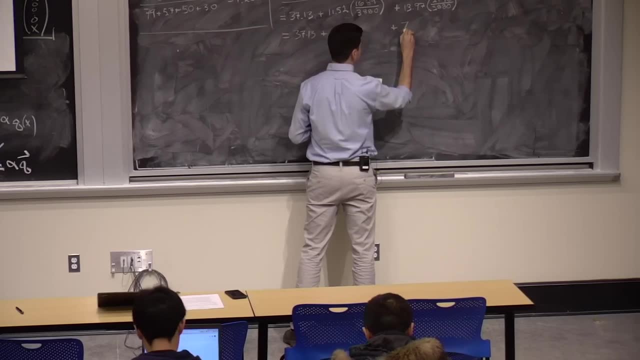 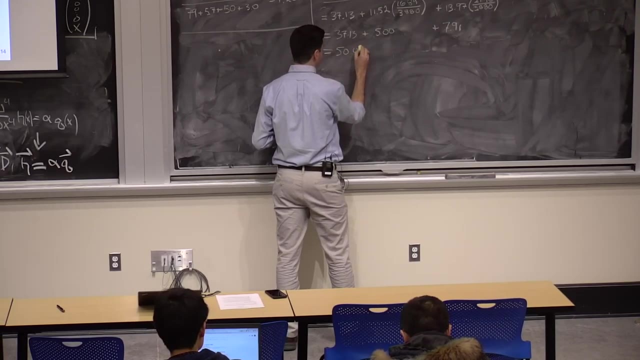 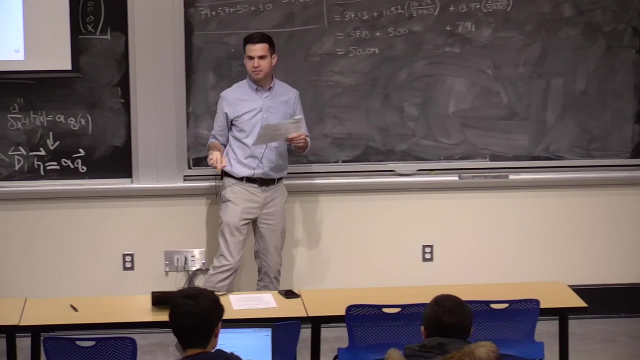 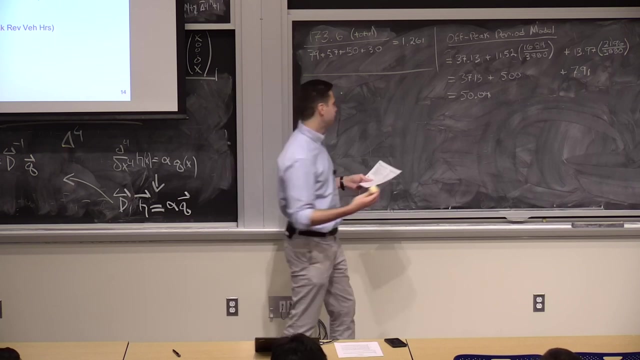 So that's 3713 plus about five plus about 791, and that comes out to 5004.. Okay, so where do we get 1684 and 1296 from? It's similar to before. right, We just count how many hours there are, So let's just do it quickly here for. 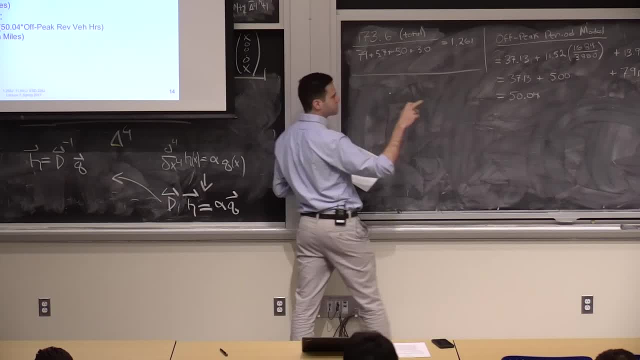 the record. So let's just compute the bottom one, actually, and you'll get the idea for the others, because it salt forever. Alright, so let's do look at scandals. Alright, so let's just do look at scandals. Okay, so let's just do look at scandals. So let's just do look at scandals. 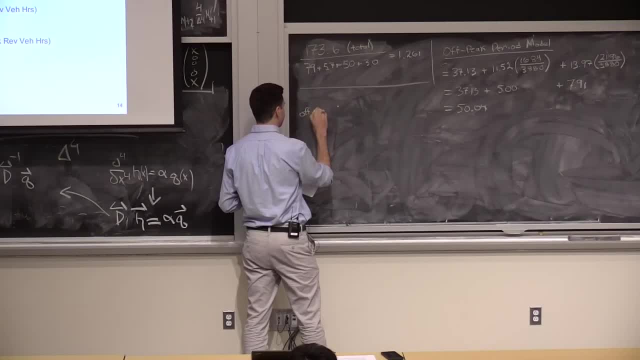 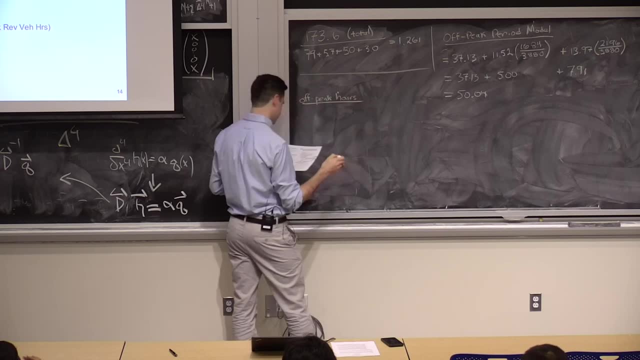 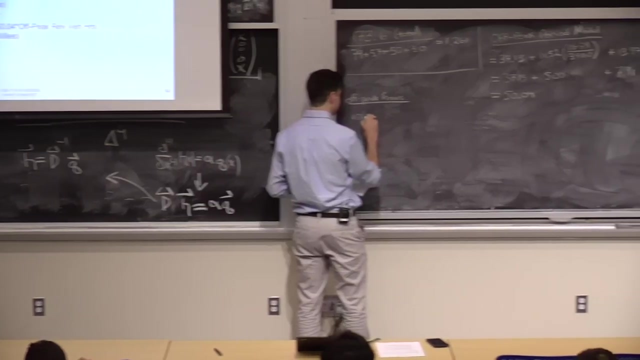 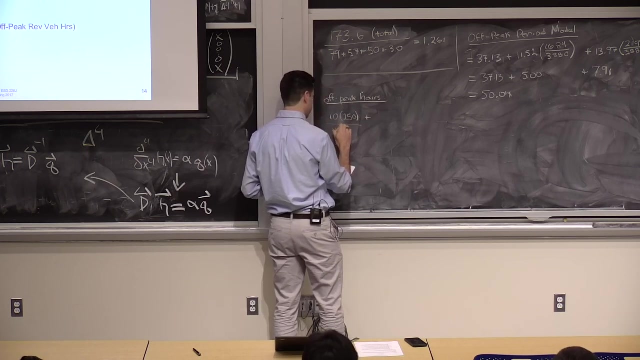 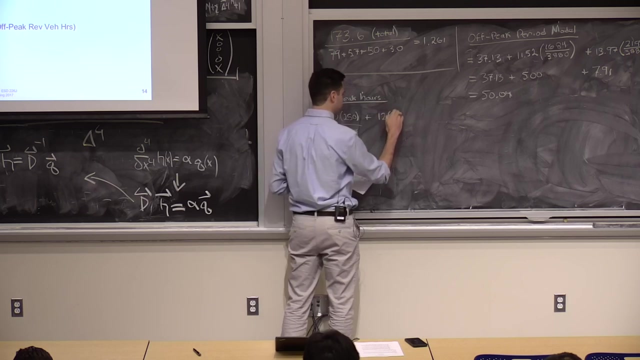 So it doesn't make sense to do all of them. So off-peak hours: So we have 10 off-peak hours in the weekday times, 250 weekdays per year plus. so this is weekdays plus 12 hours on Saturdays, And we said there are 58 Saturdays per year. 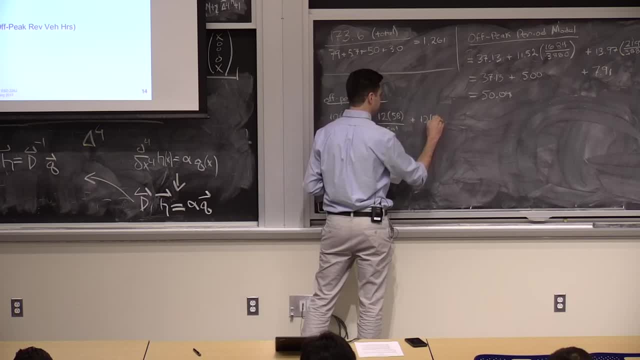 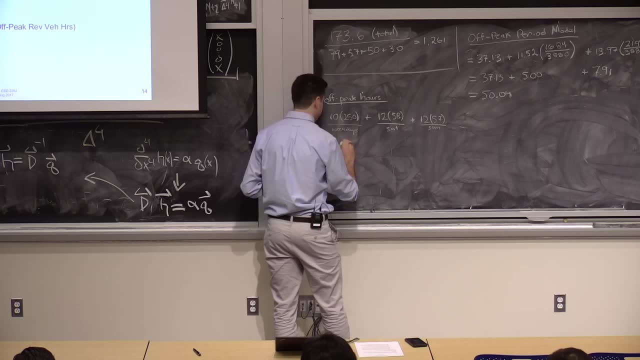 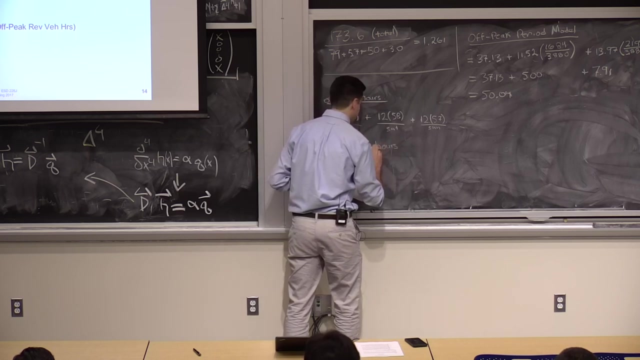 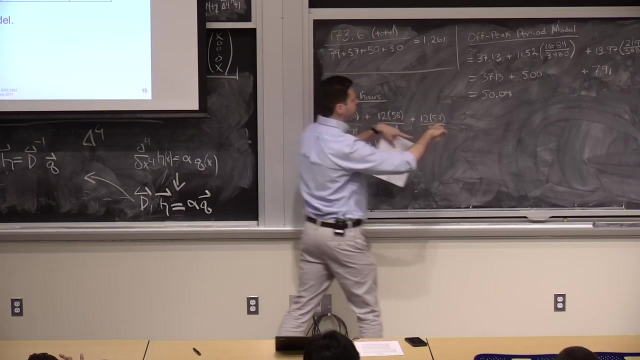 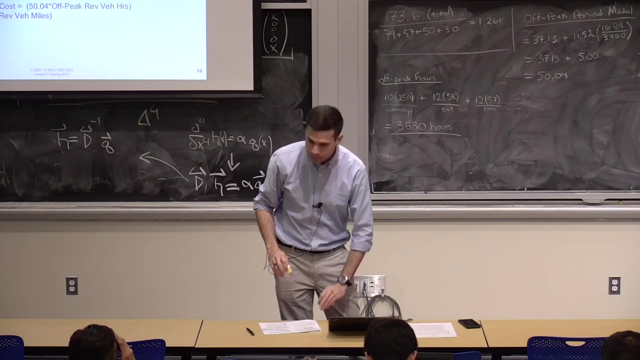 plus 12 hours on Sundays, And we said 57 Sundays per year And that comes out to 3,880 hours And you can select combinations of these to get the 1,684 and the 1,860.. So for the 1,684, that's Sunday evening service, right. 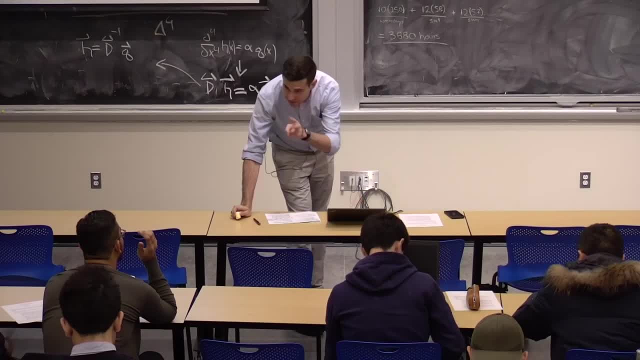 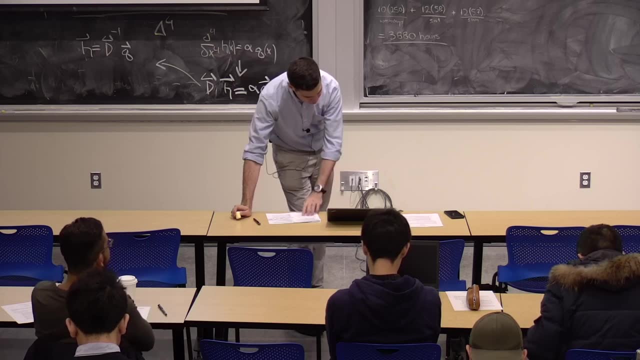 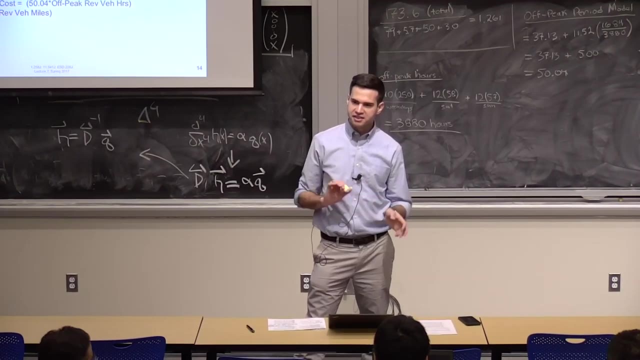 GABRIEL SANCHEZ- Right, so yes, exactly. So that's Sunday and evening, Right, The other is Saturday and weekday, basically. GABRIEL SANCHEZ- Yes, exactly OK. So did people follow this allocation example? 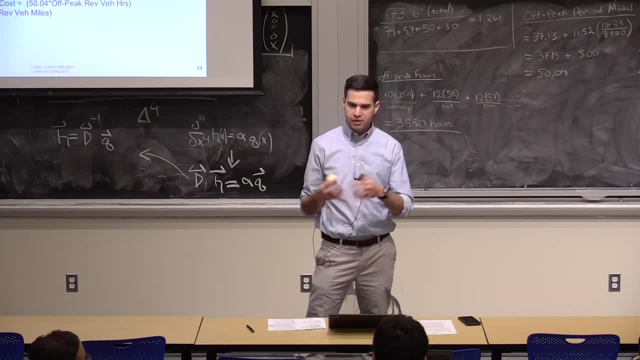 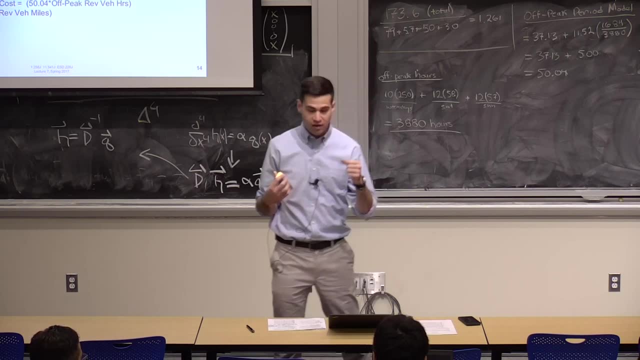 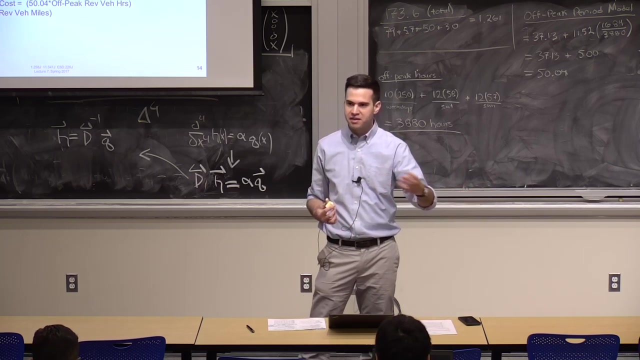 So what we're doing is dividing the day into periods, Some periods we recognize are more expensive than others to run. We take the now. we have fixed costs and we want to allocate them across periods, And we want to allocate more costs to the peak. 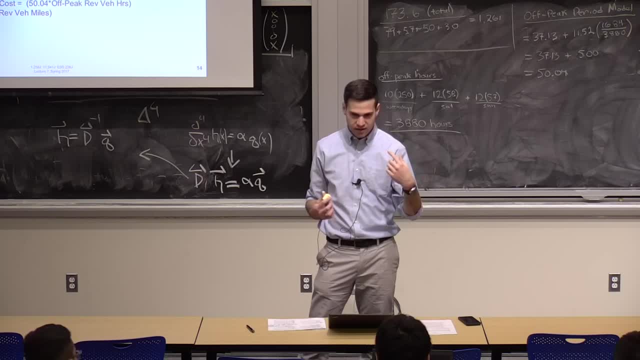 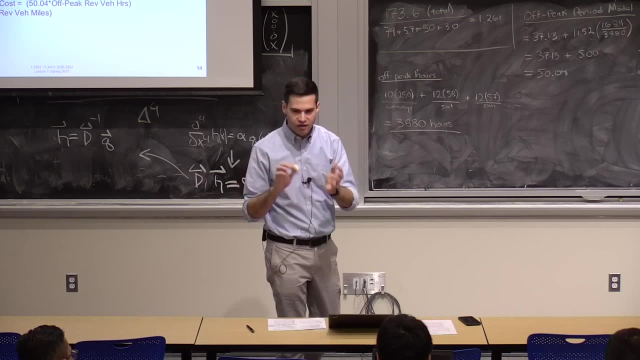 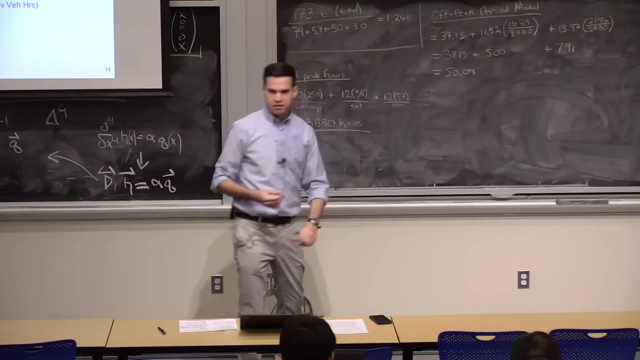 because that sort of costs more. So we then use these unit costs to and we count how many hours we provide off peak and during the peak And we do things in proportion to that. essentially, These are not the only cost models that you can come up with. 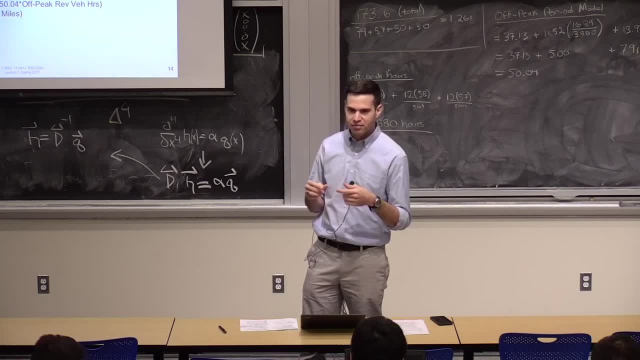 These are not the only ways of allocating costs, But they provide an example of how you can go about allocating costs. Allocating cost is a science. It's also an art, And you encounter it in agencies because you have these huge, huge budgets or huge expenditures. 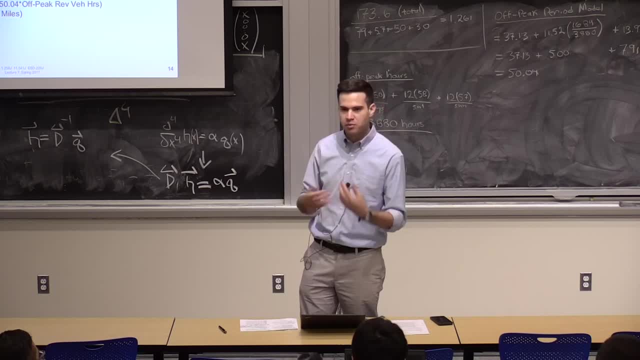 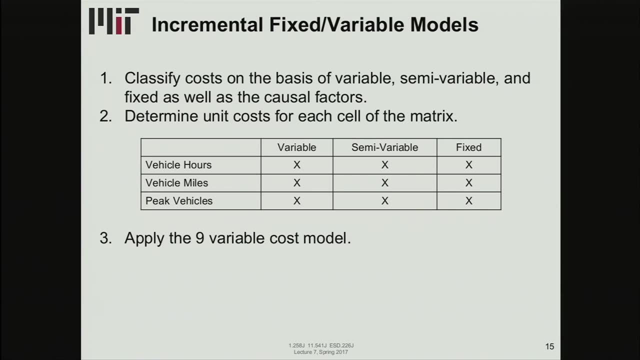 And many projects require you to apportion or allocate costs, And if you want to have a cost model, you have to do it, because your cost model should reflect these different variables. exponential variables: OK, the last, the third and last type of model. 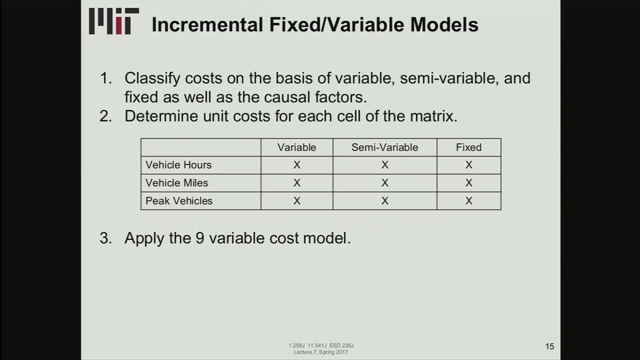 that we want to discuss is the incremental fixed variable model. So here it's somewhat similar to the ones that we saw before. Now we classify costs as being variable, semi-variable and fixed. So we have a little more precision, a little more precision in what we consider fixed or variable. 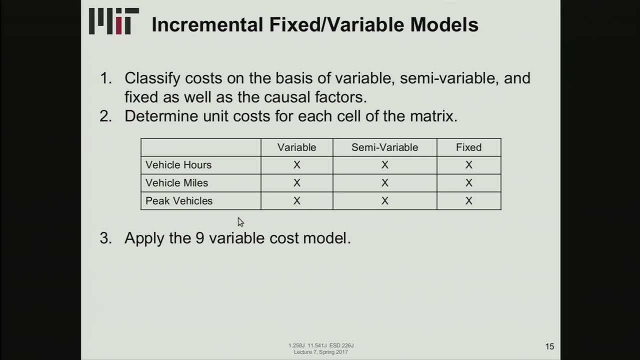 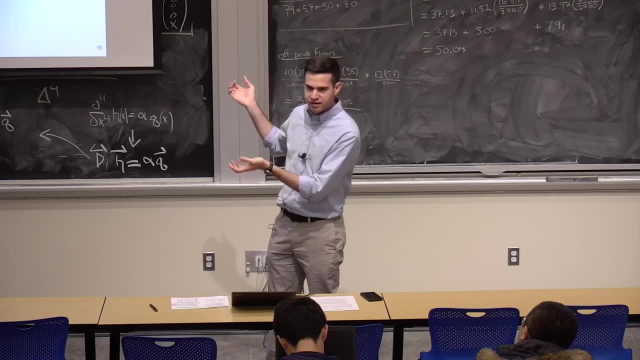 We also have the same explanatory variables that we had before, so vehicle hours, vehicle miles and peak vehicles. So now the combination of these are nine different explanatory variables And we do the same thing as we have done before We go, we have a schedule of expenses. 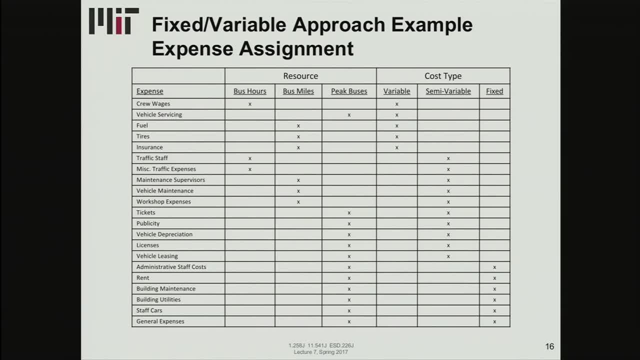 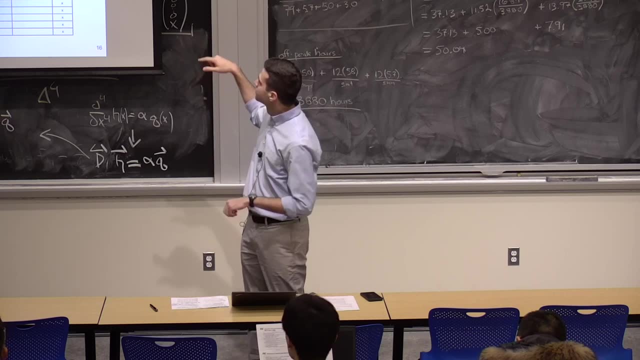 These are accounts in your ledger. So crew wages, vehicle service and fuel, tires insurance, traffic staff, things like publicity and rent and building maintenance- everything is included here. So all of your budget is going to fall into some category is divided among these categories. 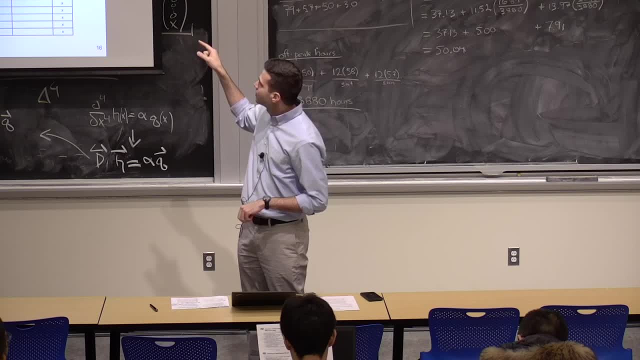 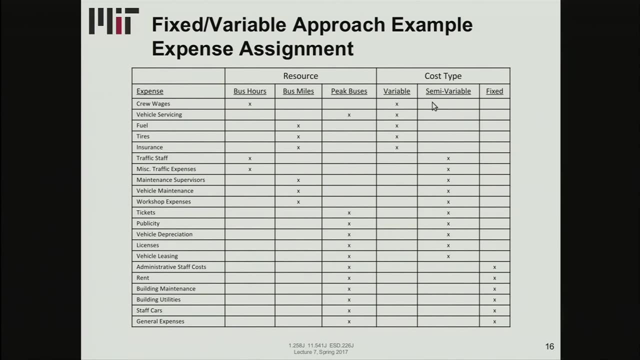 So now you decide for each of these which ones which of these three resources apply and which cost type you consider this to be. So, for example, crew wages: let's associate that with bus hours, as we did before, And that's fully variable. 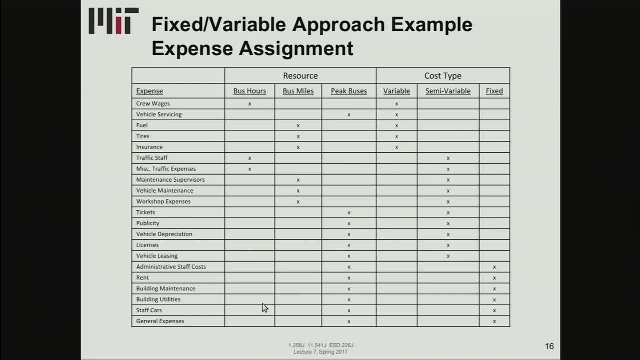 So that we should feel comfortable with Things like building utilities that shouldn't be variable. So that's a fixed cost And we'll associate that with peak buses, because peak buses is the one that we say is a good proxy for how big the agency is. 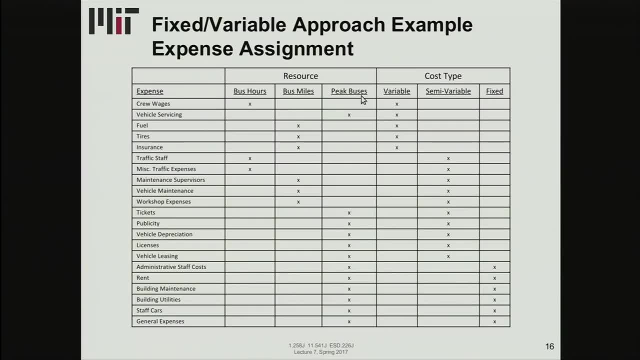 So peak buses is again like agency size, if you will. So then there are things in the middle. So publicity, well, semi-variable, because to the extent that you increase service there's going to be some amount of additional publicity. 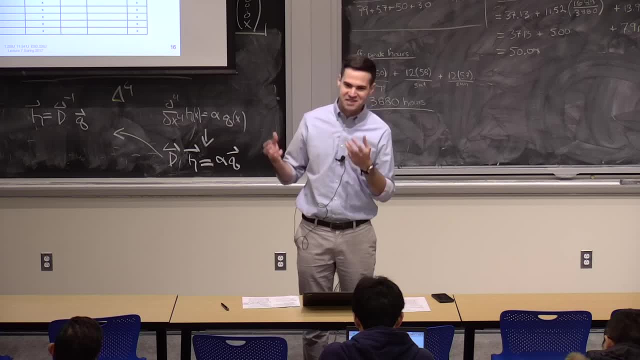 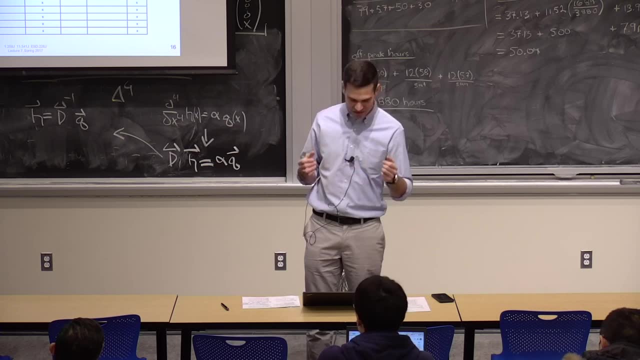 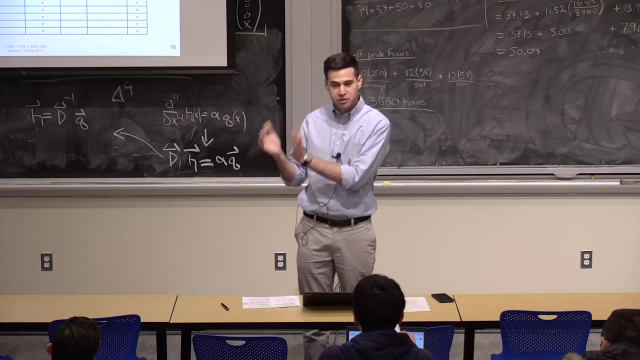 There's not going to be necessarily a linear proportion increase with we have one more bus than you, have that much more marketing or publicity expense You have some of those expenses are having an office and staff, So some salaries that portion is fixed. But then there's extra space that you 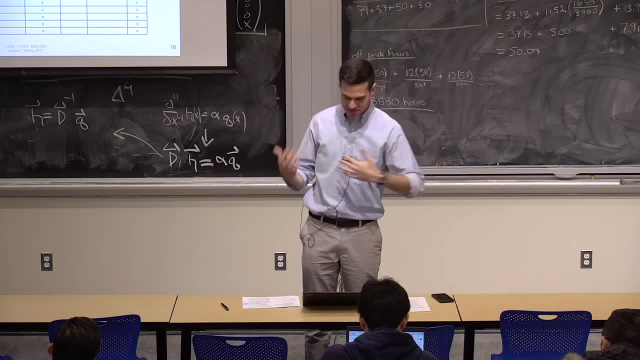 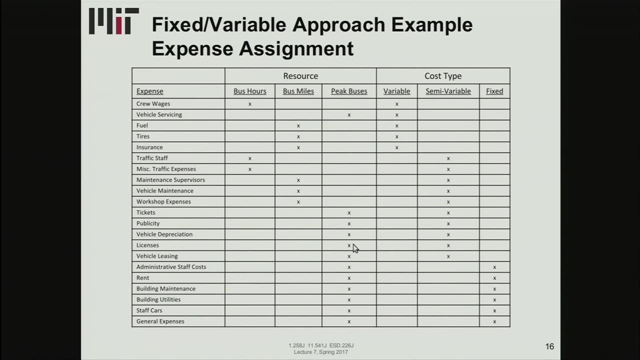 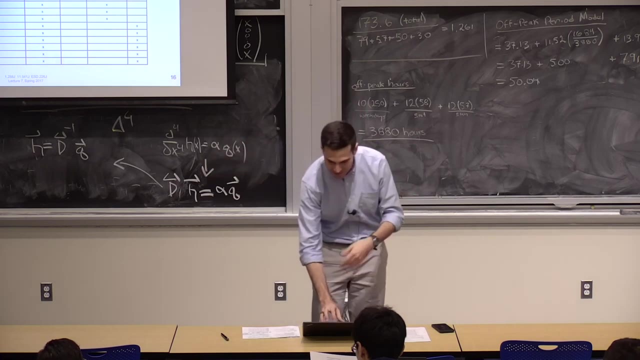 have to cover on each additional bus. So that part is variable. So now we have a semi-variable cost And you can associate that in this case with peak buses, because for each peak bus you have, then that's how many buses you have to plaster with ads. 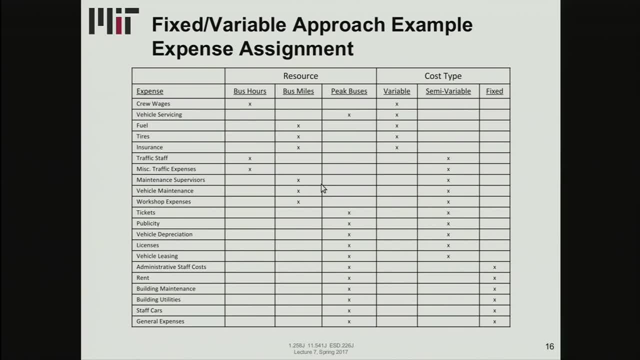 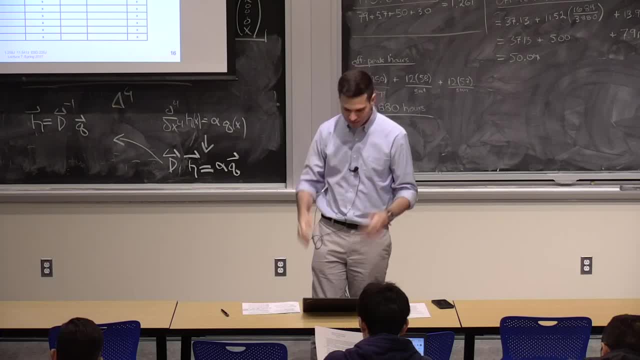 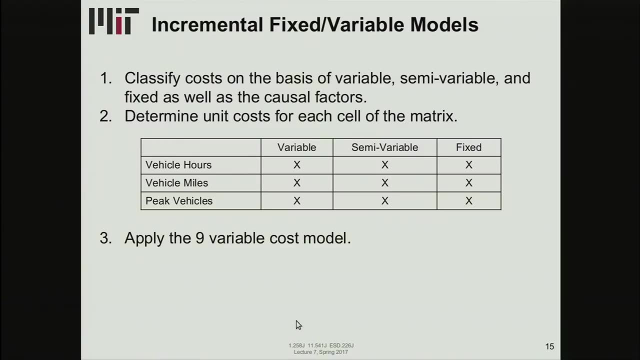 That gives you an example So you can go through each of these. Again, this requires judgment And therefore each person might do it slightly differently, But you use the schedule And you then build your. you calculate your unit costs, much like we did with the earlier examples. 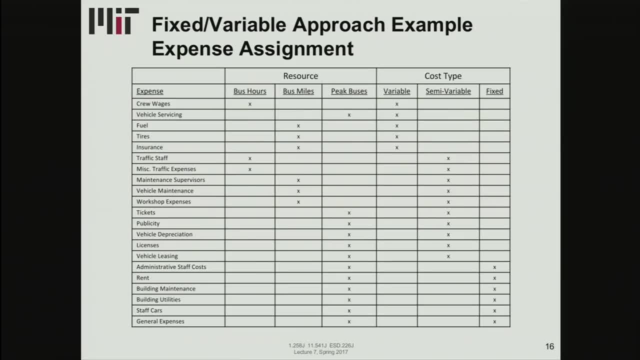 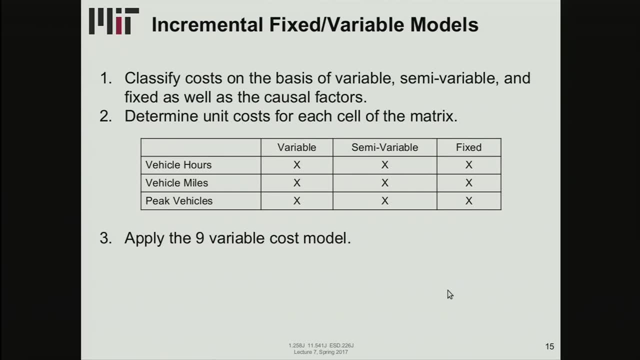 And you then apply it all. So. but now we have more precision. So if you have some kind of new expense or you decide that you're going to save some money somehow, then you decide what? How am I going to spend less or spend more? 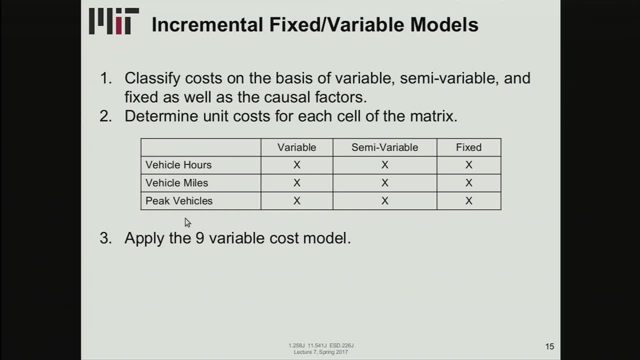 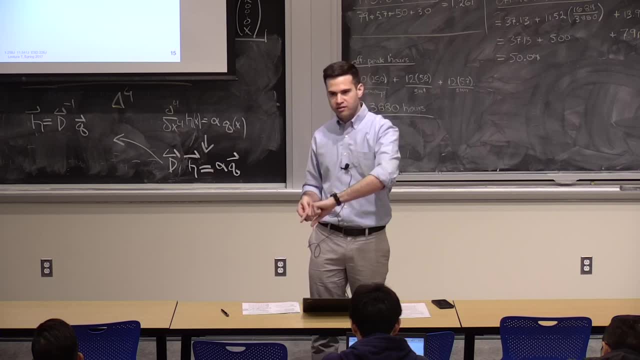 Would that be a variable, semi-variable or fixed cost? Would I associate that with vehicle hours, vehicle miles or peak vehicles And then you would use that unit cost to bring the total cost up or down from the agency And you can even more detailed models. 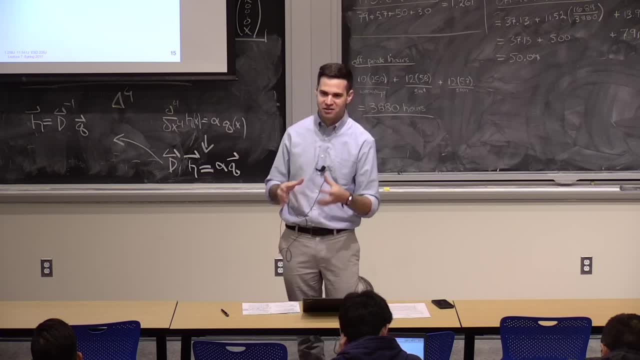 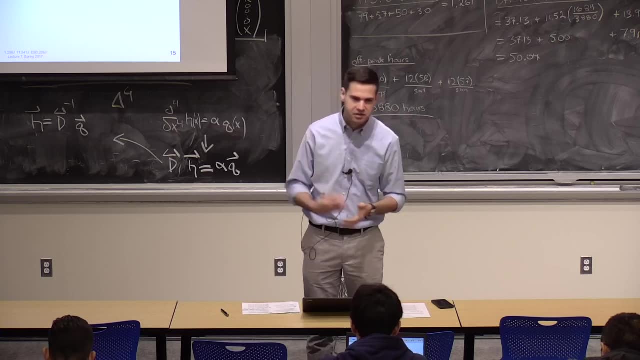 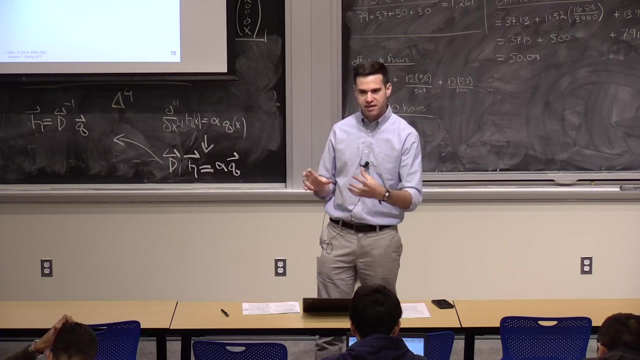 you could just go by expense category and do your engineering style sort of budget if you want to really calculate exactly how much- How much cost you'll save or exactly how much extra cost you'll incur. But these cost models are applied more, a little more. 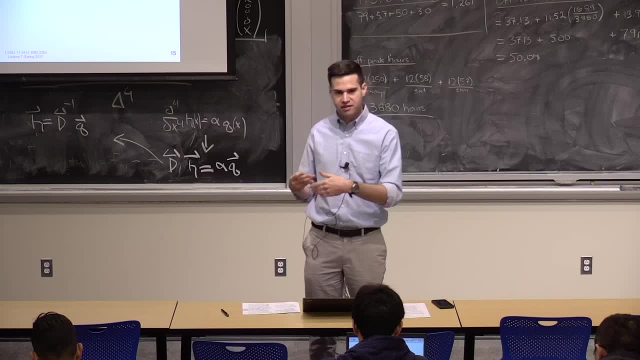 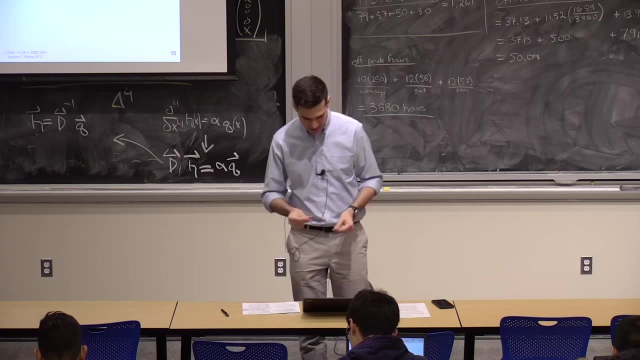 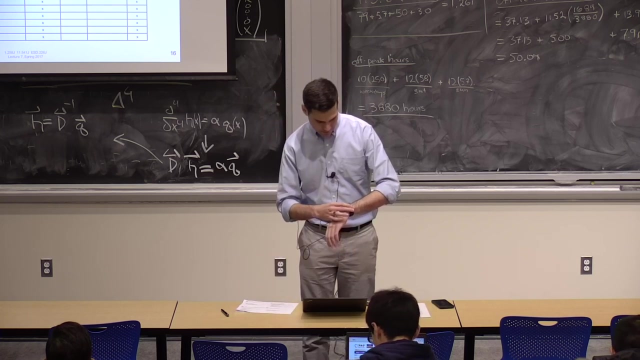 bluntly, in projects where you are evaluating, especially at an early stage, what it would cost And you have different scenarios And you want to quickly know how much it would cost. So questions on cost modeling: No. questions on cost modeling. Yeah, one question. 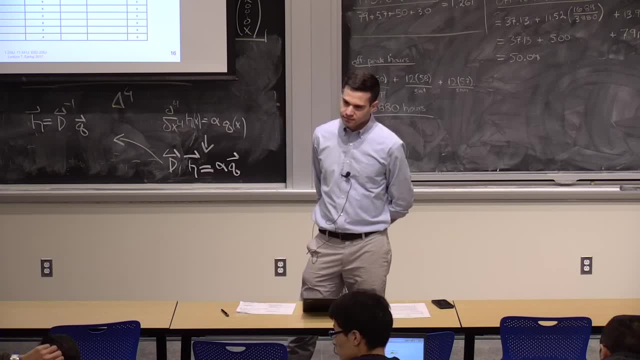 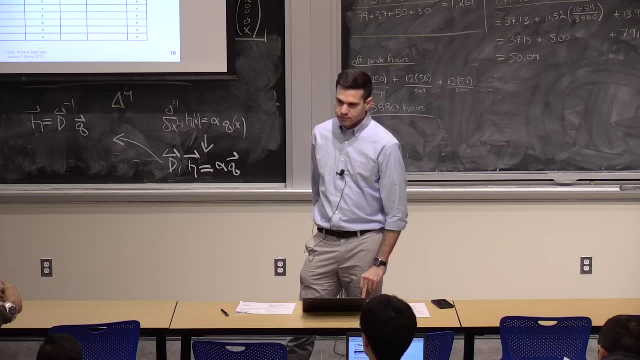 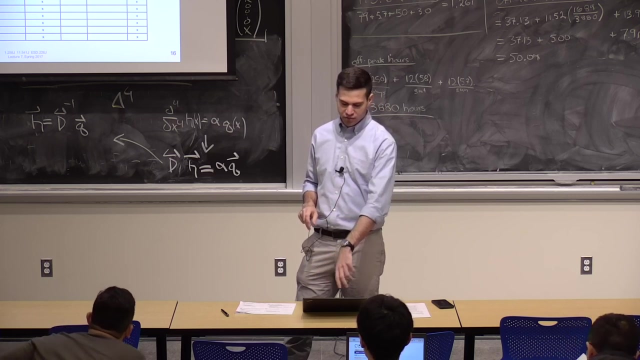 So in this case you would have a more reliability on the proportion of each expense assigned to each factor. Yeah, so essentially you're lumping things a little less. You have more variables, So your unit costs are more precise, And, I think, the ability to move to more sophisticated models. 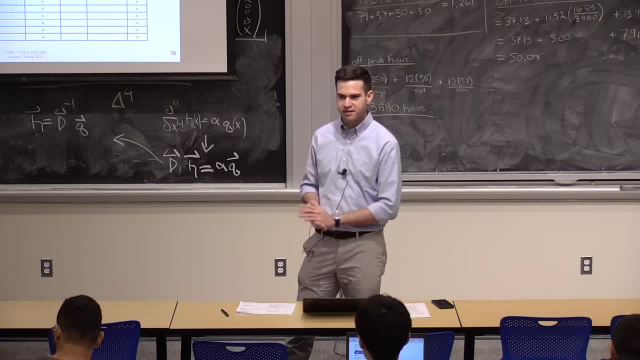 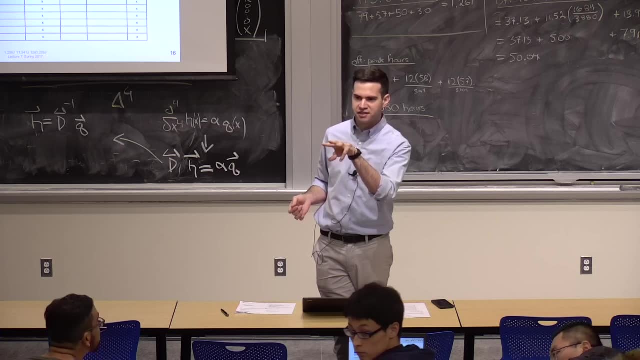 is sort of increasing now that everything is computerized. Yeah, Yeah, It's computer-based. Sonia, do you have a question? No, Sorry, Oh, the three of you have questions. No, Not you. OK, I had a question. 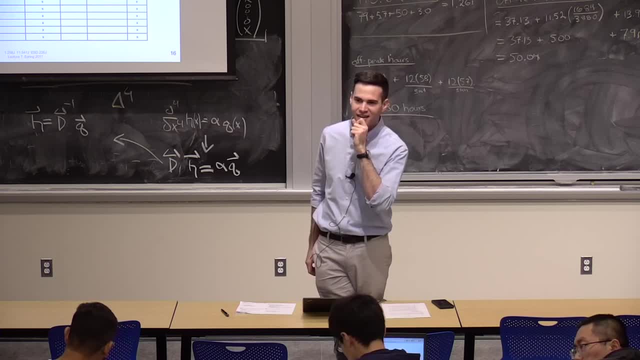 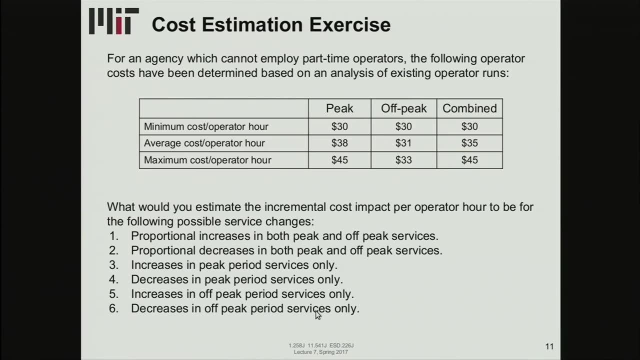 Back on slide 11, you said it's possible that reducing driver hours and off-peak periods might have a factor that could even actually increase costs. It could Well. yeah, It shouldn't decrease, It shouldn't increase costs, But I was going to ask it. Is it ever the case that off-peak service, when there's really low demand, exists simply for the convenience of scheduling shifts rather than needing maximum headways or anything like that? Potentially, But because driver costs are not the only cost of operating. 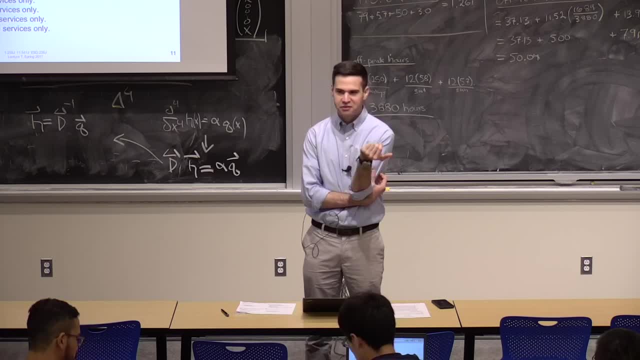 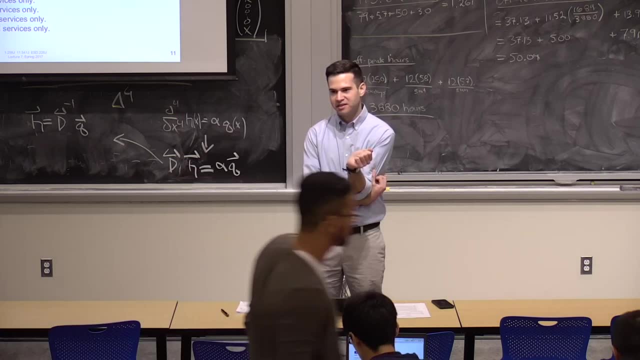 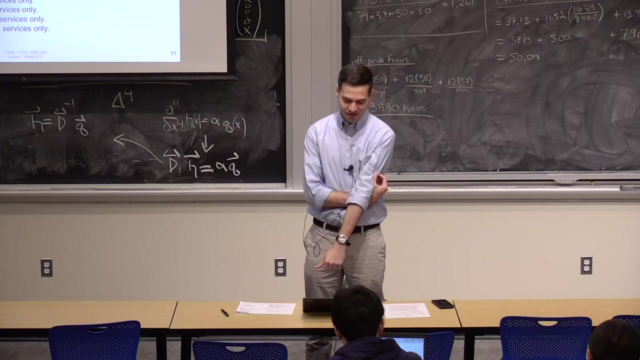 service. you would then also agree to spend extra fuel and extra maintenance costs, And that is also a significant portion of the cost. So you don't, It's not just free. Only this part might be free, not the whole thing. But yeah, I think, if you find yourself in a situation, where your labor agreement requires you to have, maybe there's a cap on how much spread you can have. So you have all these straight runs and they're only working for four hours, And then you say: well, let's just add service. 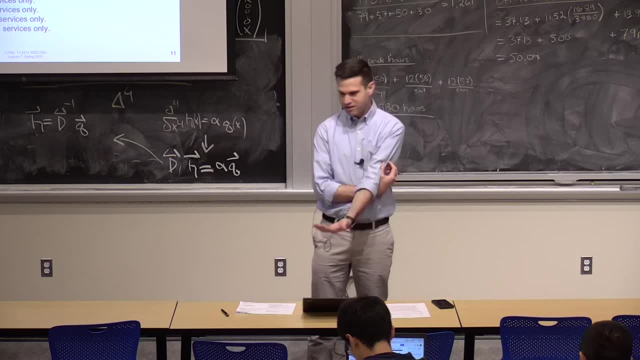 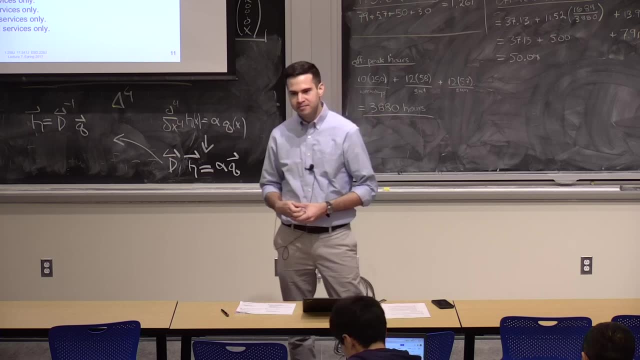 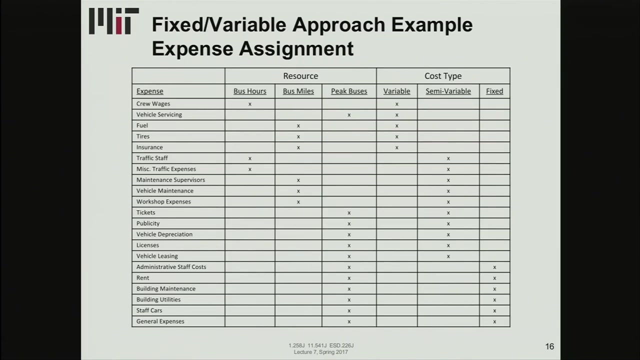 And let's make the off-peak service, which is very good. So, yeah, that could happen, But it's a management decision, That's not something of a science, It's a policy, not a real decision. Yeah, On the last slide we were talking about 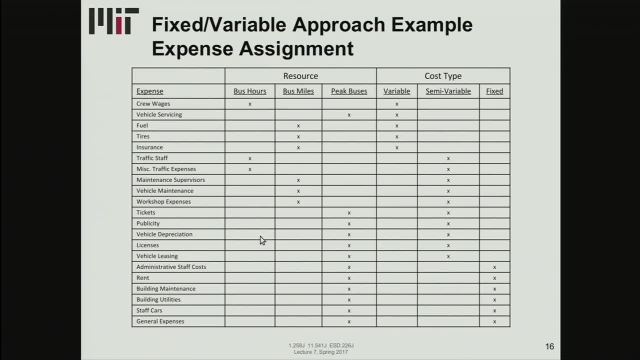 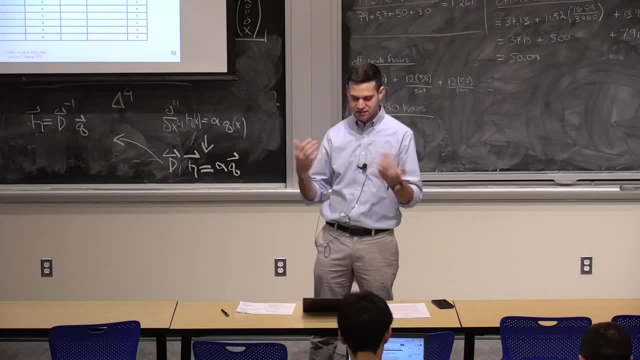 What did you say about being? is it indicative of agency size, or GABRIEL SANCHEZ- Yes, so in this example, we only have three. well, we have nine exploratory variables, which are the combination of the three. 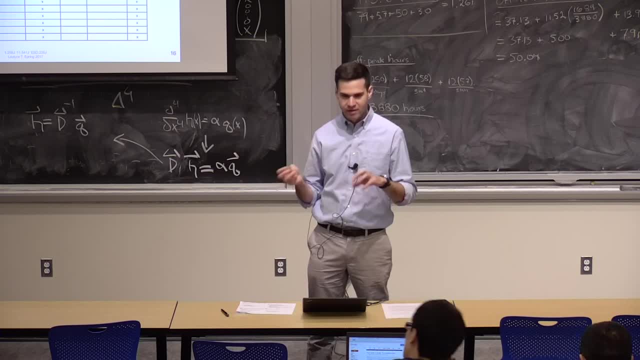 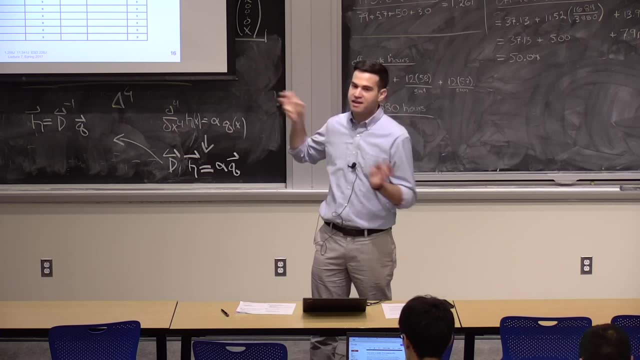 resource variables and the three cost types. But if you go back to the first example in this lecture, we have three exploratory variables- bus hours, bus miles and peak buses- And we have to assign everything to one of these three. So of those three peak buses is something. 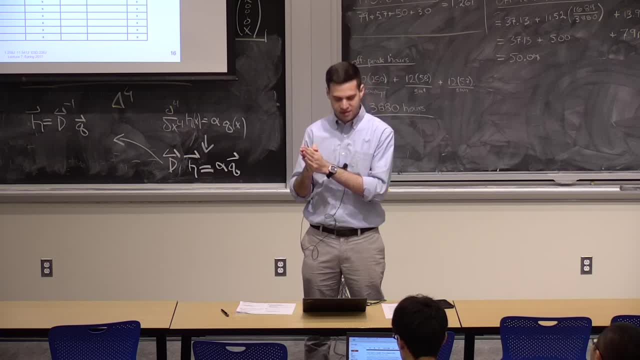 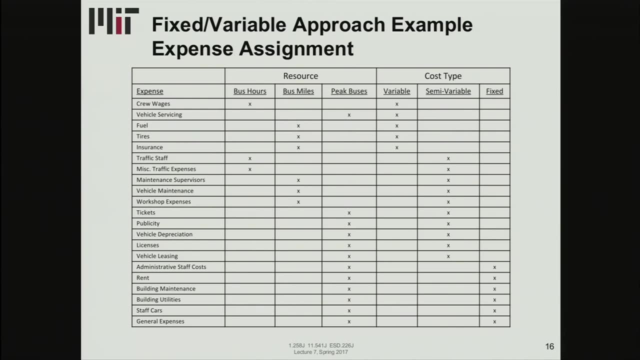 that most closely relates to how large your agency is- right, Much more so than bus hours or bus miles. And if you had other variables then maybe those would be even closer to agency size, But in this example we only have these three. yeah, And why peak buses? Well, because if you have more buses, you need a bigger parking garage for them. You need a bigger refueling and maintenance facility. You might need more mechanics and more right. So the many costs that are mostly fixed. 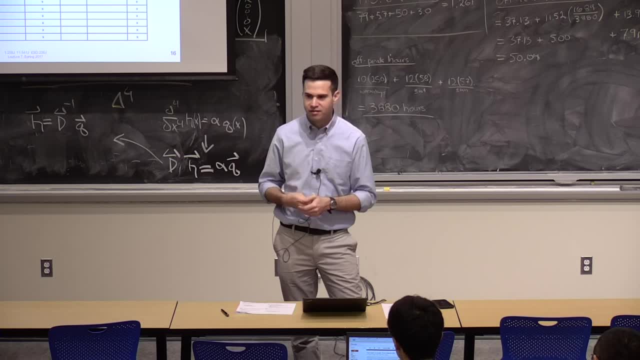 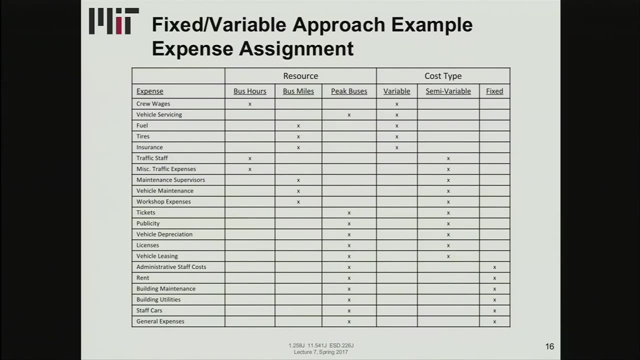 scale up with how many vehicles you have on your garage and how many garages you have and all those things. So another detail which I want to emphasize is that, with regards to variable and fixed, So again, if you have to incur an expense, that 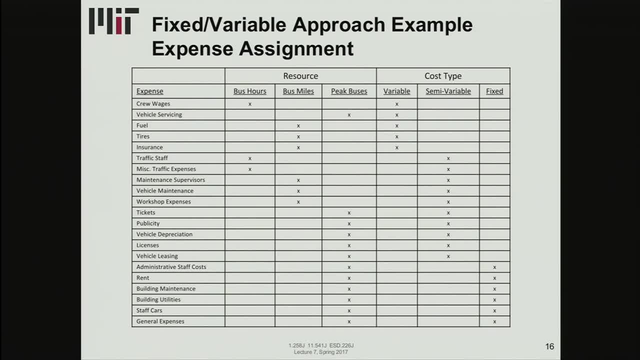 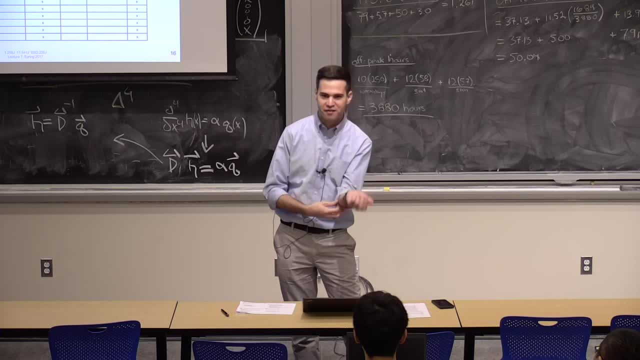 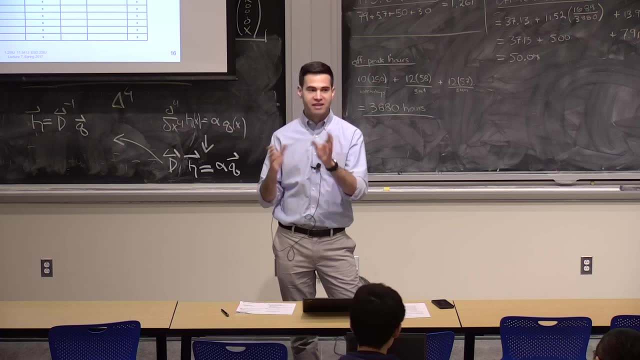 is more marginal, then you might want to use a variable cost model, because you may not need another garage, for example for a few extra buses, But at some point you do incur on. you reach an investment threshold where now you've crossed the line. 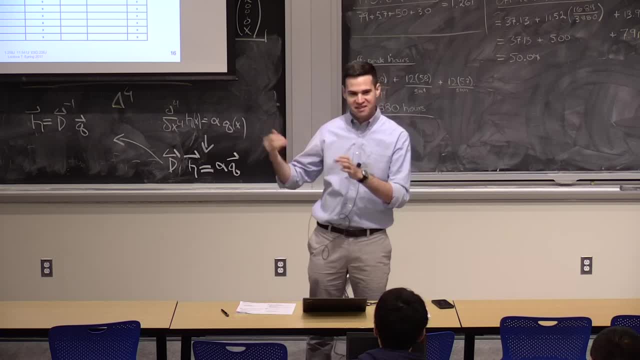 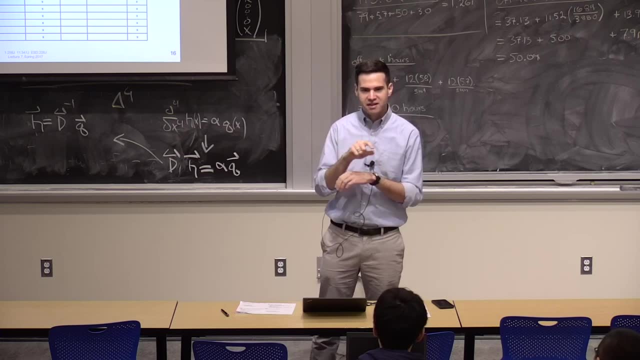 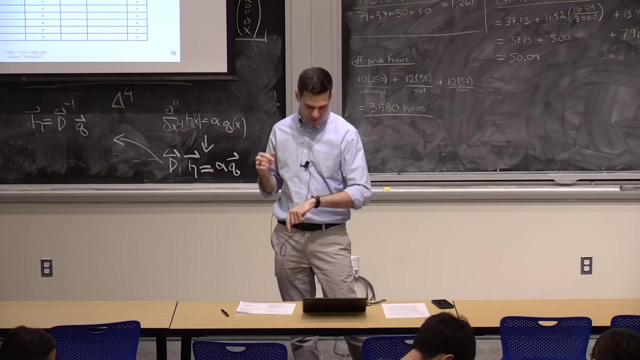 And you do need an extra facility And you have to hire people to run that facility And that's going to be, that's going to increase your base cost. So that happens in lumpy fashion rather than variable and scaling up. We have an additional 10 minutes. 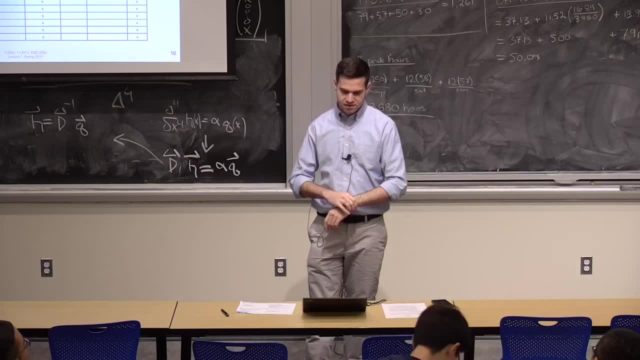 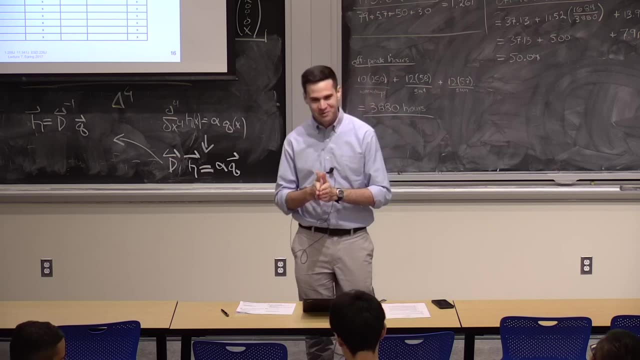 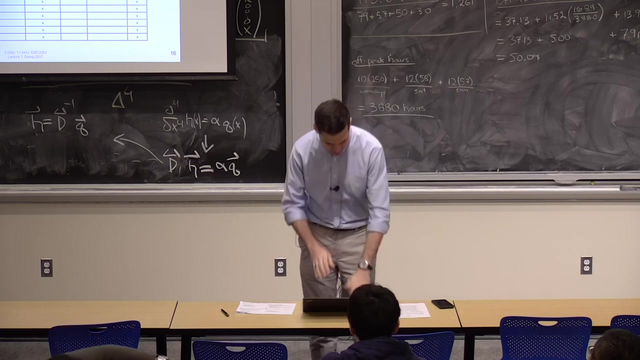 And maybe it would be a good opportunity to discuss the first assignment which I have not finished grading. But I'm sorry about that. I hope to have that back to you soon. But we might as well go over it and just discuss the solution. 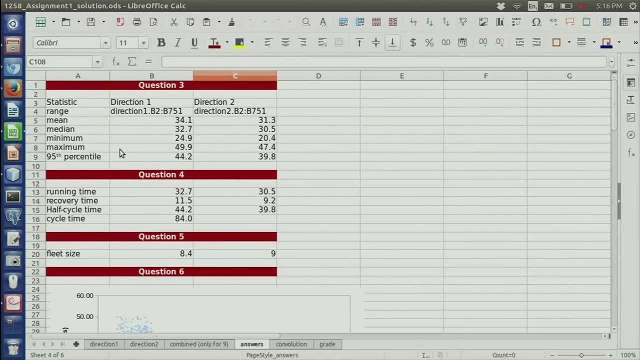 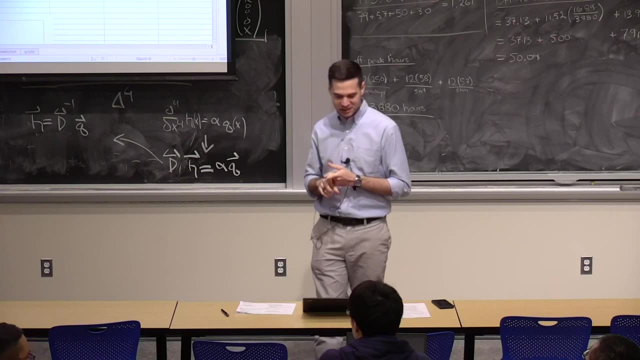 So let me switch to that. OK, So does everybody remember the first assignment, Or is that sort of back in your? So you had some sample data in a spreadsheet And you have to calculate. The first question was: calculate statistics by direction. 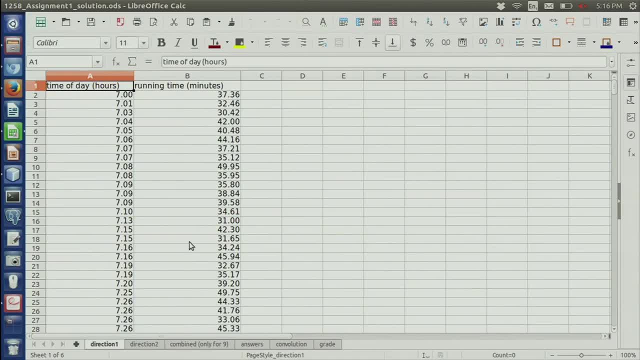 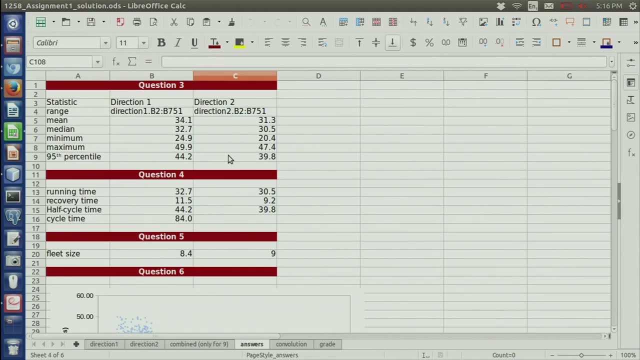 So this is a spreadsheet: time of day and running time. This data was given to you And I like to use the indirect function. I don't know if people know it or not, but it's convenient. So if you type the range name in a cell, 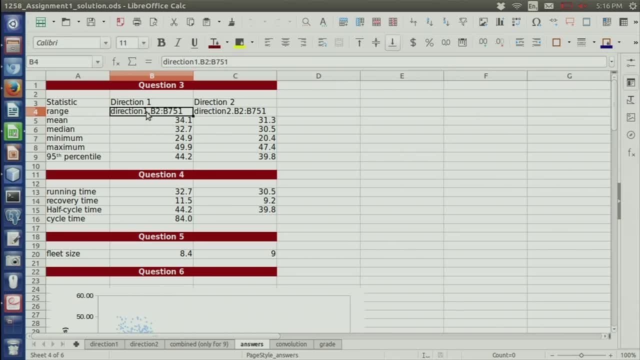 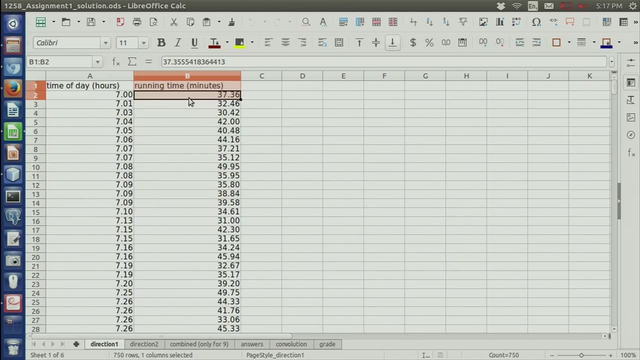 then you can compute things as a function of that range name And that's very convenient. So I selected: OK, So this is the range b2 to b751. And that corresponds to all the data on this first sheet. And then I did the same for direction 2.. 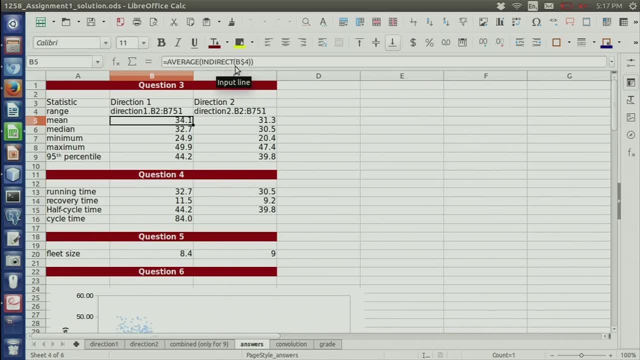 So therefore when I go to mean, I say equals average indirect of b4. And I'm pointing the mean to the range, which is a variable in itself. That's very neat. So you can do that for average median min max. 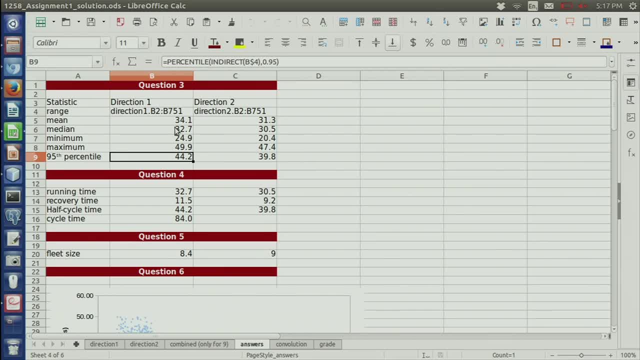 And percentile and then fill to the right, because you have a different range here. So it'll reflect that little trick. So these are the statistics. This was very straightforward. Then question 4 starts getting more transportation itself. This requires some judgment. 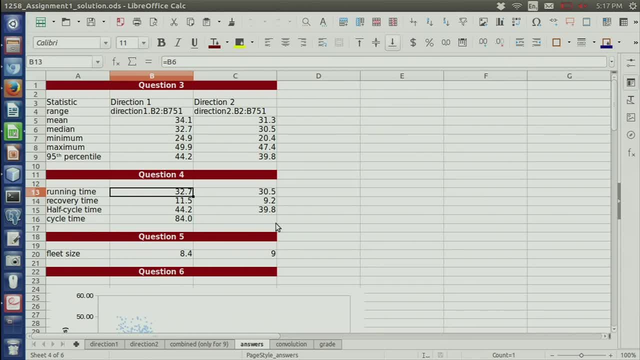 So we're saying: what's the running time, What's the recovery time, What's the half cycle time, What's the cycle time? So running time should be something that happens typically, because this is what you publish on your schedule. This is what's going to go on your journey planner. 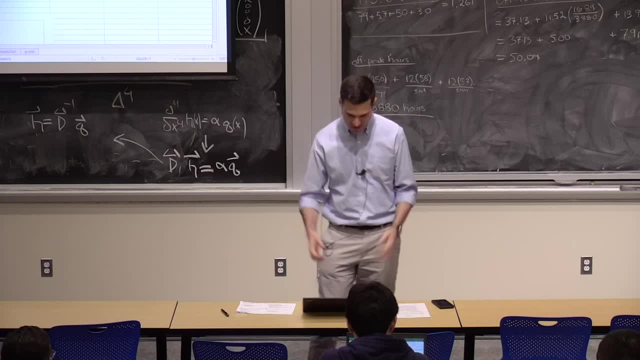 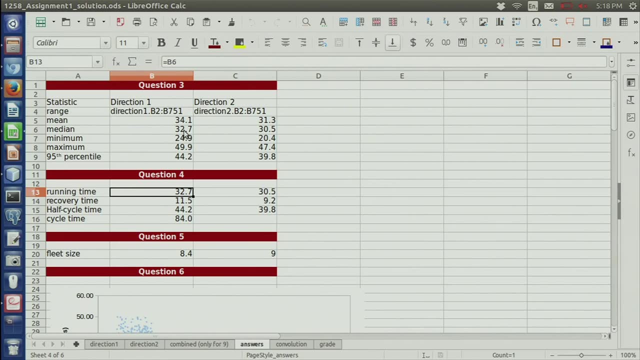 So people need to know what to expect, And therefore running time should be based on the average or the median. Those are the two Of these statistics that you computed before. these should be the two that you use. I usually prefer the median because the average 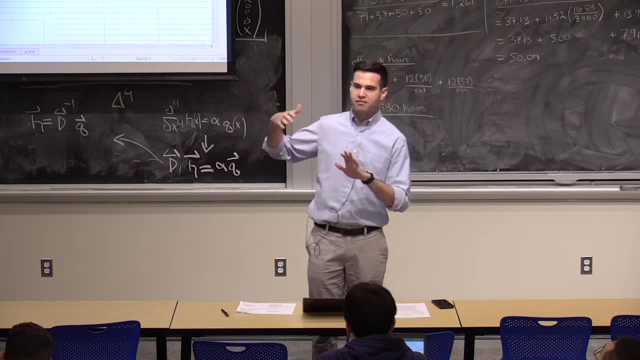 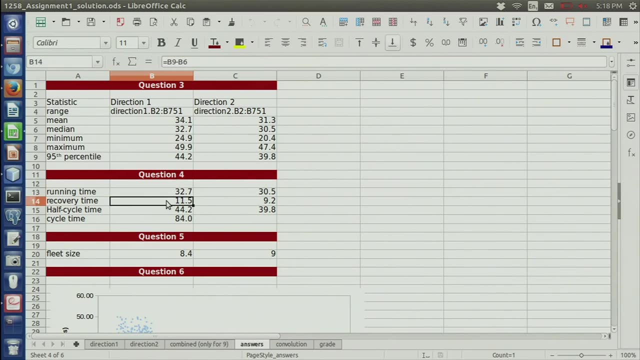 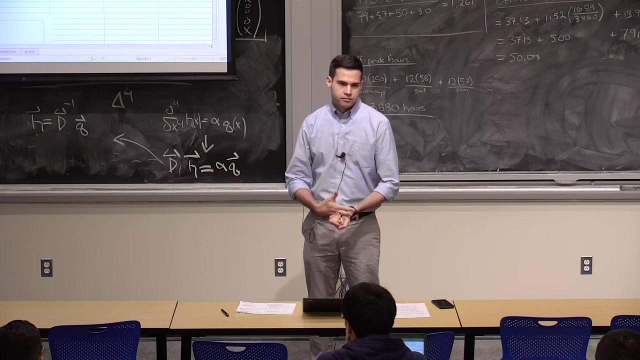 is affected by outliers and by heavy sort of tails on the right quite a bit. So I usually go for the median or the 50th percentile Recovery time. So what is recovery time for? For making up? Well, first of all so the drivers. 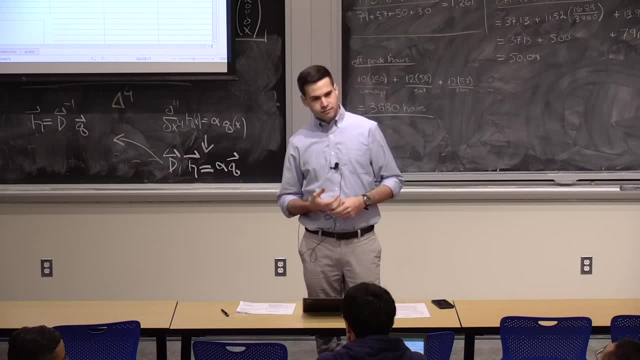 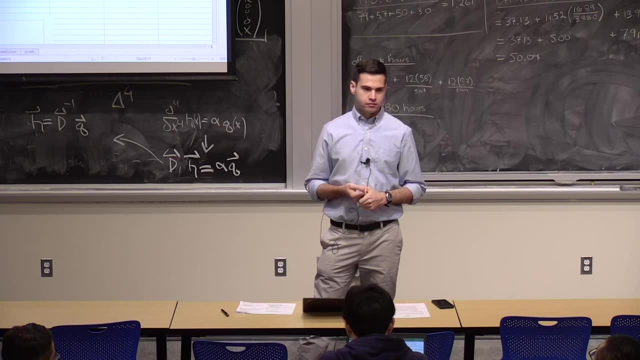 can go to the bathroom and things like that. And then, second of all, to make up for problems in the schedule. So say, I'm driving out on this bus route and it takes me eight minutes longer than I thought it would. GABRIEL SANCHEZ- I wouldn't. 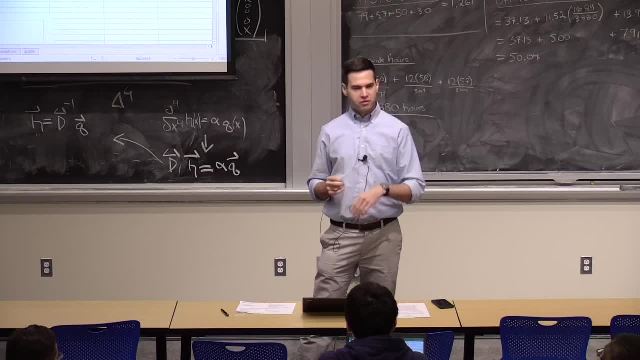 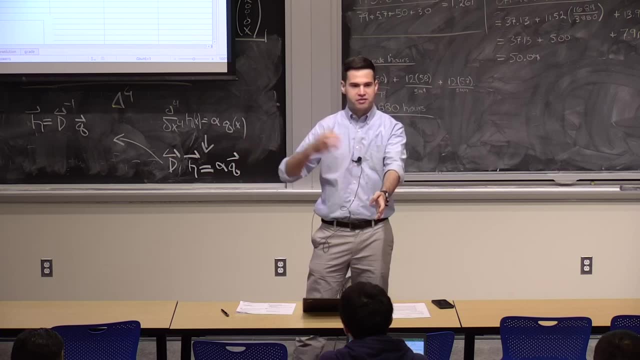 characterize it as a problem. It's a problem with the schedule per se. So the schedule is a deterministic decision about how long it will take you, And the reality is that the running time is a stochastic variable. It varies from run to run. 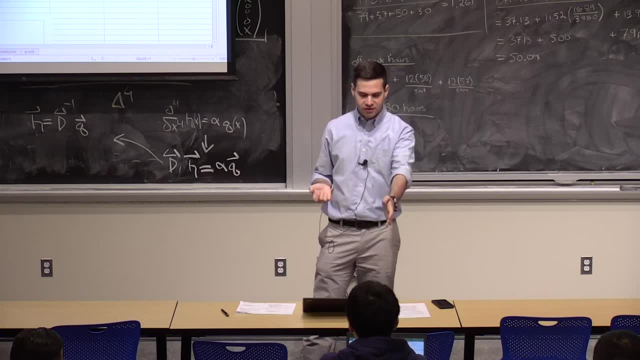 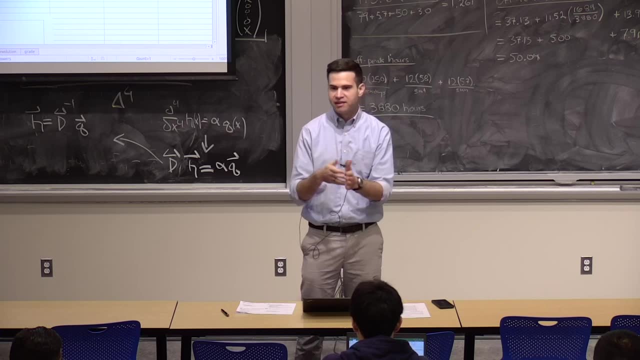 So you want to say, you want to make a claim about what the typical running time is, But then you have to have some recovery time to account for anything later than that And you recognize- it's a way of recognizing- that these running times are stochastic. 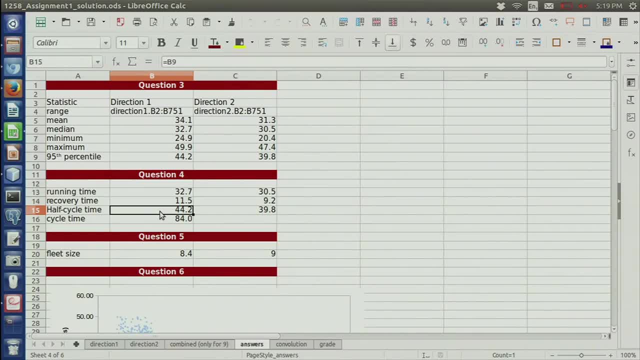 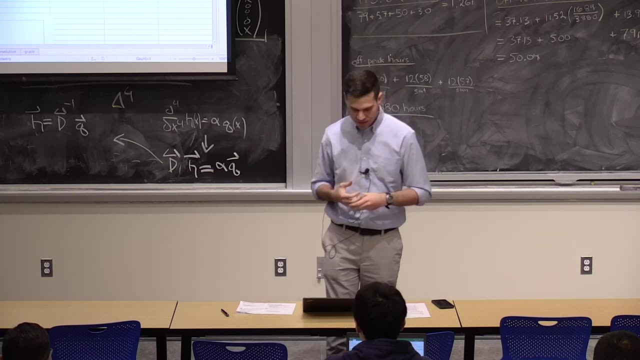 So the half cycle time is how much time you budget for the run, including those late ones. So I set that to a high percentile, the 95th in this case. The reading was suggesting that you could use 15% times the average or things like that. 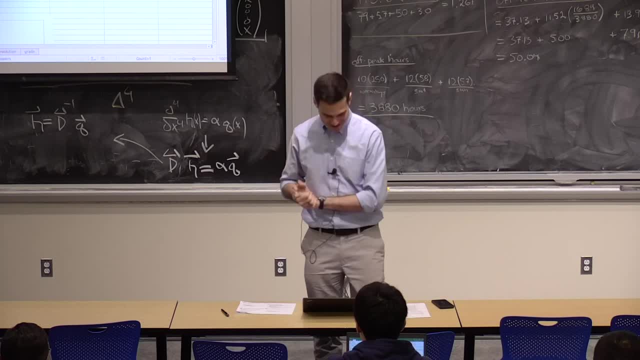 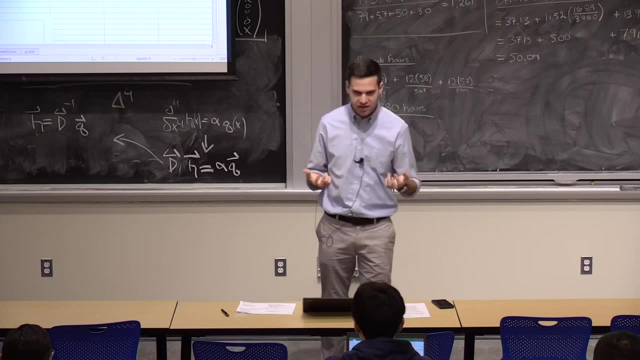 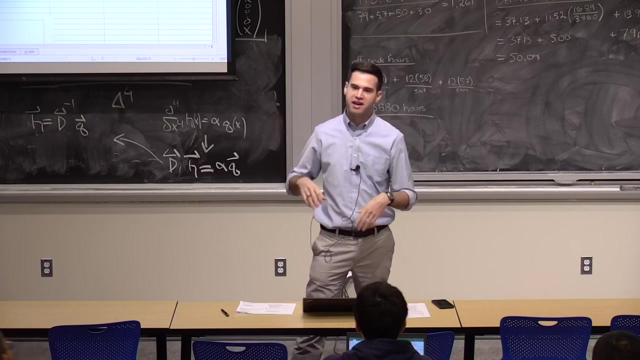 When you have data, then you should use the data. So the technique of taking an average and multiplying it by percentage is what the industry typically does When you don't have automatically collected data, when you essentially send someone out to drive behind the bus or to do a write checker to collect. 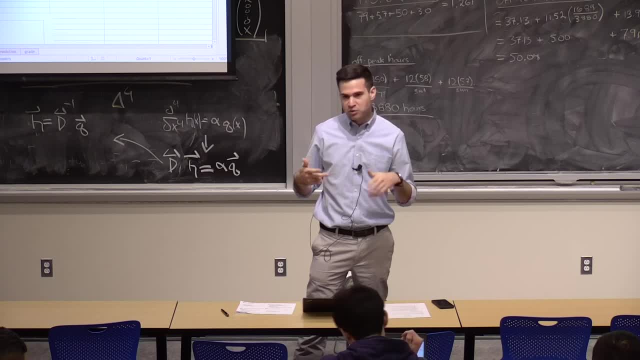 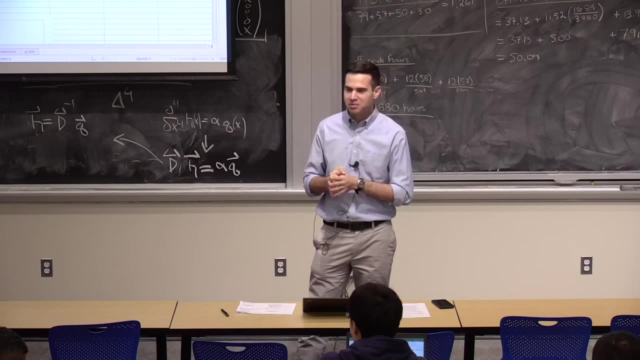 data on the bus and you do five or six, maybe 10 trips and you get an average And that's not enough to estimate your high percentiles because you probably didn't see the high percentile in those only 10 trips. 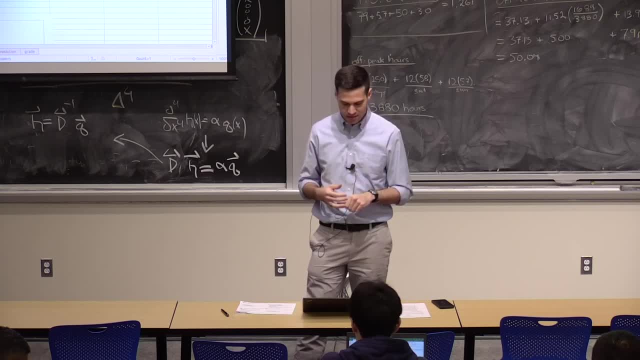 So therefore, you have to rely on a different method, And then you could multiply it by a percentage. But if you have data, Then you should use the data, And 10%, 15%, 20%- whatever you use- might not be adequate for a specific bus route. 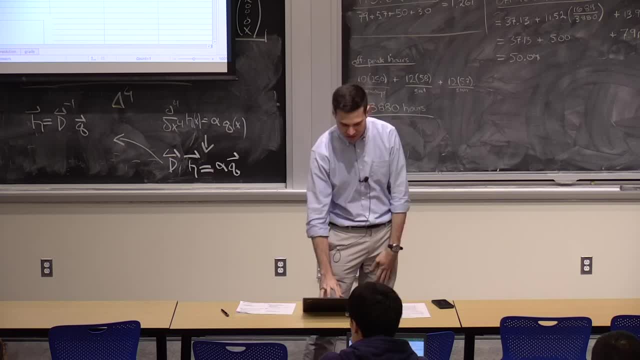 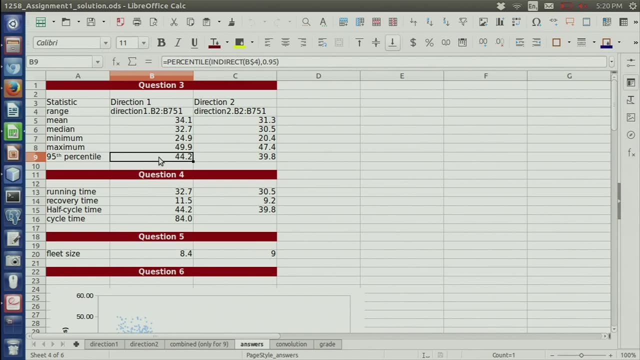 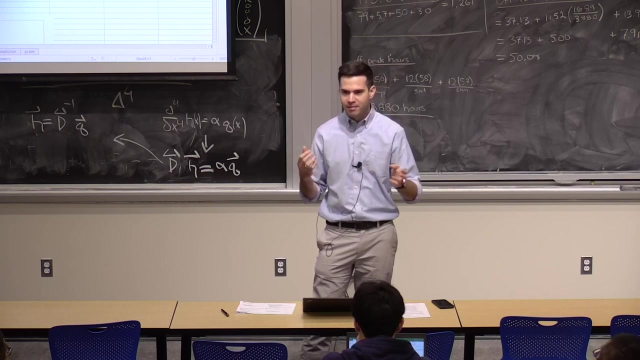 So because you have data, you can actually measure how variable it is And therefore high percentile is a better choice. 95 is 1 in 20, right. So if you think of there being 20 weekdays in a month, then you're saying well about if for that for the 8 o'clock. trip. I expect it to be late about once in a month. To start out late, GABRIEL SANCHEZ-. To start out late because for there to be a knock-on effect on the next trip, essentially, And for every other time of the month. 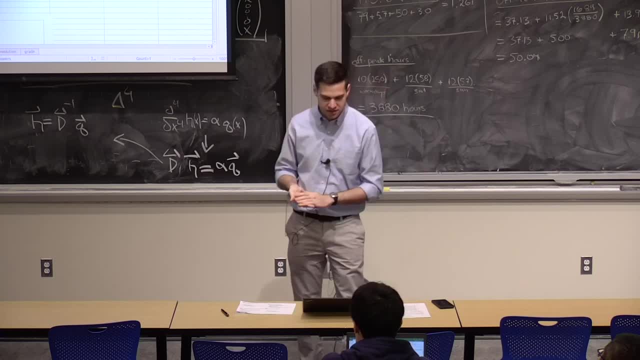 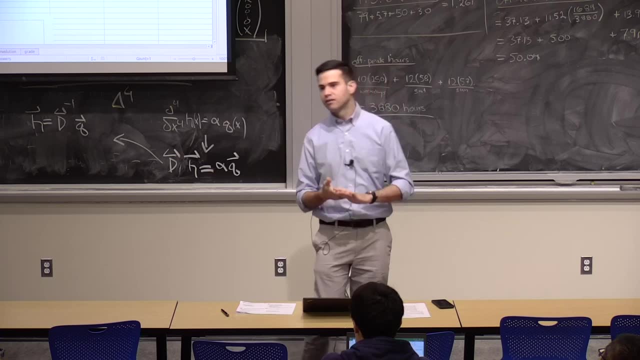 I expect it to run smoothly, So that's why 95 is a typical choice. Lower numbers of percentiles are common, especially at high frequency service: 90, 85. Question on the back: Yeah, So how do you use the 95th percentile for the recovery? 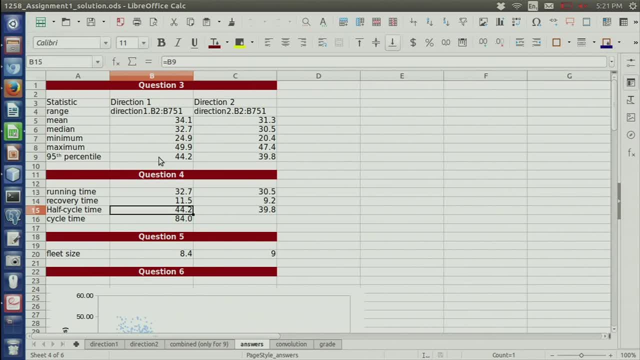 GABRIEL SANCHEZ- So the half cycle, exactly The half cycle- is the 95th And the recovery time is the difference between the half cycle and the typical. So on your journey planner, you only put the running time. 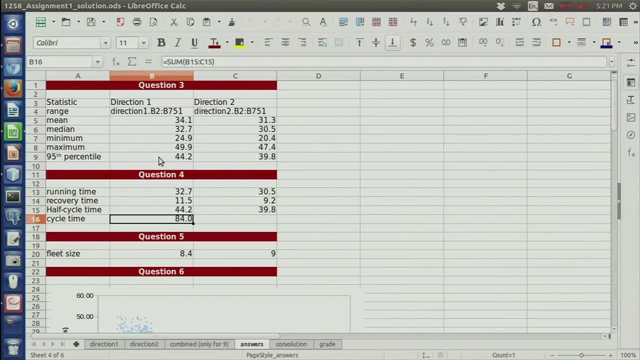 But then between trips you add the recovery time And then the cycle time is the sum of both half cycle times. So that's pretty straightforward. Question five was: how many vehicles do you need to operate this? And there's an equation which is maybe: 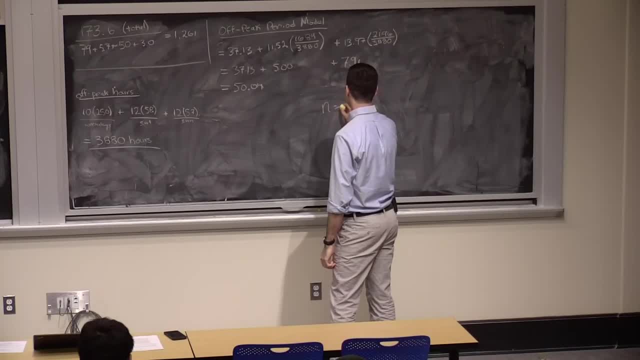 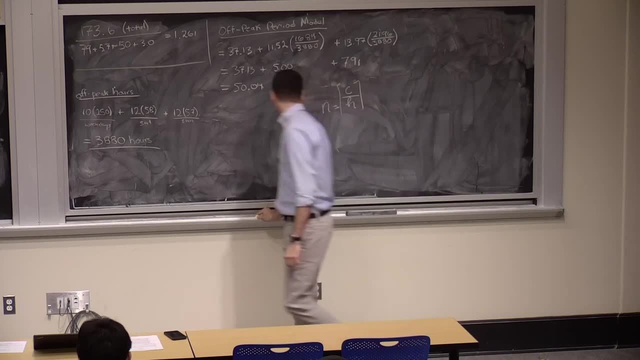 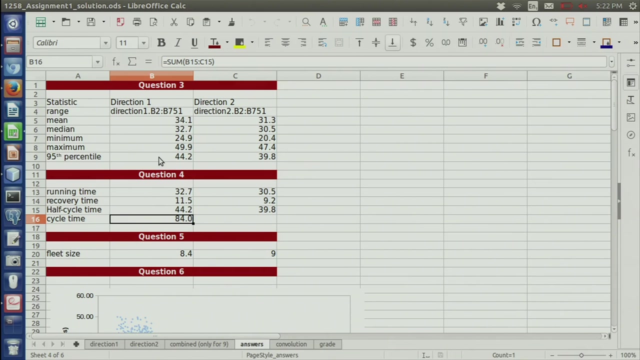 the most important equation in the whole code. of course, Number of vehicles equals cycle time divided by headway, And you need to round up. So cycle time is 84 minutes. The headway we said was 10 minutes, So that's 84 divided by 10.. 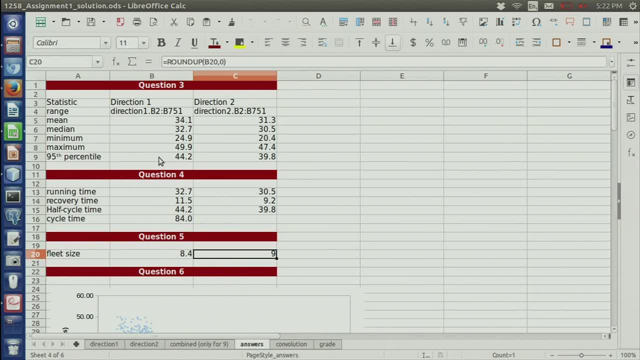 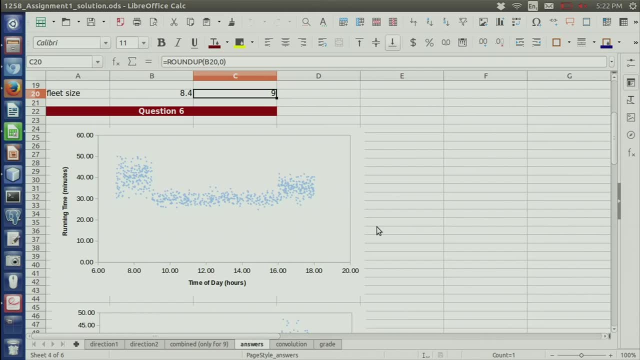 It's 8.4.. Round up, that's nine vehicles. OK, So you need nine vehicles to operate the bus route. Question six asked you to plot the times. Hopefully, you labeled your axis and did everything like you should, And so here's time of day. 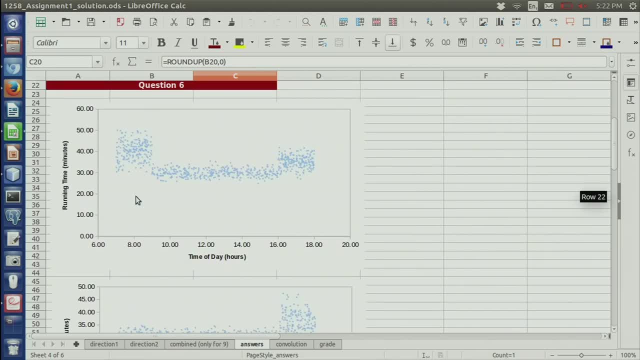 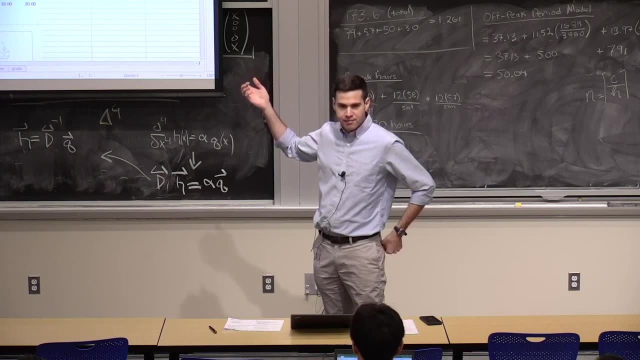 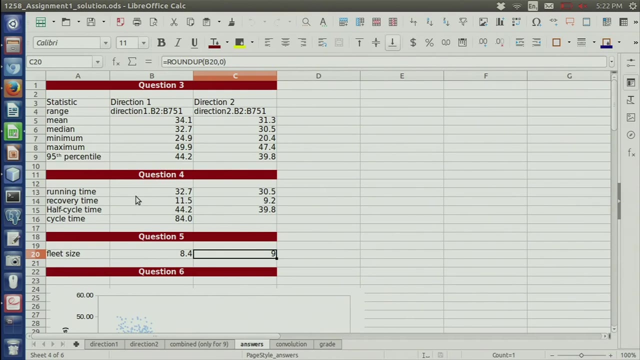 And here's running times in direction one, running times in direction two. And we identify that not all of these running times come from the same operating environment. We can see that there are some peaks and some off peaks And, uh-oh, we just calculated everything wrong. 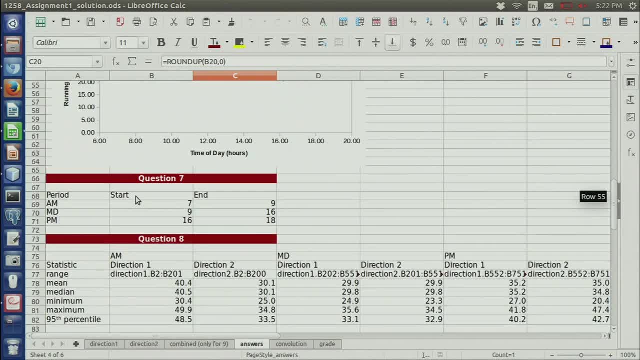 because we mixed up all the data we shouldn't have. So the question was: what are these periods? So am peak going from 7 to 9,, midday from 9 to 16, and pm from 16 to 18,, using the 24-hour format. 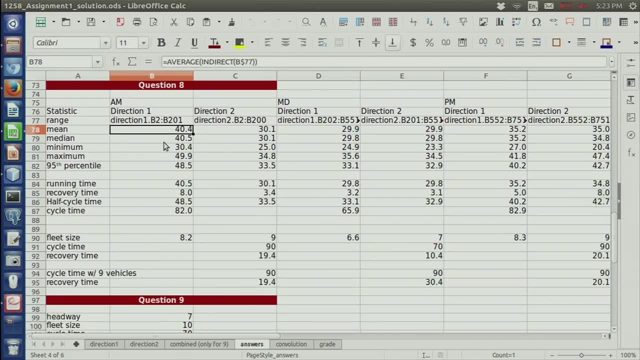 And now we have to redo all the work. We have to compute the same statistics. I've just changed the ranges and copied the formulas from below and the fill to the right And we have all the statistics. So that's great. We repeat the calculation. 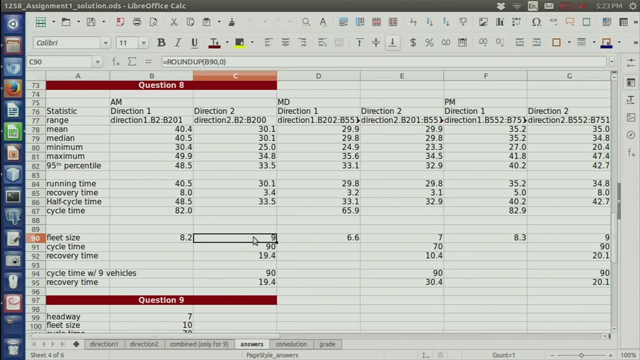 And we get the vehicle requirement by a period now. So we have it. We still need nine vehicles in the am and pm peaks, But it turns out that we only need seven in the base between peaks. So that's great. 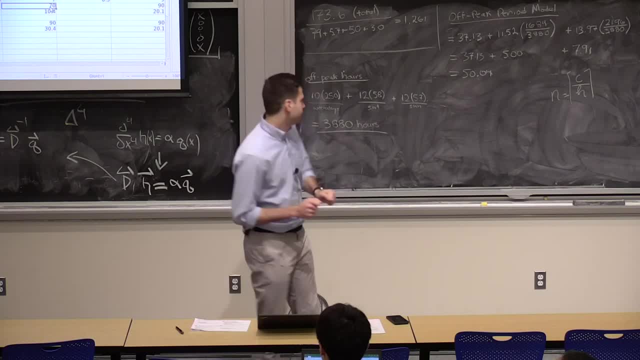 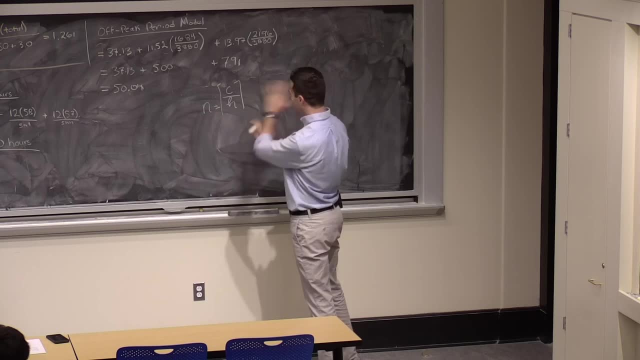 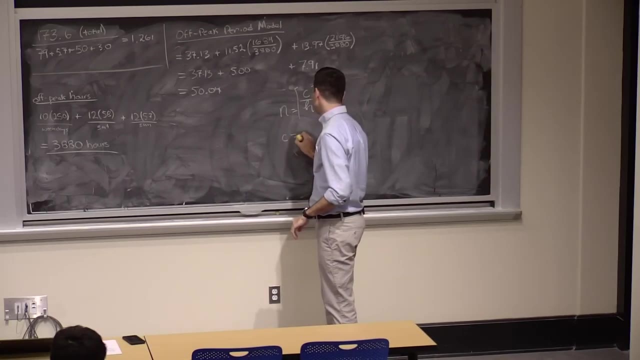 What's the cycle time? The cycle time. once you've calculated, you can flip this equation. I could have an entire lecture on this equation. You can flip it around And there's many ways of interpreting this equation. But if you solve for c cycle time, 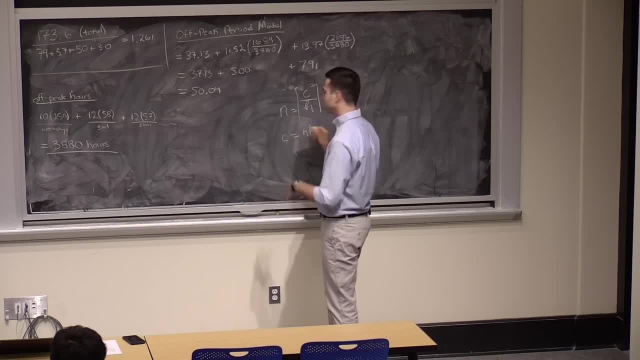 equals number of vehicles. times headway. Now you don't round any direction. So once you've decided what n is, then you solve this equation for c and revise your cycle time, Because you round it up, your cycle time will have gone up. And therefore your recovery time will have gone up. So the cycle, the revised cycle time, is 90 minutes am at pm peaks, 17 minutes off peak, And the recovery time is the difference between the day typical running time and that cycle time. 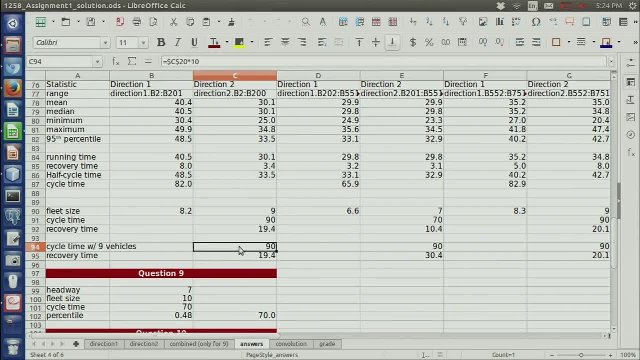 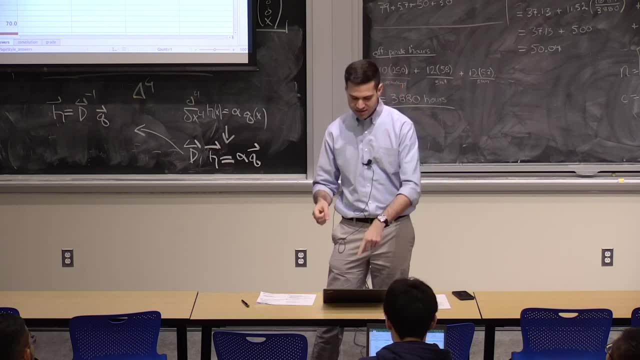 So then I asked: what if you had done the mistake of using all the data combined? That means that you're fine on the am and pm peaks, but you would be excessively provisioning resources in the off peak. So your cycle time was 90, because you. 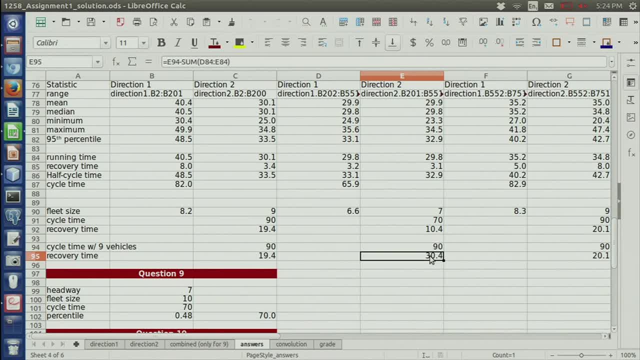 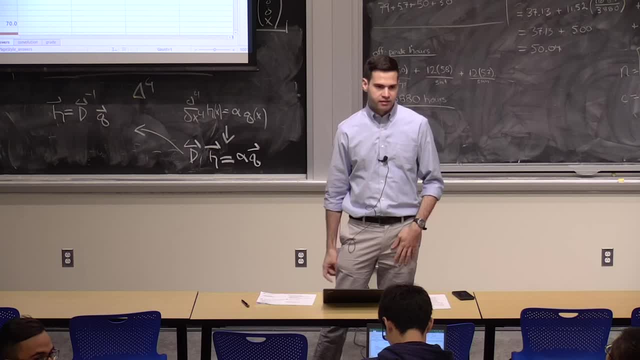 said it was nine vehicles And that recovery time would be 30 minutes and a half, which would be excessive. It's fine if we use the average instead of the median. Yeah, yeah, I prefer. I think the median is a better choice. 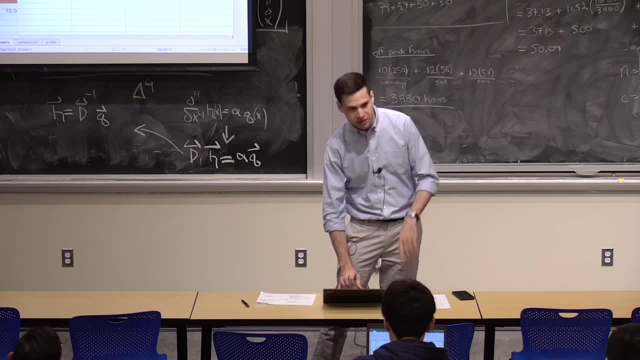 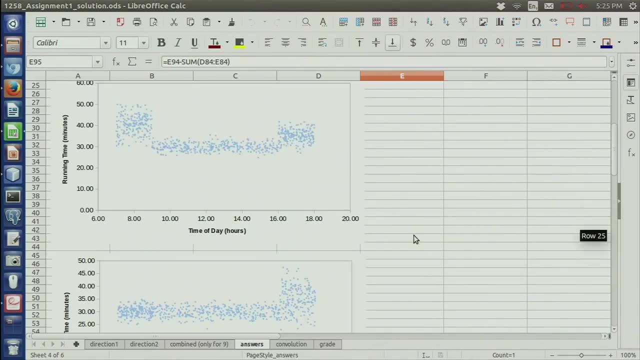 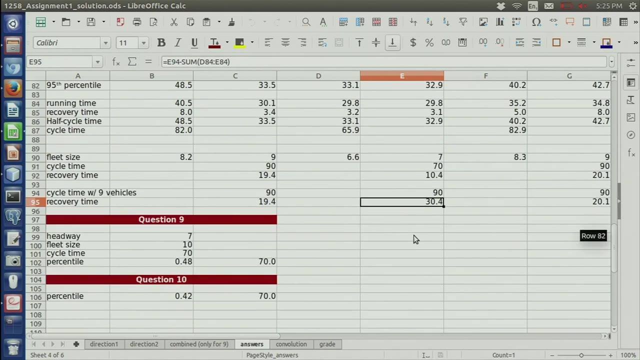 but both are fine. yeah, Especially if you remove outliers from the average, And this data didn't have outliers. As you can see on the graphs, it's very suspiciously clean data, right in very precise places where the period begins and ends. 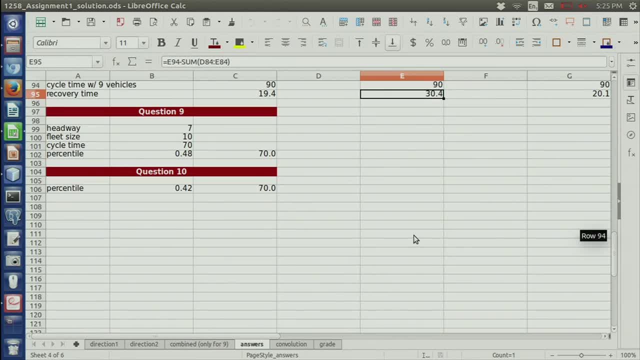 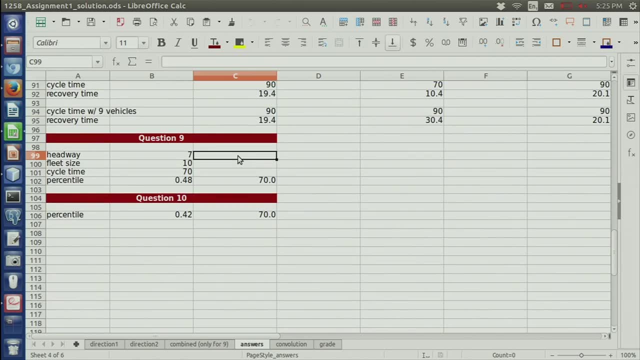 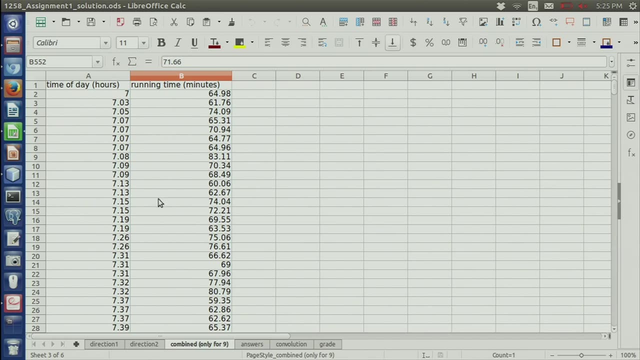 The data you'll get for assignment three does not look like that. So all right. Question nine said: Now imagine that this bus route runs in a loop. It only has one terminal And I provide data. We have data here for that combined operation. 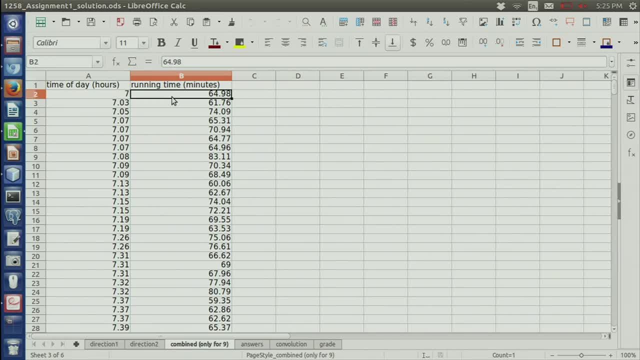 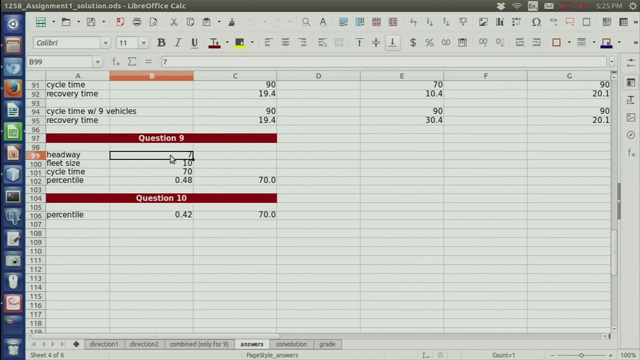 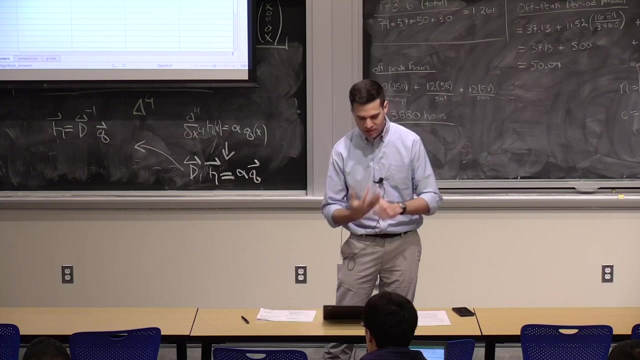 of running inbound, downbound and coming back. So what is the? we said we have a headway of seven minutes and we are running with a fleet size of 10 vehicles. How reliable is this service? Well, we can compute from the headway and the fleet size. 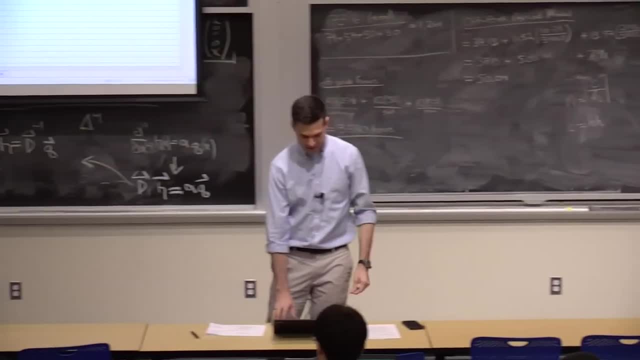 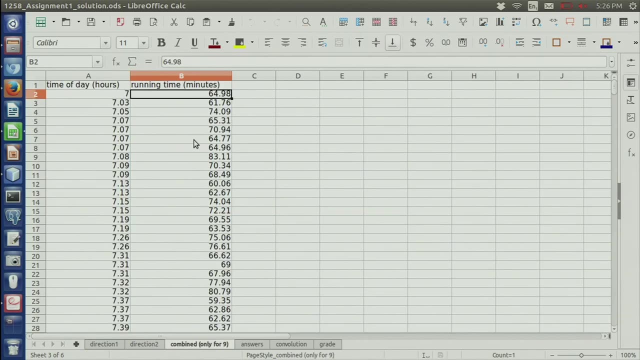 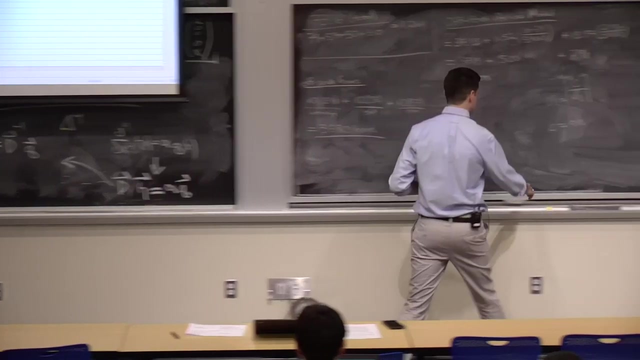 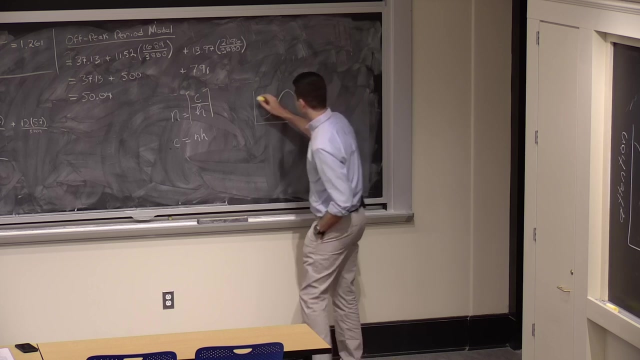 the cycle time using this equation right here, And we have 17 minutes. And what we want to do then is: from all these observations, you can think of this as a probability distribution, right? So we have some distribution of running time. This is probability density. 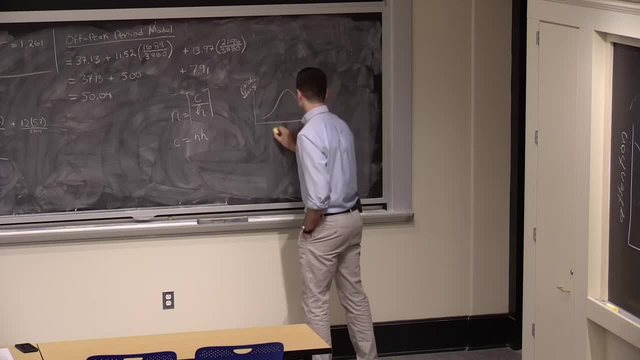 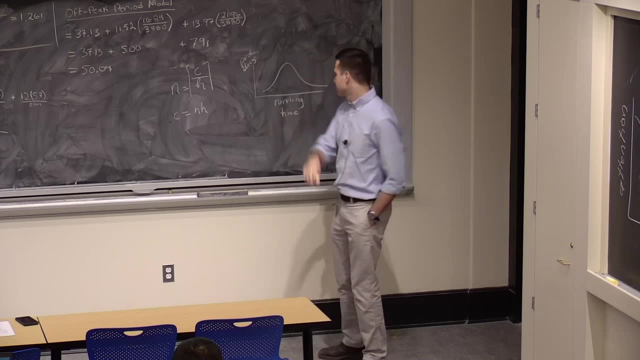 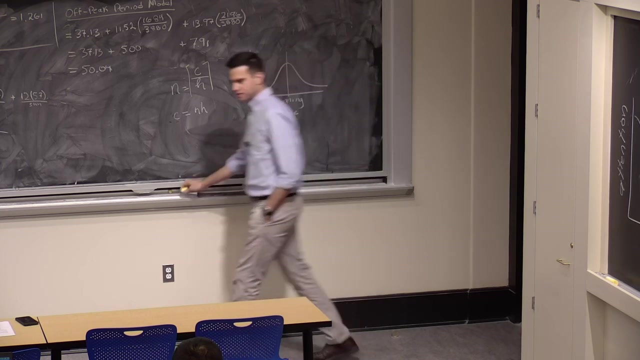 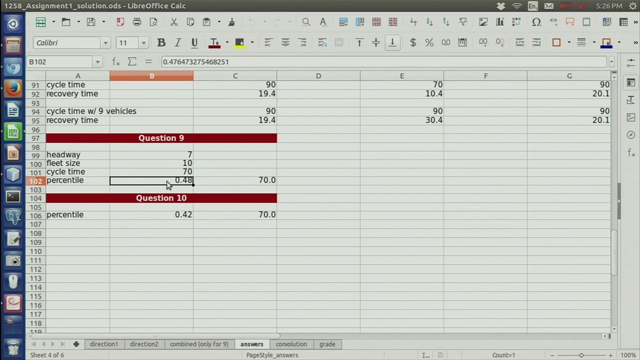 And this is running time And we said the cycle time is 70. So 70 will fall somewhere around here. it turns out, if you look it up, That's very close to 50%. So the way I computed it, I used the spreadsheets Solr. 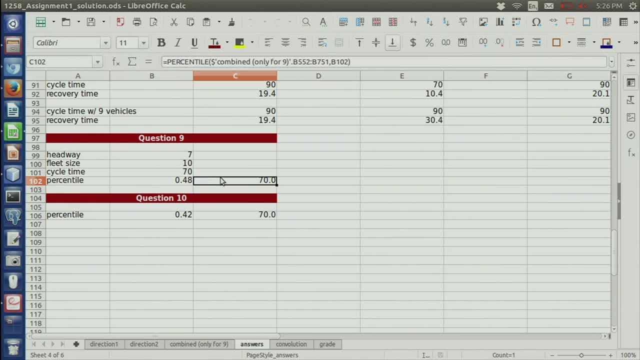 Go-Seek different names for it. So I said: calculate the percentile of whatever percentile I give you here, right? So initially I set it to. I don't know, maybe I set it to 95, right, And it gave me the percentile. 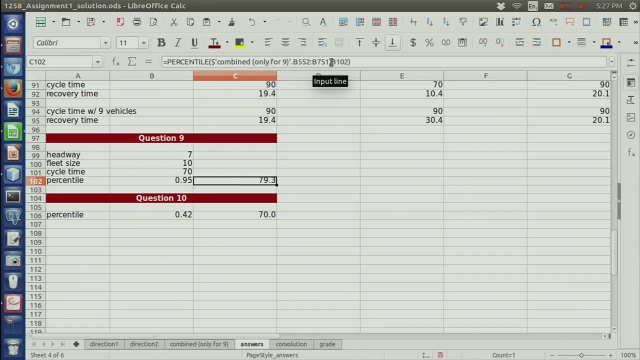 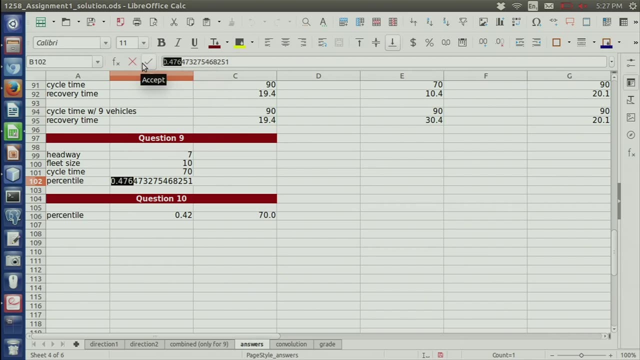 This percentile is running on the AMP data or whatever it is on spreadsheet 9.. And then I said: change that percentile such that this cell equals 70. And it solved it And it gave 476.. Probability OK, So is that reliable? 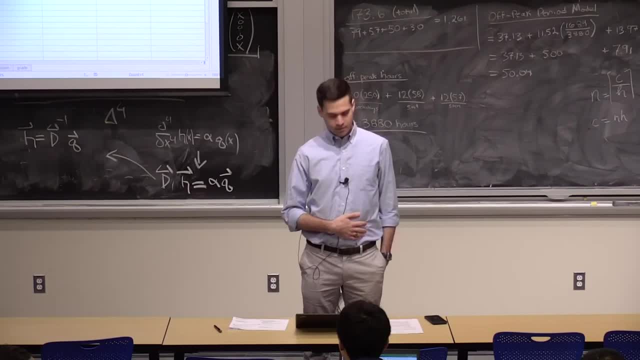 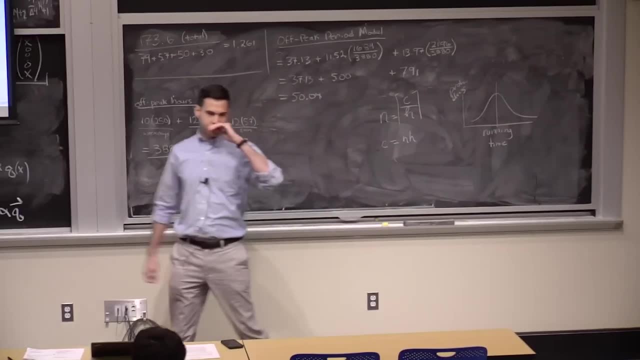 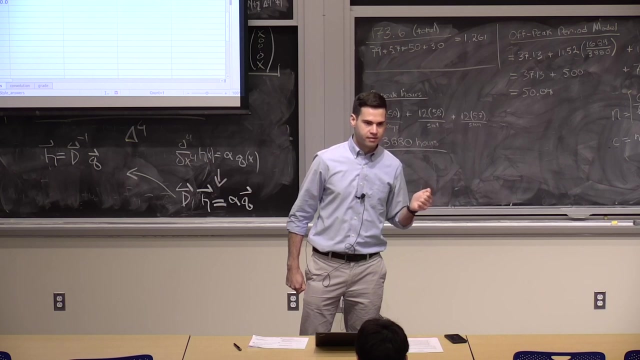 Yes or no? No. So what's that probability? GABRIEL SANCHEZ- That's the probability that you can run in 70 minutes or less And therefore you don't cause delays on the next trip. Your next trip can be in on time, OK. 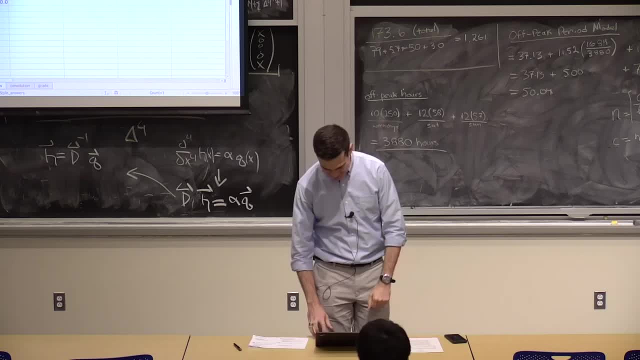 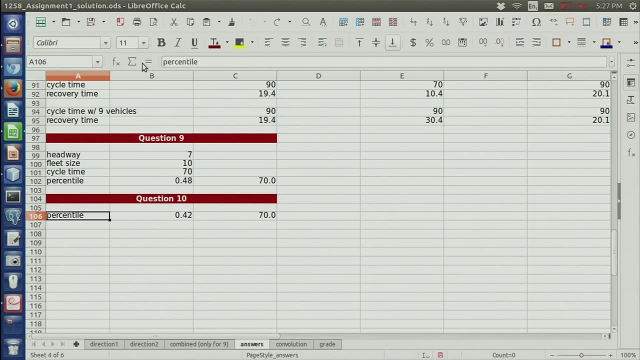 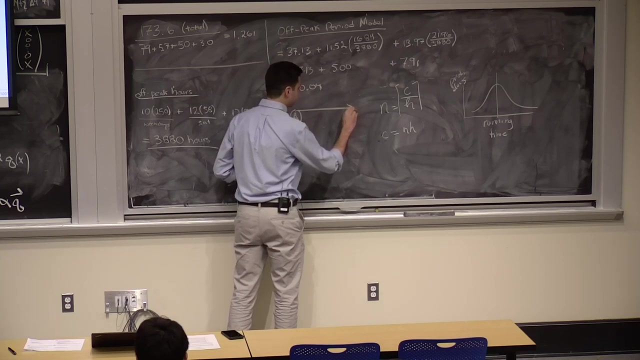 Sorry, Not reliable. GABRIEL SANCHEZ- Not reliable. Thank you, OK. So question 10 is the challenge question. So now you have two terminals, So now you have recovery. You start at A, You go this way: 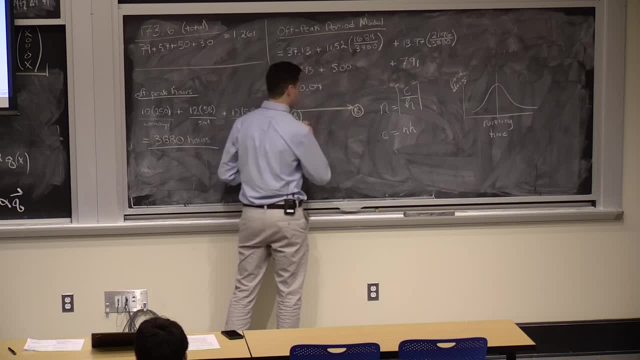 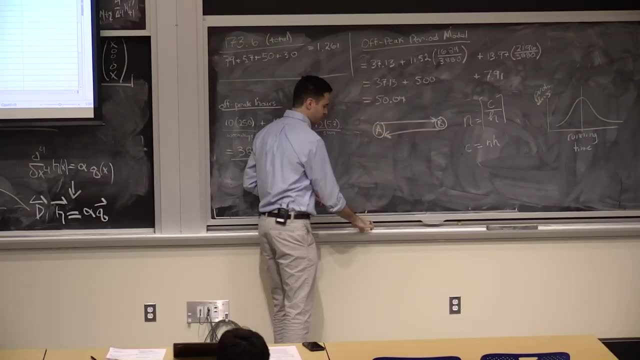 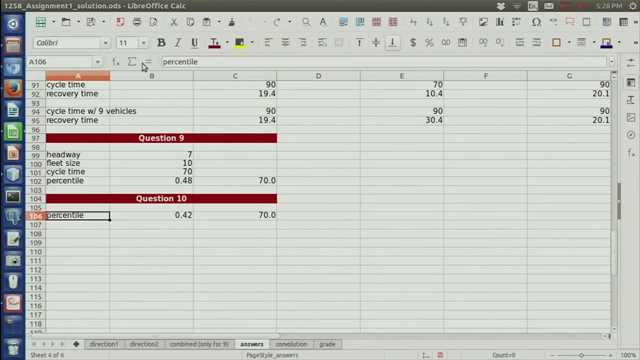 You reach B, You do recovery there And then you run back. So you have recovery here and here. And we're asking about times here. So we're saying what's the probability, with the same situation of seven minute headway and a fleet size of 10, that this trip? 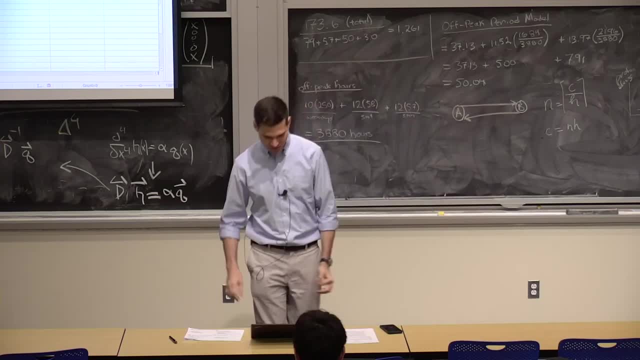 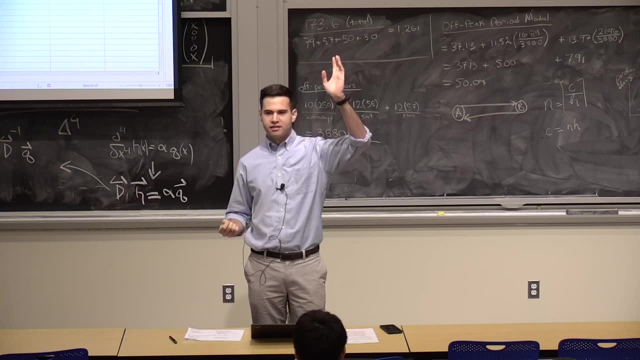 can depart on time, right. So for that there are different approaches for this. How many of you tried the question And how many of you think that they solved the question? Most of you, OK. Not with that answer, GABRIEL SANCHEZ- OK. 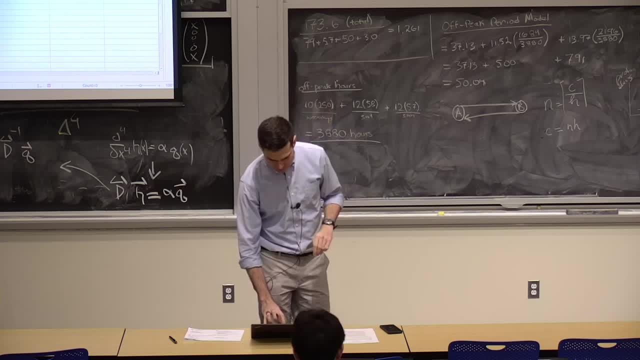 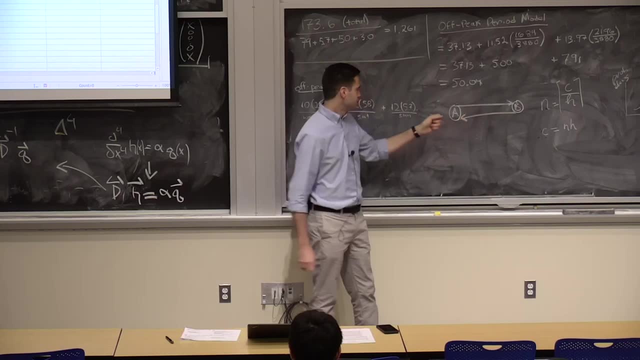 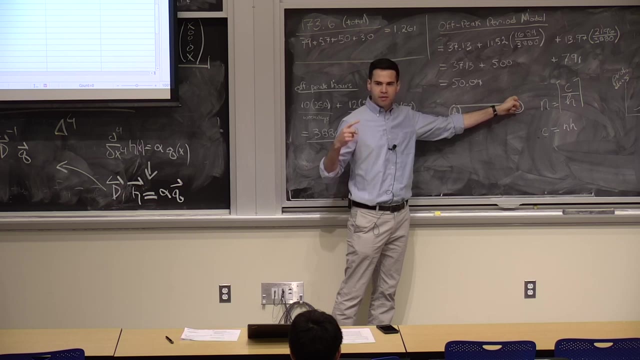 So it's actually not that difficult You can. essentially, what you have is a situation where you have different cases, right? Right, GABRIEL SANCHEZ-? So if you run here and you reach terminal B early, before your half cycle time is. 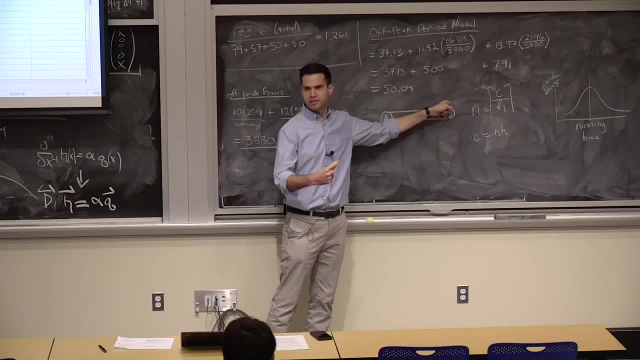 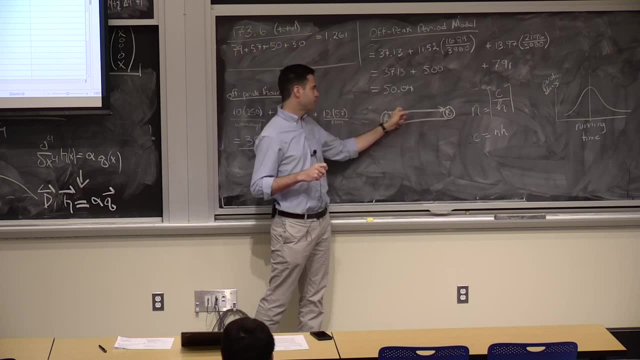 completed, then you will recover at B until you reach your half cycle time, right, And in that case the only thing that matters is the running time coming back. But there is a case where you run here and it's late and you depart immediately from B. So for those cases, 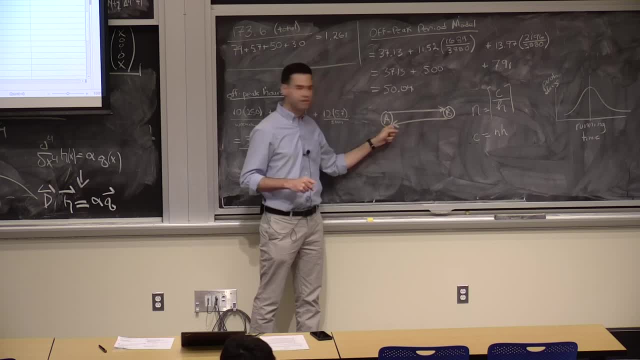 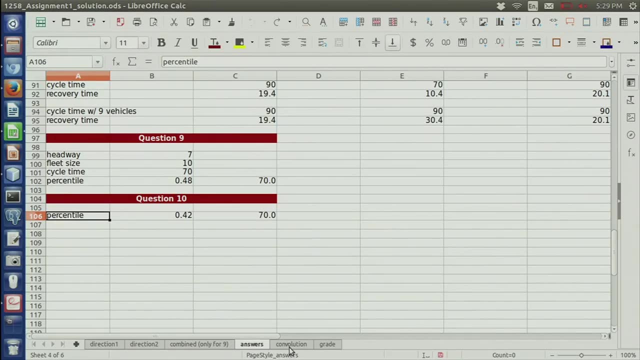 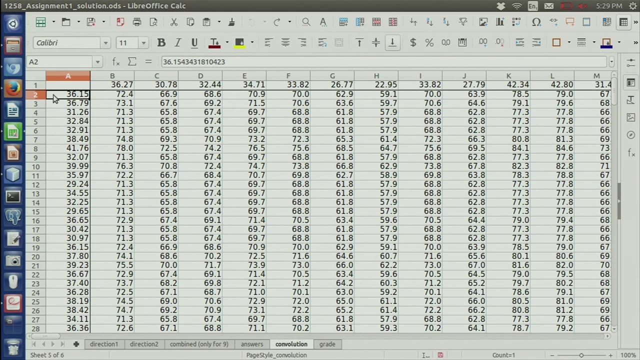 you have to compute the probability that the combination of running this way and that way is less than 70. So you have those two cases. One way of doing that is to take all the running times that apply, I think the set A and peak. 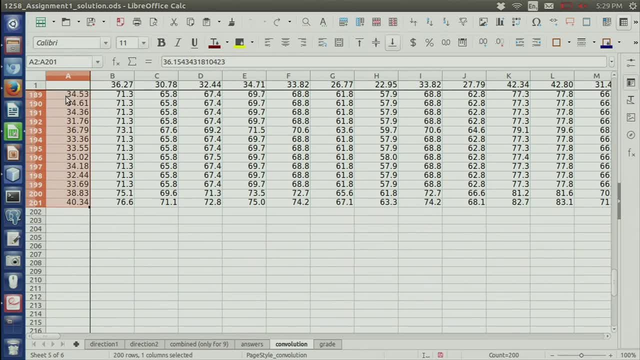 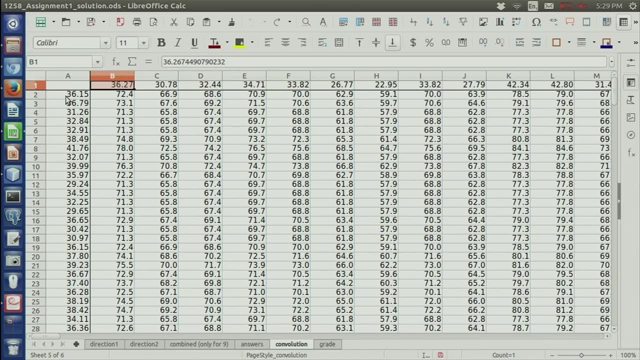 So direction 1 is on column A. There are 200 of these. Direction 2 is on row 1.. So I've done the transpose and put it on row, And then for each of these cells we can compute the combined running. 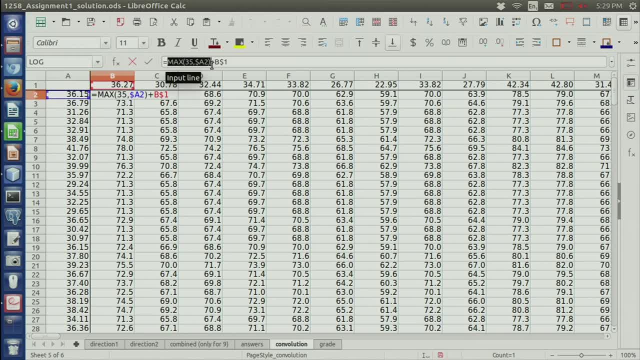 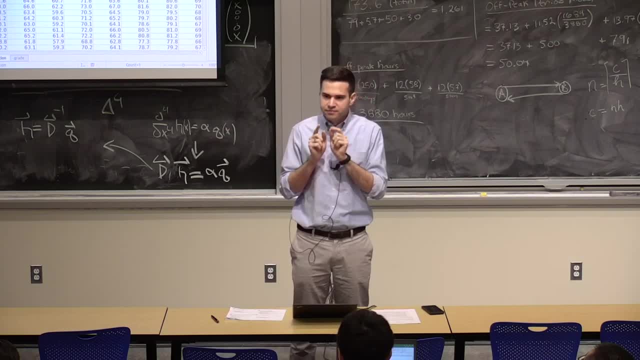 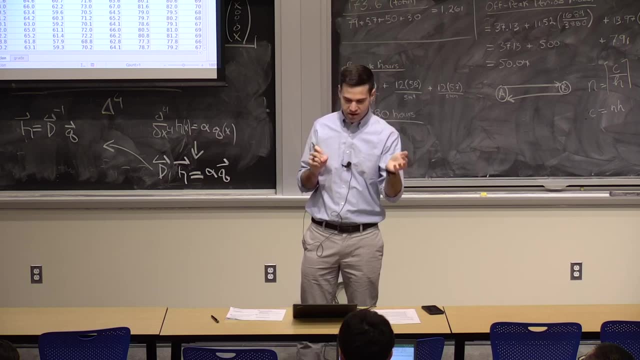 time. So notice that for the first one we're saying max of 35, which is the half cycle time. I decided here arbitrarily to split the whole cycle time of 70 minutes in half. So I'm saying the half cycle for the first run is 35 minutes. 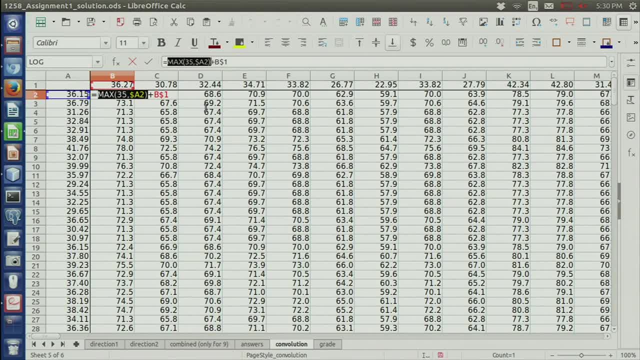 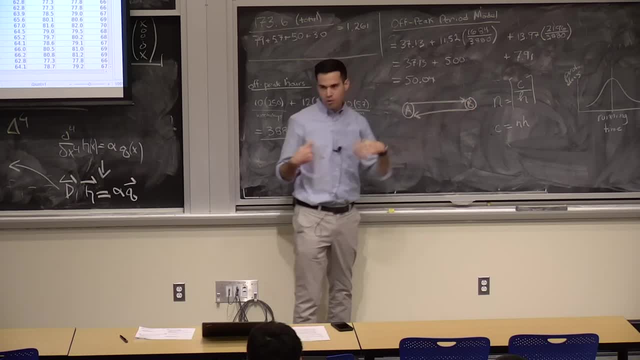 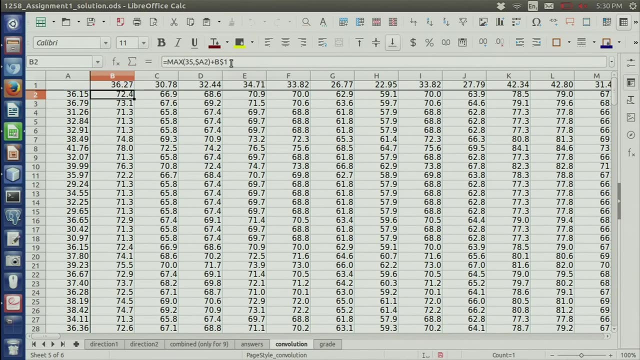 So the time of departure from B is going to be the maximum of 35 for cases where it was faster than 35. Or the running time if it was longer than 35. And then we add the running time in the return direction. So we combine these two distributions. 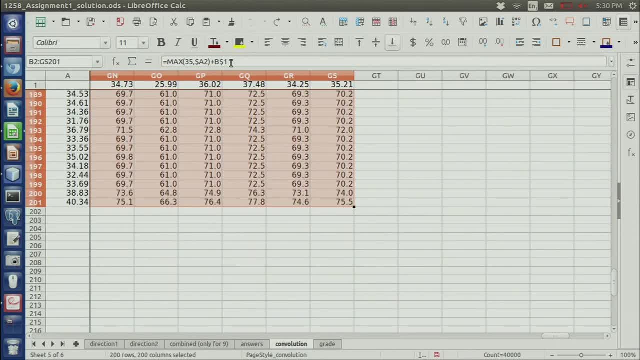 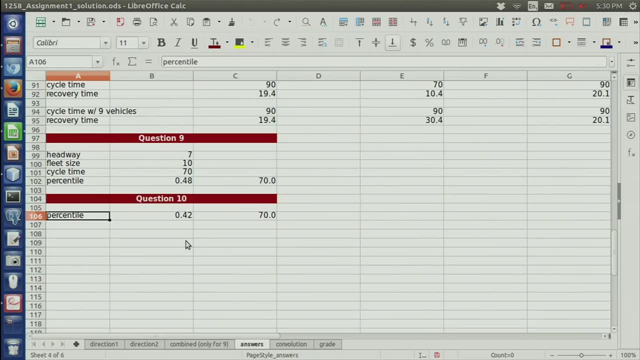 That's called the convolution. by adding all of these up, And all of these are possibilities, All the combinations of these observations are possibilities. And then we repeat the same thing. So we say: let's assume this is 50% And let's calculate the percentile. 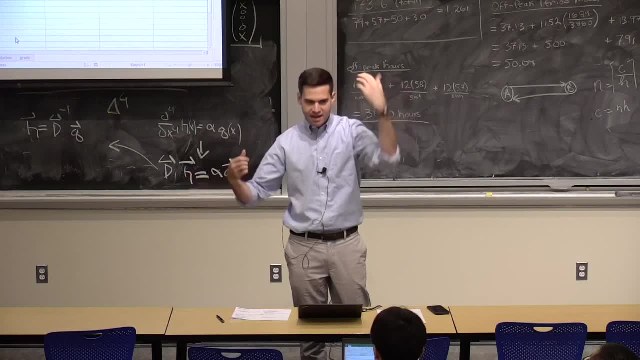 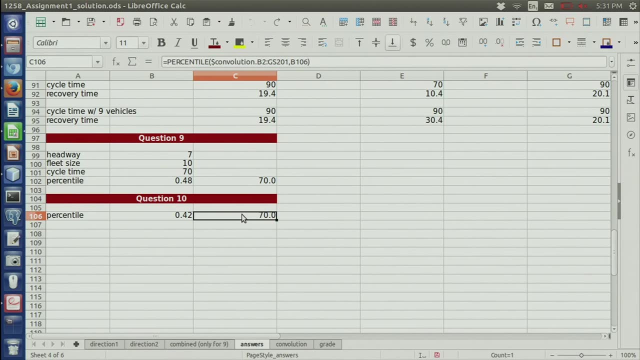 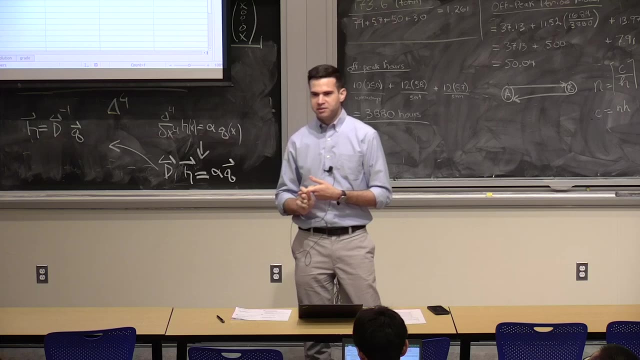 on all the cells in that matrix and ask the spreadsheet to provide or solve for the percentile that gives you 70. And the answer is 418, a little lower. Then there was an 11th question, which is very important. It's not a number question here. 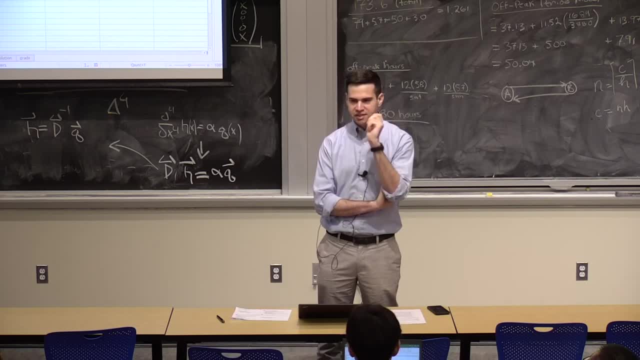 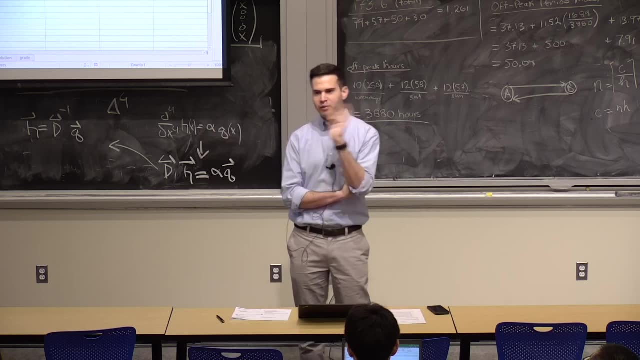 But it said there's this person who is watching these vehicles recover at the terminal And this person is annoyed that service is is not frequent enough And these drivers are wasting time. They're sitting there and not working. And that person proposes that you should run. 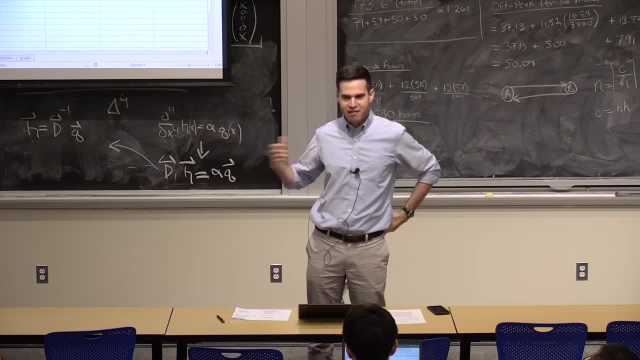 This person is an activist And they've gotten on the bus And they've measured the average time And they say: you can run this much faster, You don't have to wait, They're budgeting for so much time, So you should run this with average running times. 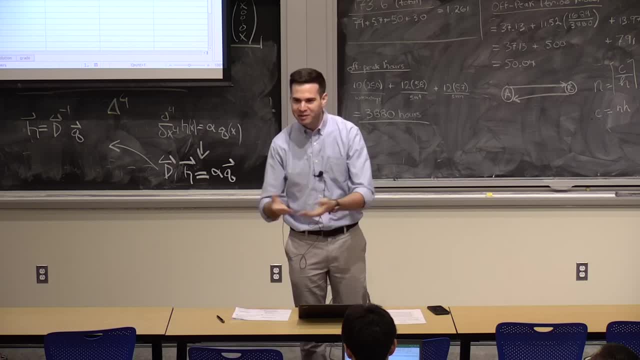 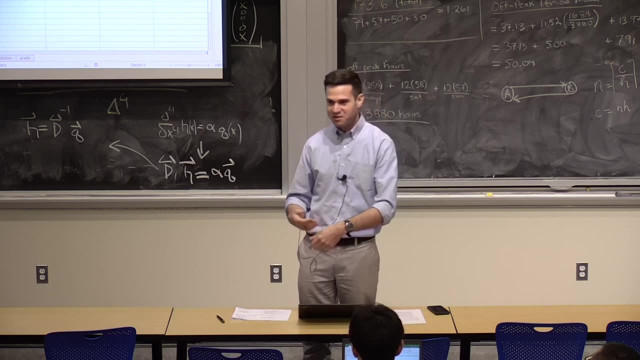 And it's your turn to sort of argue back. So hopefully you said that no, Recovery time is important. If you don't have recovery time, then many trips will start late And if you're trying to take your bus based on schedule, 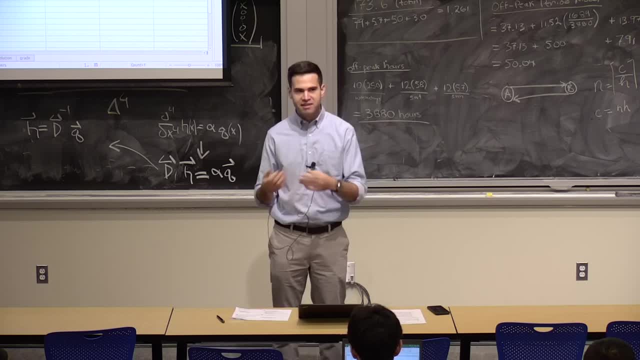 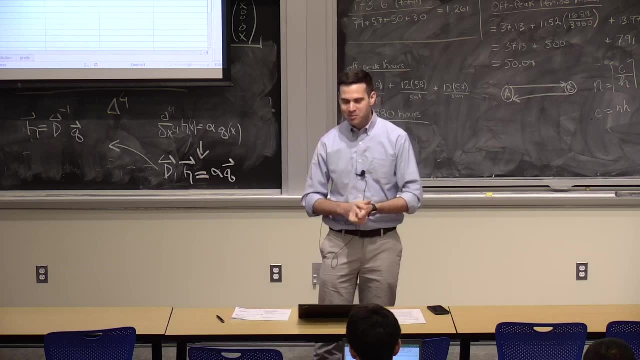 then it'll never be there on time And that would mean that you have to wait a lot longer And it will be very annoying for everyone. So that's it for assignment 1.. I hope you understood all of this And if you have questions, let me know. I will grade it and have it back to you as soon as possible. Thank you. 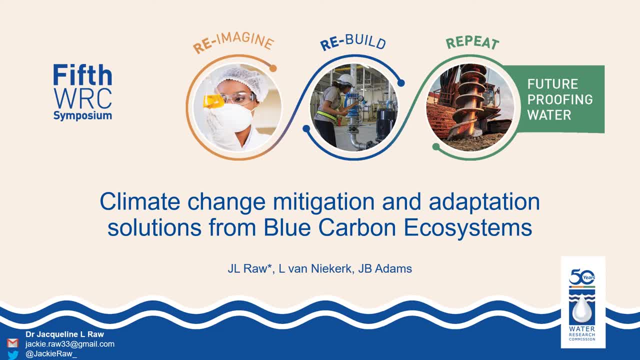 Good afternoon. my name is Dr Jackie Raw and I'm a postdoctoral researcher at the Nelson Mandela University. This afternoon, my presentation for the WRC Symposium is on climate change mitigation and adaptation solutions from blue carbon ecosystems. So what is blue carbon? 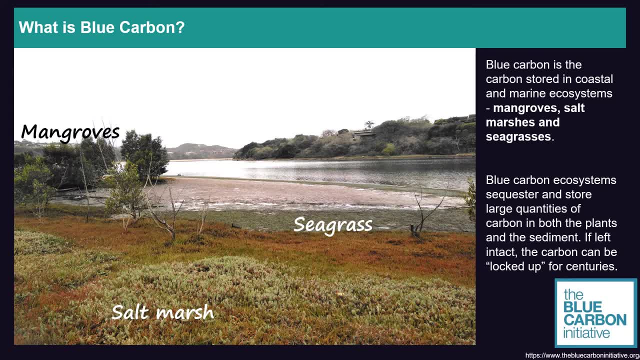 Blue carbon is the carbon that is stored in coastal and marine ecosystems, specifically within mangroves, salt marshes and seagrasses. These ecosystems sequester and store large quantities of carbon dioxide from the atmosphere, which is then locked into the plants and the sediment. 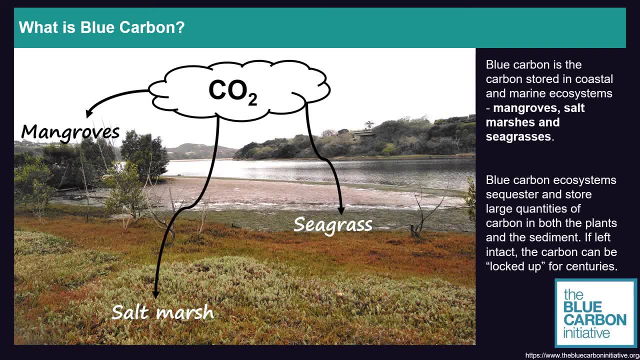 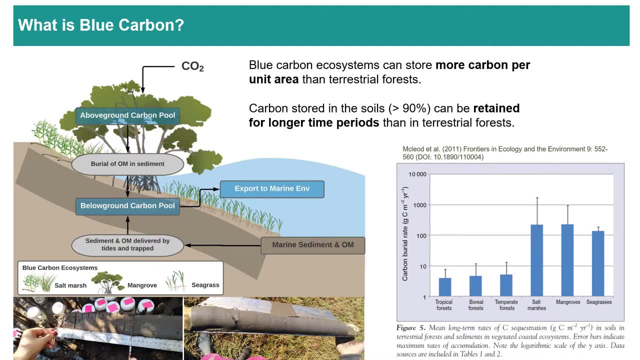 If this is left intact, the carbon can be locked up in this way for centuries. Blue carbon ecosystems can store more carbon per unit area than terrestrial forests. This is because up to 90% of the carbon stored in these ecosystems is within the soil, and this can be retained for much longer time periods than in terrestrial forests. 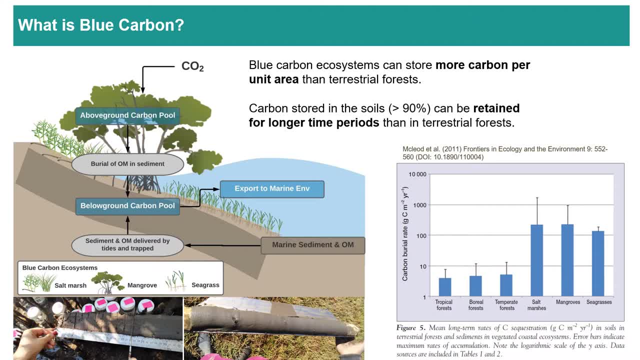 If we take a look at the lower left-hand side, we can see the organic rich soil deposits that are extracted from these ecosystems. On the lower right-hand side, we see the carbon that is stored in these ecosystems. If we take a look at the lower left-hand side, we can see the organic rich soil deposits that are extracted from these ecosystems.